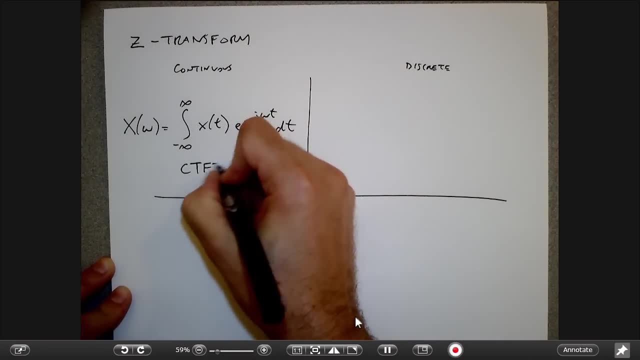 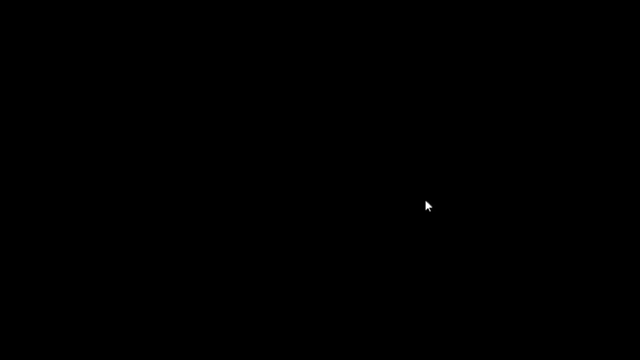 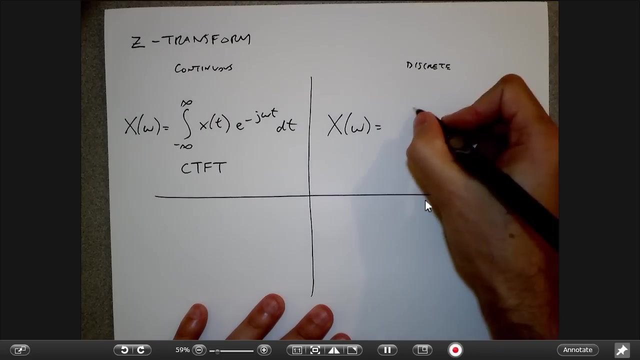 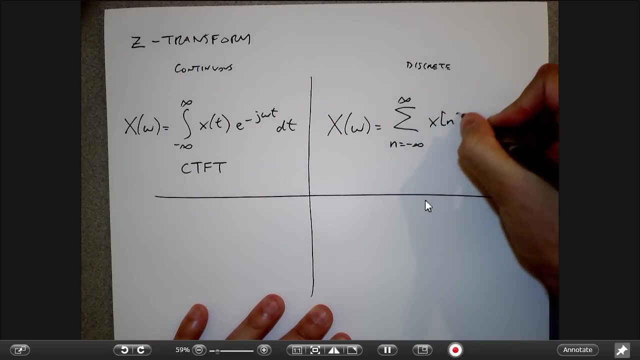 And so I would call this the continuous time Fourier transform. In the discrete world we have the discrete time Fourier transform, Which is, instead of an integral, it's a sum. So since I have a discrete set of x values, that means I turn this infinite integral into an infinite sum and it looks kind of similar. otherwise, right. 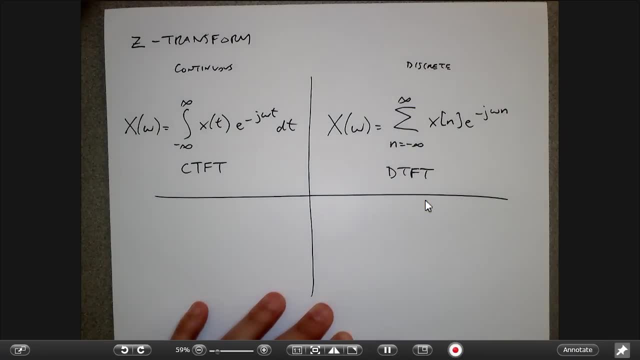 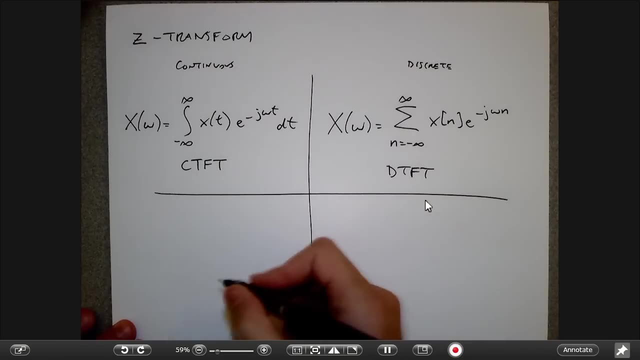 We defined this as the discrete time. Fourier, transform. Now, when you were taking single systems and differential equations, you also saw the Laplace transform, right. So the Laplace transform, which I'm not going to talk about really at all in this class, I'm just putting this down here as a reminder of what you hopefully remember. 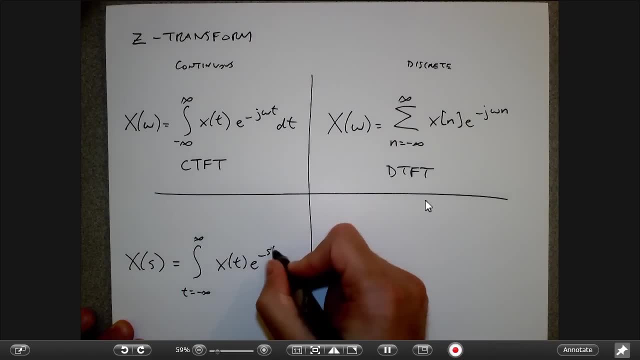 The Laplace transform was kind of like a generalization of the Fourier transform right. What I was doing was I was replacing j omega with this more generic, complex variable s right. And so the reason that we cared about the Laplace transform was it allowed us to solve problems that we couldn't solve with the Fourier transform alone, right. 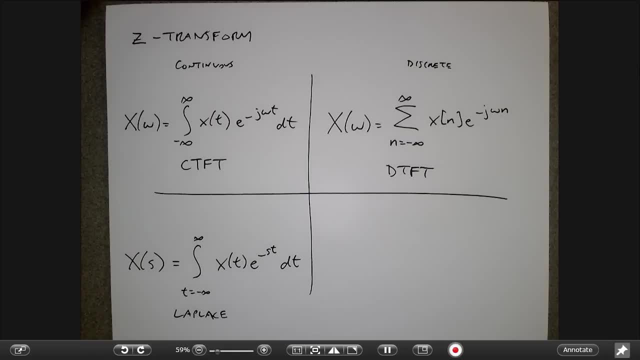 And so in some sense, you know, once you know the Laplace transform, you can solve a lot of things in the Laplace domain without actually having to go back to the Fourier transform. The advantage of the Fourier transform is that it has this very intuitive and concrete interpretation of its frequency. 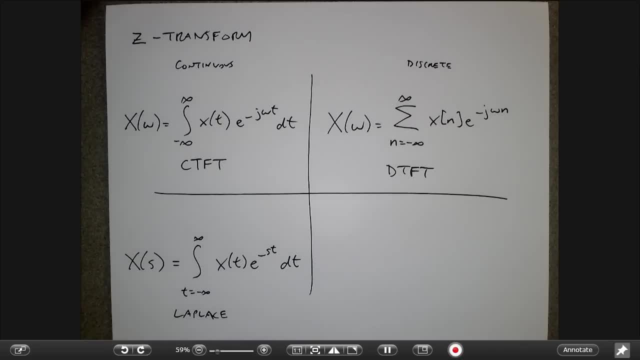 We know a lot of real-world electrical engineering systems involve frequency, and so that's why you know we kind of need them both, can't need them both, And so the question today is: what is the discrete time version of the Laplace transform, and that's what's called the Z transform. And again the idea. 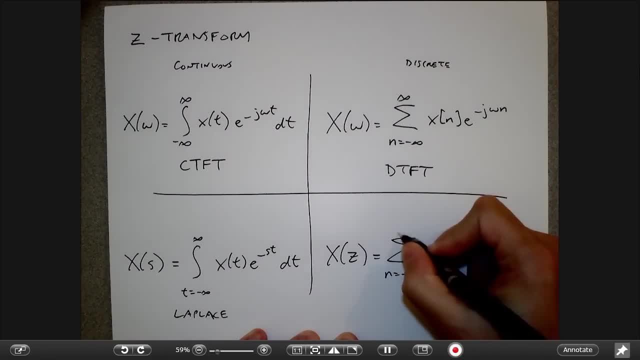 is the same. I turn this infinite integral into an infinite sum and I replace the e of the j omega n with a z to the minus n, And so again, this is a more generic idea- where before my omega was only a kind of real-valued frequency variable, Now z is. 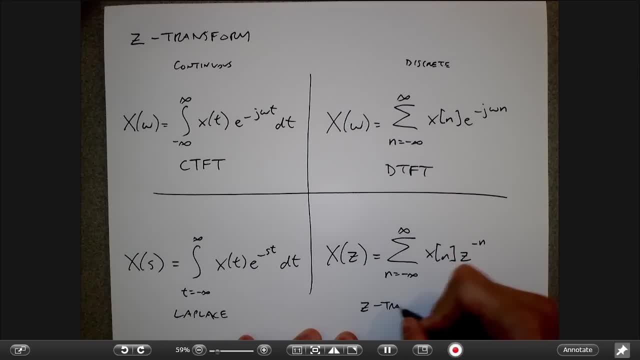 some complex number, And so let's pause and ask: so why does this make sense as a thing that we want to do to a signal? And so, again, one of the things that we showed- for both the continuous and discrete time Fourier transforms- was 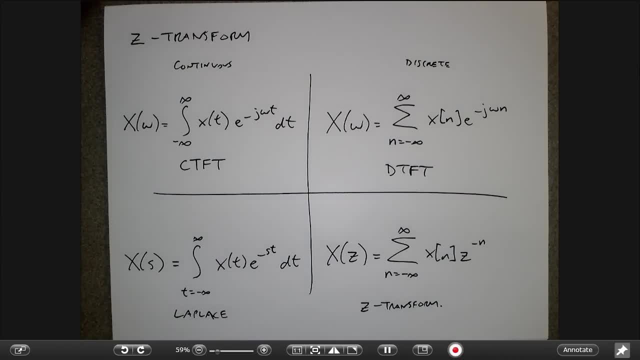 What I showed was that these exponentials e to the somethings were kind of important for LTI systems in the sense that when e to the something went in, the same e to the something came out, just modulated by this frequency response, And so the same thing. 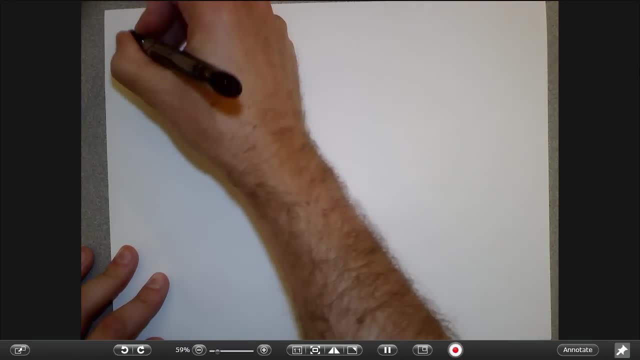 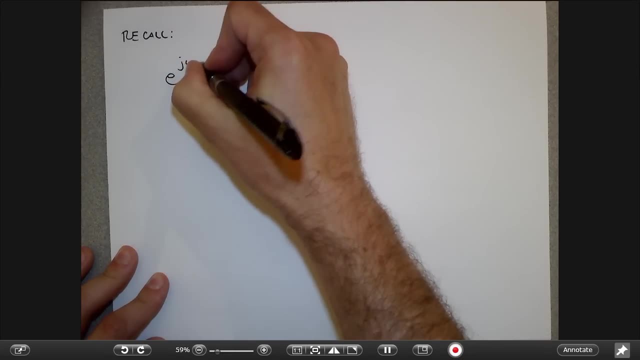 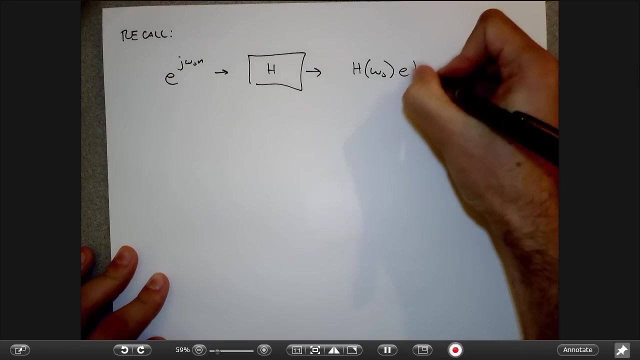 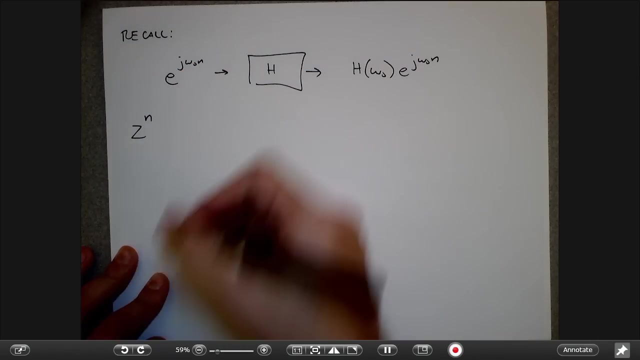 is actually true for z's. So kind of remember that if I had something like e to the j, omega zero, n and I put that into the system, what came out was basically the same thing. So that is basically the frequency response, like so, So in the same way, z to the n. more generically, 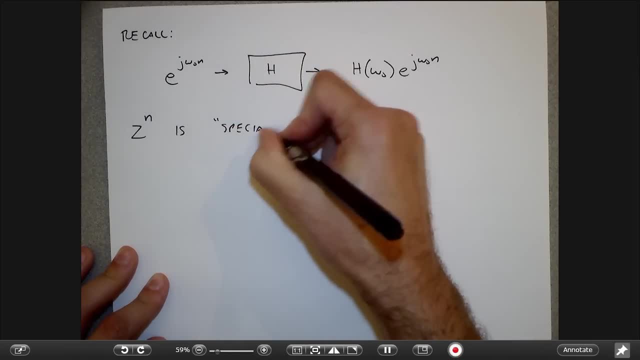 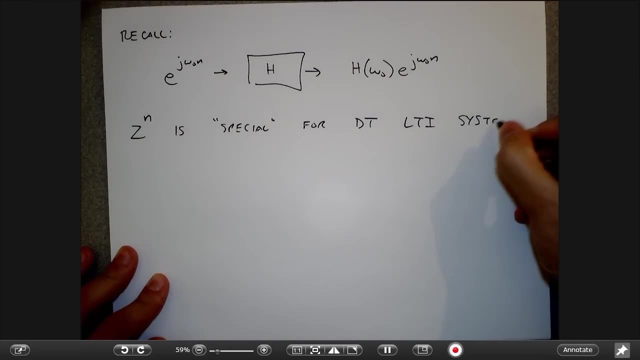 is special for discrete time LTI systems. What do I mean by that? Well, let's suppose that my input signal is this: z to the n. So I usually try to put a little bar through the z if I forget. Keep in mind this is a z. 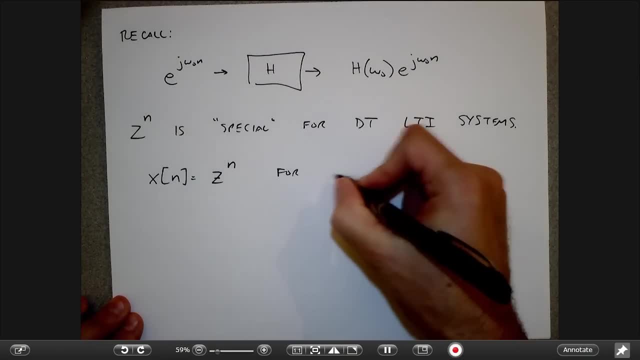 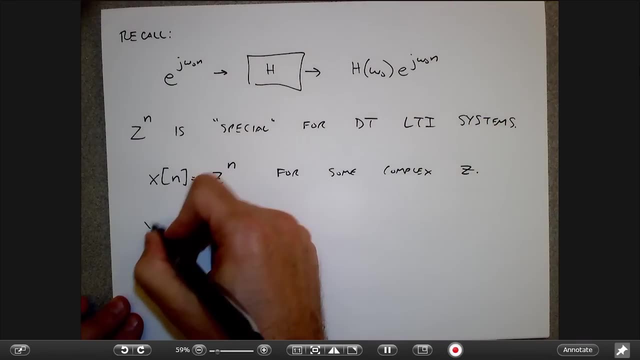 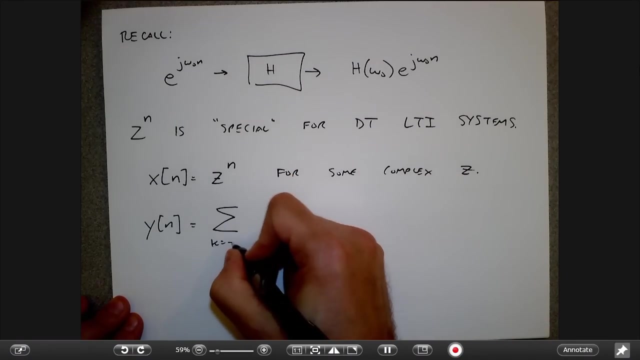 and not a 2.. So this is going to be z to the n for some complex z. So what is the output if I put that signal through an LTI system? Well, it is going to be my usual convolution between whatever my impulse response is and whatever my signal is, And so that's going. 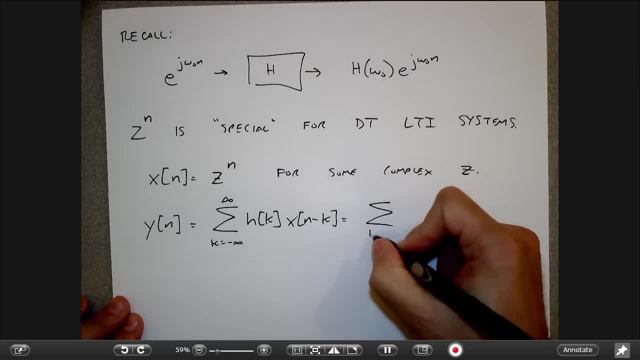 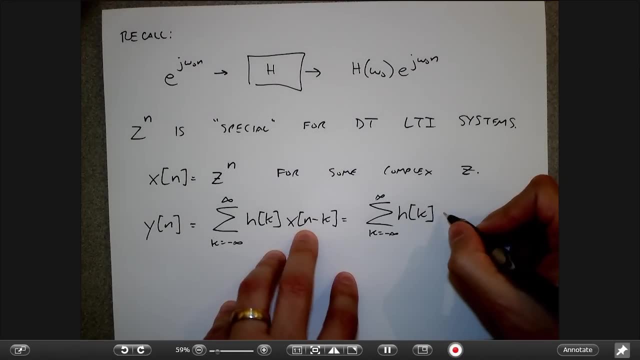 to be my usual convolution between whatever my impulse response is and whatever my signal is, And I'm going to plug in what I know here. I have the impulse response and I have x to the n minus x of n minus k is the same as z to the n minus k, Since this sum is over. 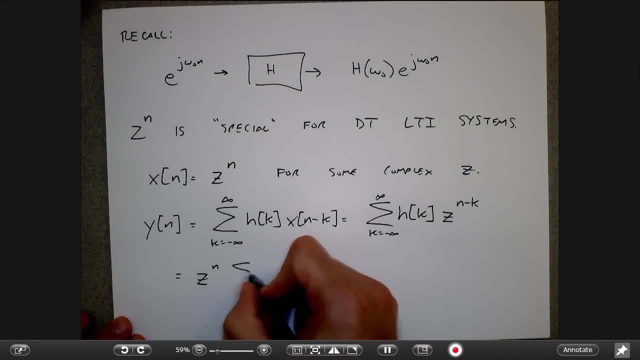 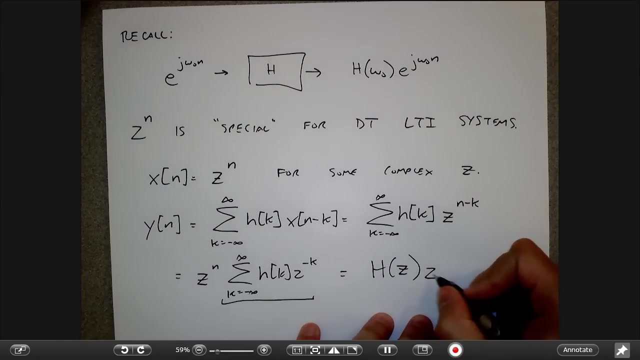 k, I can take the z out and I have just this sum, And this, in fact, is the z transform of the impulse response. So, basically, this is what we call the z transform of the impulse response. This is called the transfer function, And what we showed is that if this complex 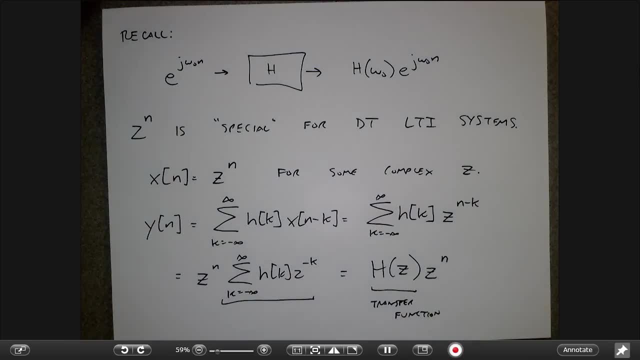 exponential comes into the system, what comes out is the very same complex exponential just multiplied by again this transfer function evaluated by complex number z. And so this is what we've just kind of shown here- is that this notion of special signal comes in. 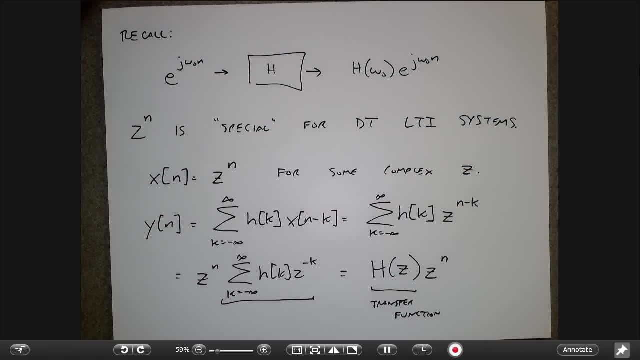 exactly the same, as special signal comes out, just modulated by some complex number. that's exactly true. So what we kind of showed before was this was true for some specific set of complex numbers, that is, the ones that are on the unit circle e to the j, omega something. 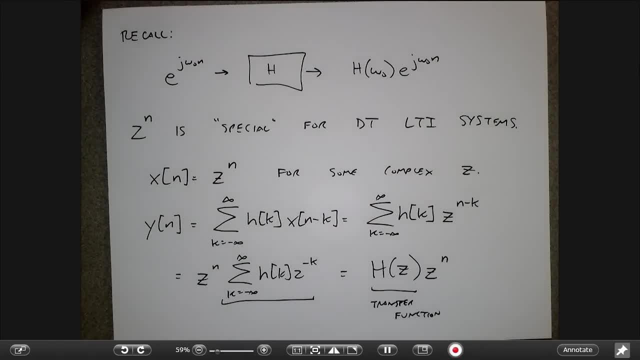 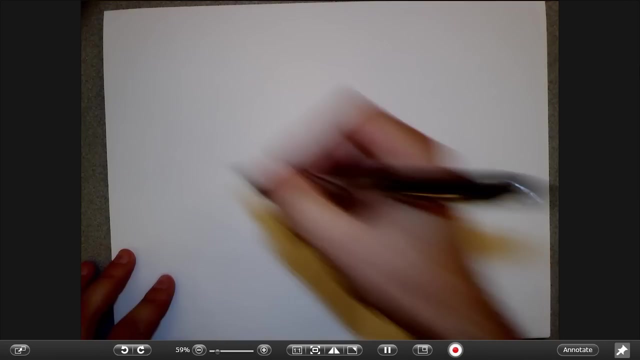 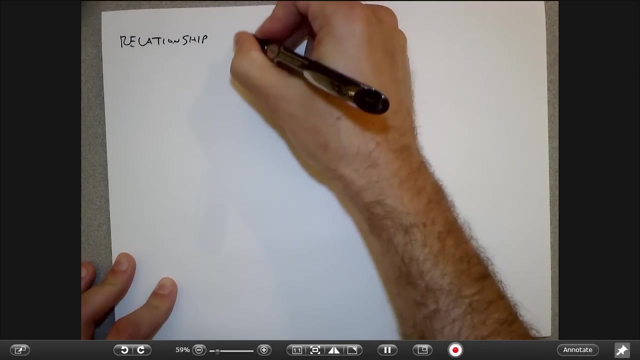 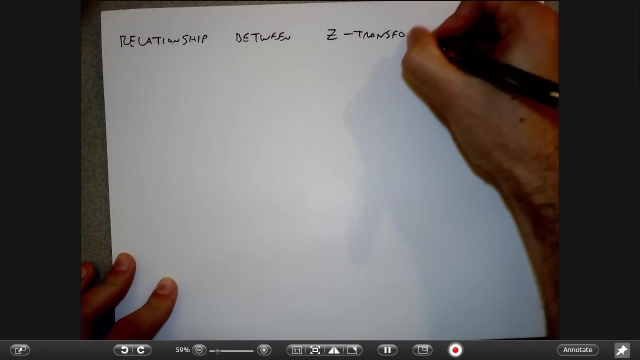 But here this is actually true for any complex number, And that's why we can talk about more generic transformations than just the frequency response. So just as a refresher, so let's look at the relationship between the z transform and the DTFT. 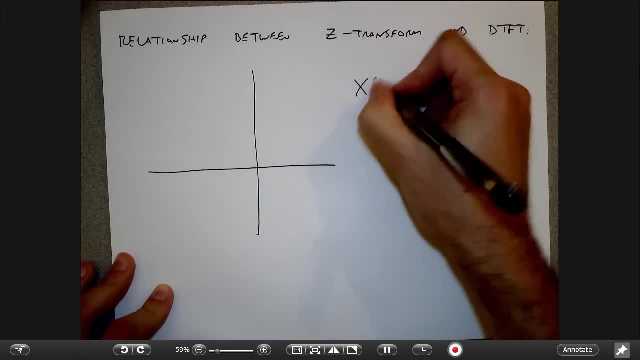 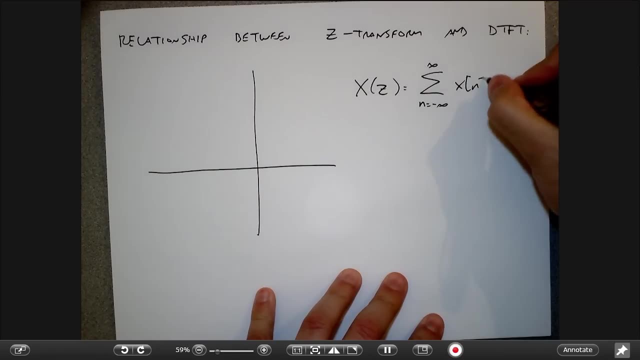 So the z transform is the following. So the z transform is the following. So the z transform is the following: It's this sum x of n z to the minus n. It's this sum x of n z to the minus n. 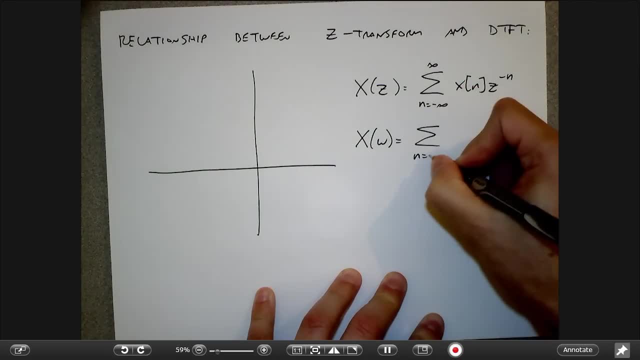 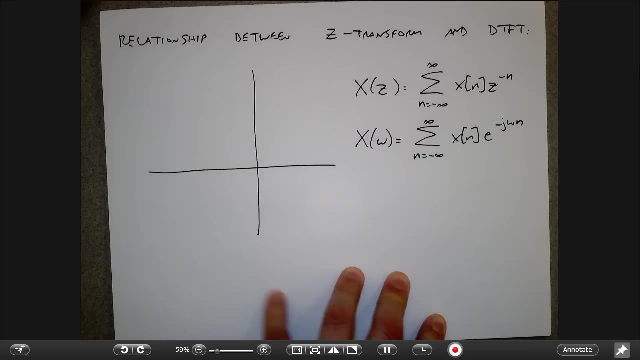 And the DTFT is this: sum x of n- e to the minus j, omega n, And I can see that these formulas look pretty similar. In fact, this is exactly what I would get if I took x- of z and I evaluated it at the 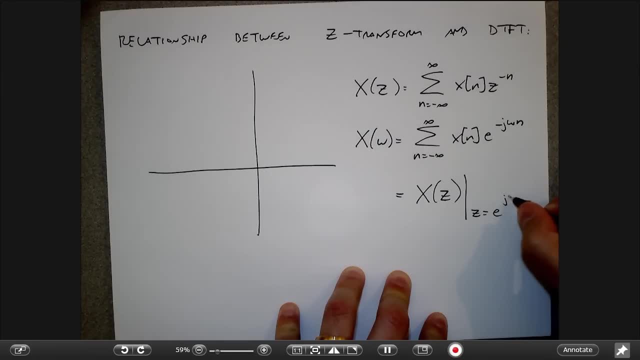 points, z equals e to the j omega Right. What that means is that that's like saying that if the Fourier transform, the DTFT, exists. what it is is the places where z, the complex number z, is e to the j omega over some omega. 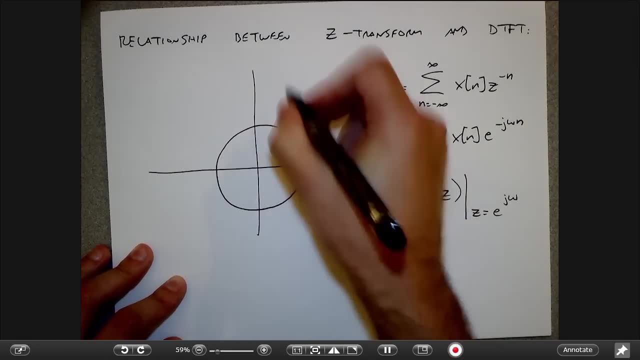 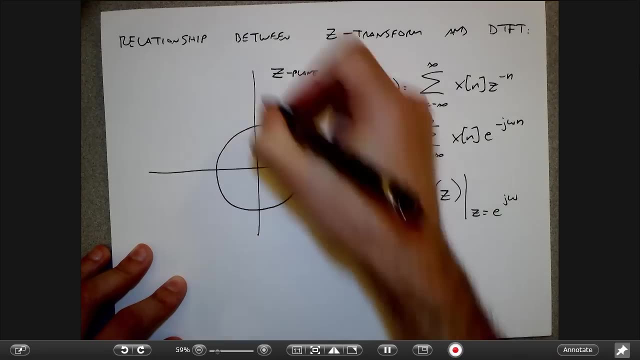 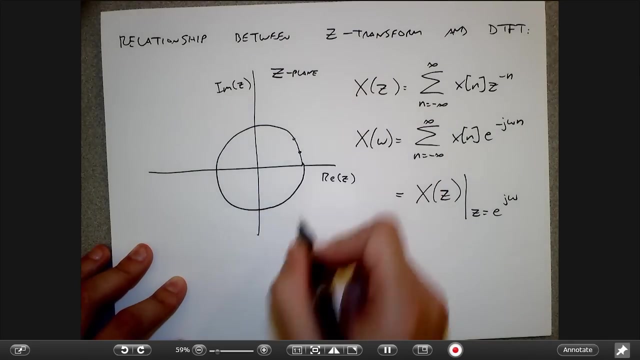 And so that means that in my z plane, if this is the real part of z and this is the imaginary part of z, I'm going to have a z. The Fourier transform is exactly those places where that complex number happens to be on this unit circle. 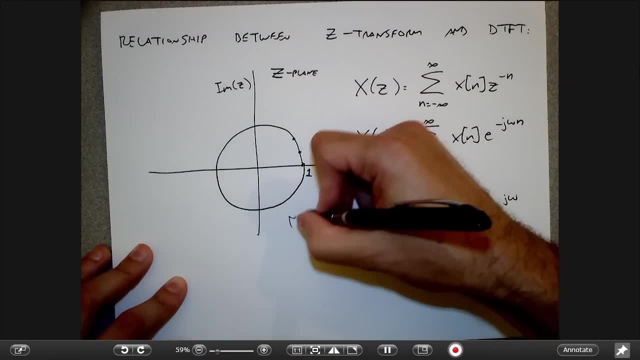 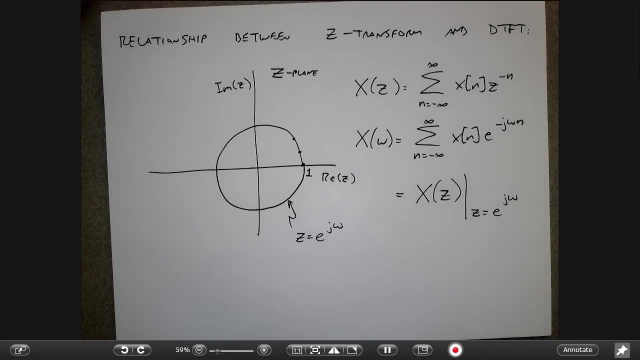 Right. So this sketch is: z equals e to the j omega, And so kind of what we're saying here is that when the Fourier transform exists- and I'm going to talk about this concept in more detail in this lecture, because one thing that you 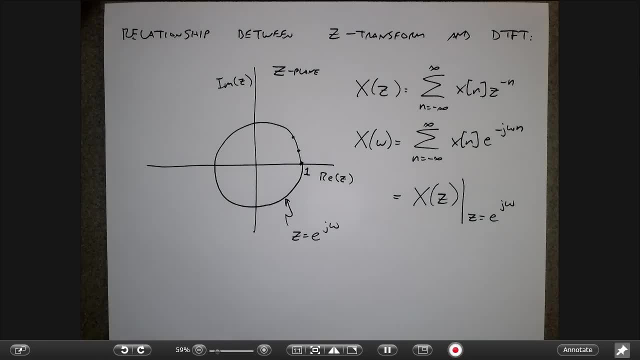 should remember about the z transform that may be familiar from your class, is that the z transform has what's called a region of convergence Right, This formula, this function x of z isn't automatically defined for any z that you choose. It's only certain z's that make this formula converge. 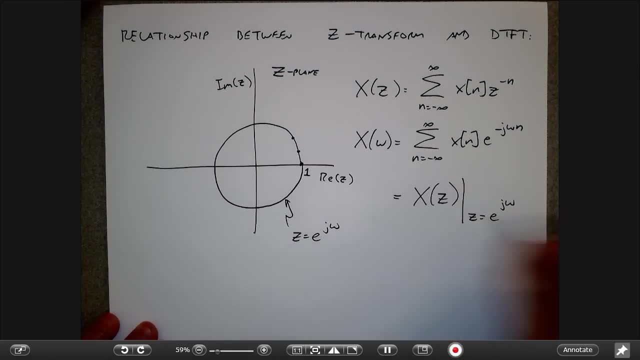 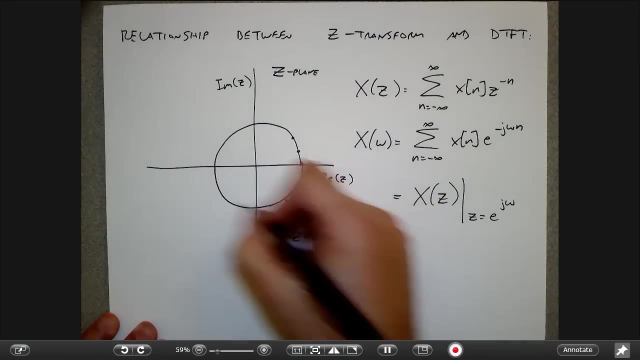 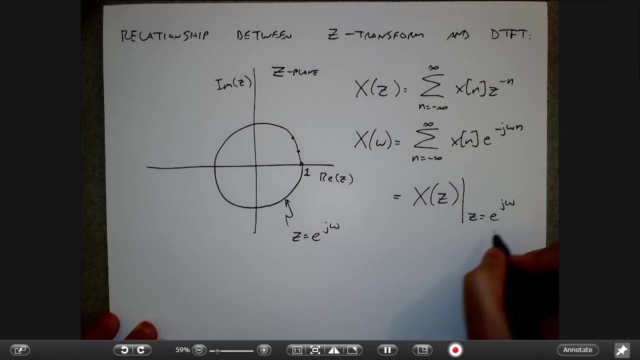 And so when the z transform and the Fourier transform both exist on the end circle, then they, then they're related by this thing, And so this actually makes it kind of clear that, since I'm evaluating omegas as they go from zero to pi, this kind of makes it clear that the DTFT has to do something. 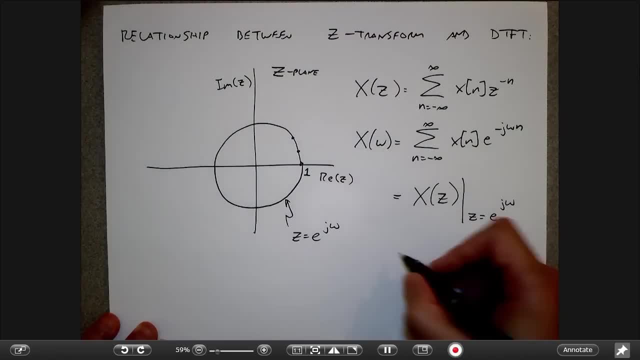 It has to be periodic because I have this circular relationship. So this again as a reminder: the DTFT is 2 pi periodic, So I'm not going to talk about Laplace too much, other than to say that just in the same. 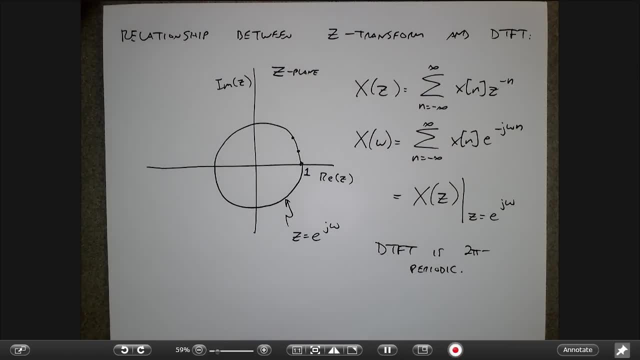 way that the j omega axis, the imaginary axis, played a big role in analyzing continuous time systems, the unit circle plays a big role in analyzing discrete time systems. Okay, So, So let's say unit circle is key for discrete time systems, like the j omega axis was for. 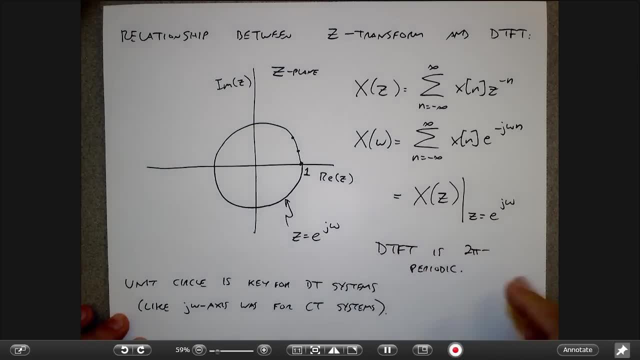 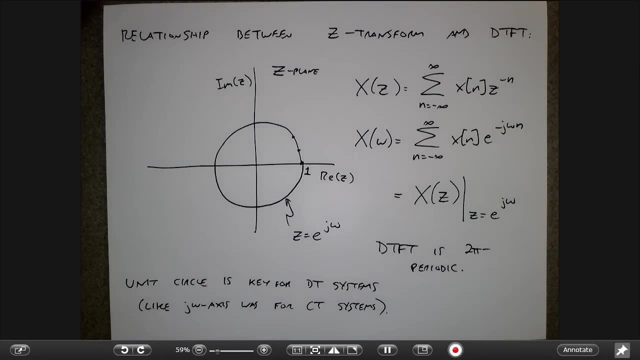 continuous time systems, Right, So if you're doing a continuous time class you spend a lot of time worrying about. you know when did poles, for example, cross over the j omega axis? That affected the system's stability, and so on. 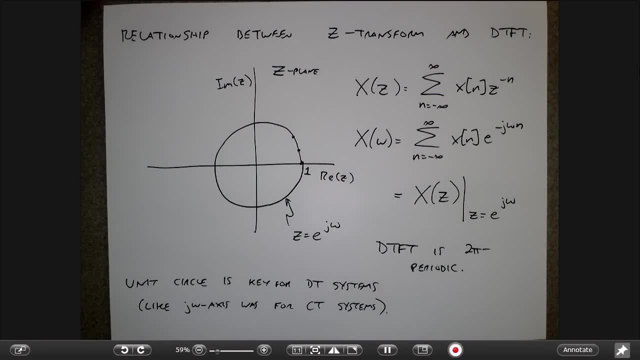 We're going to talk about exactly the same concepts here, except now we care about when do poles stay inside the unit circle, Right? So there's kind of a symmetry here, There's kind of a relationship here. Okay, So Okay. 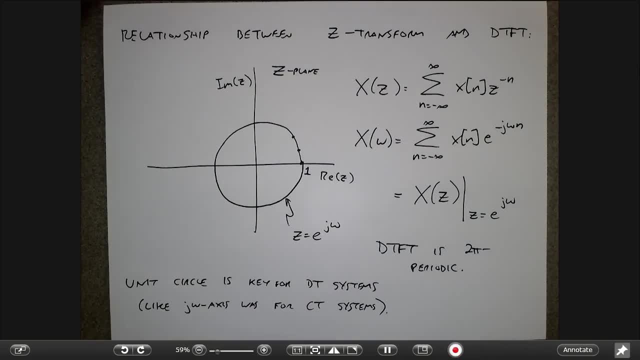 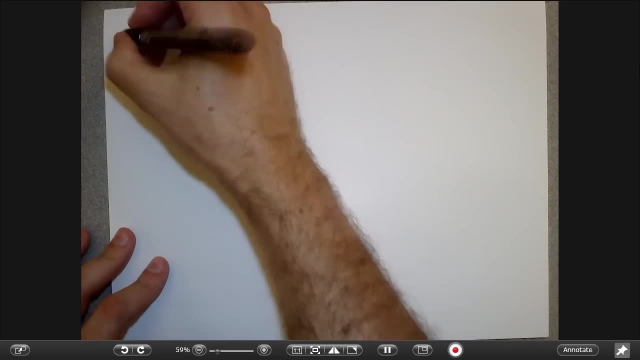 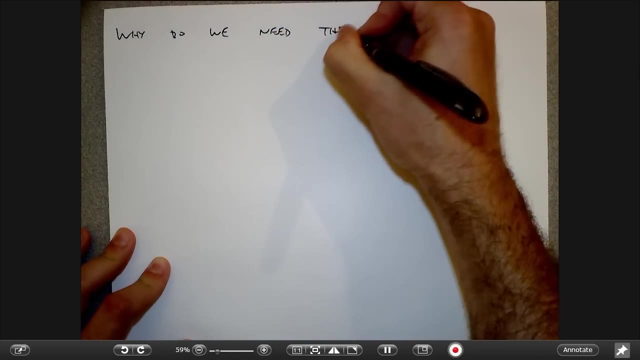 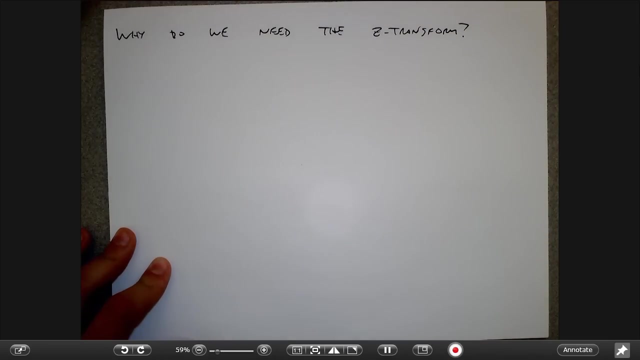 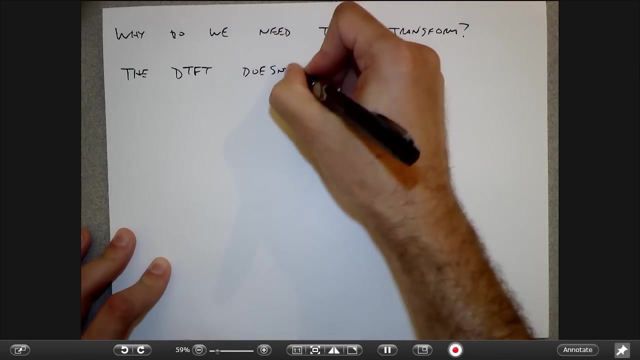 So I'm going to pause and ask for a second. Does that make sense? Any questions? Okay, So why do we need this Z-transform? So why do we need the Z-transform? Well, one reason is that the DTFT doesn't always converge or exist. 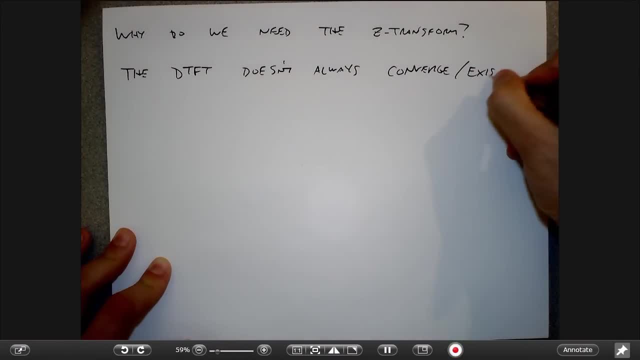 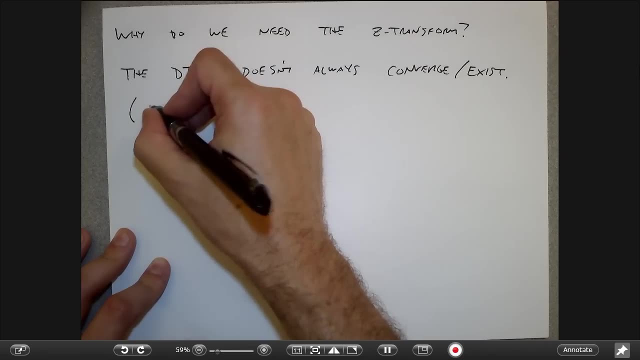 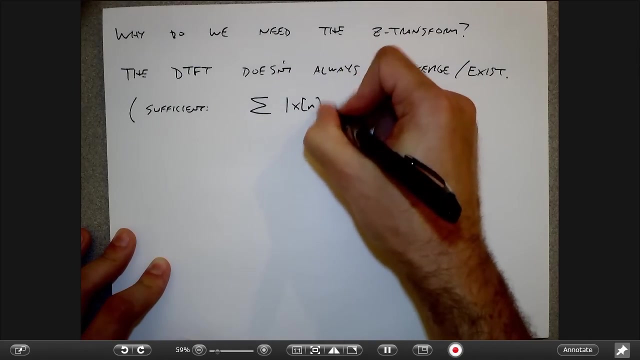 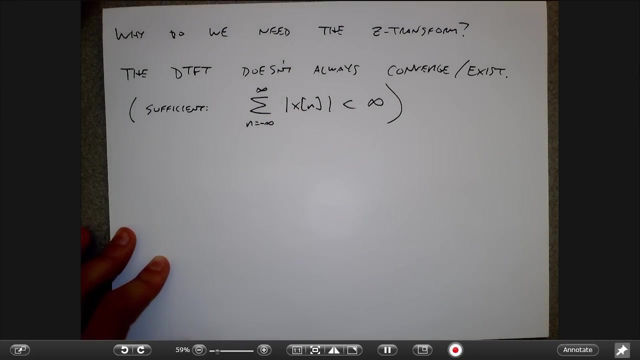 Right. So we showed last time that kind of a sufficient condition was that if I were to sum up these things, I would get some non-infinity number Right. That's like saying that you know, I need to be able to sum up the absolute and the. 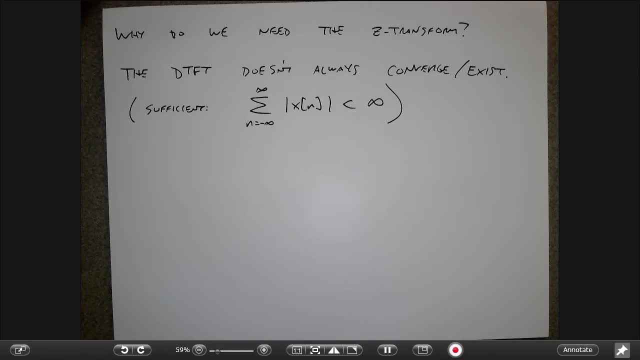 some of the absolute values of the signal for that sum to converge right, And we talked about how we could relax this slightly, but for the moment let's just assume this is the condition that we need for the DTFT to exist in the way that we want it to. 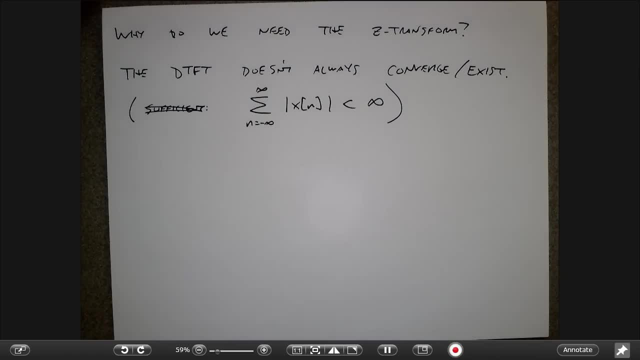 By that I mean I want to make sure that as I take incremental approximations to the DTFT given by you know, increasing n from you know 0 out to infinity, that I want to make sure that my DTFT converges at every point of the signal. 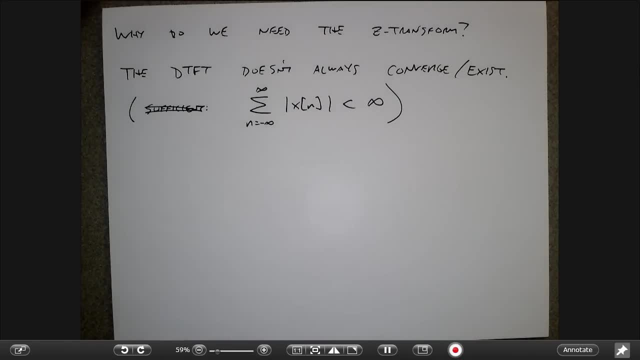 to the actual Fourier transform value, right, I want to avoid these Gibbs phenomenon kinds of issues, right? And so not every signal satisfies this constraint, right. And so if we're staying in Fourier transform world, we kind of have to throw up our hands at this point and say: 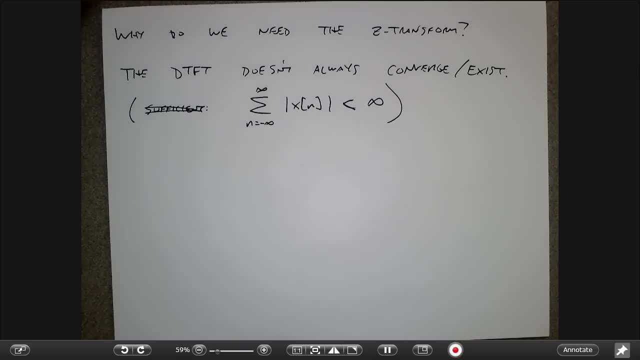 well, there is some signals that I can't analyze with the Fourier transform. right, Because the Fourier transform doesn't exist. The Z-transform allows us to talk about a more general class of signals. okay, And so some points to remember, are you know? 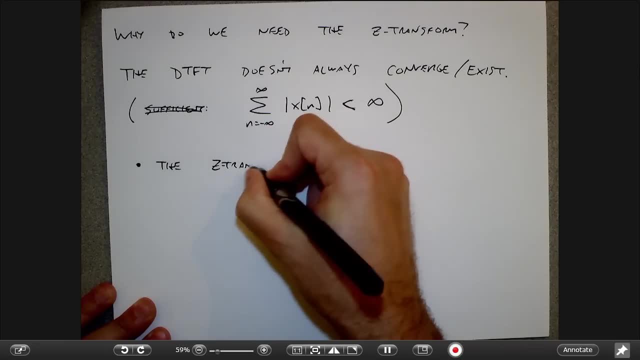 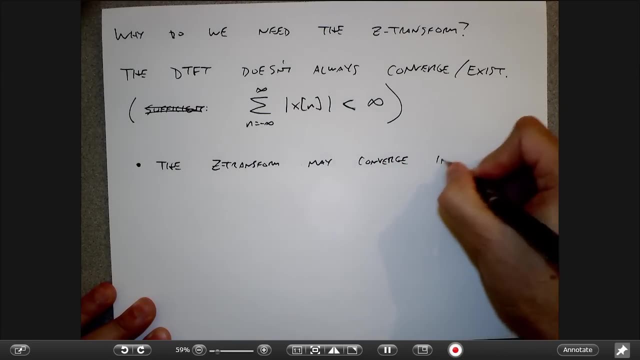 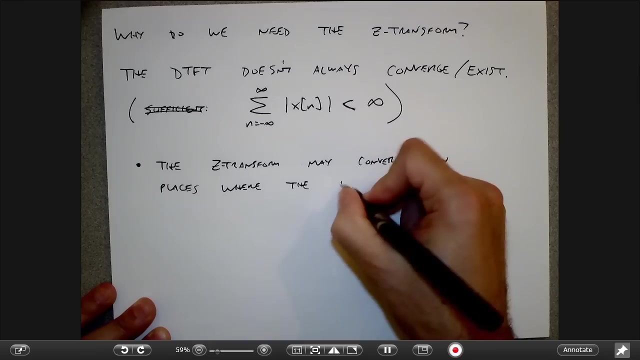 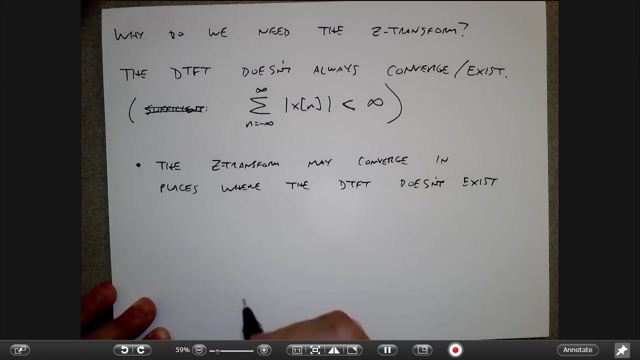 the Z-transform may converge in places where the Fourier transform doesn't exist. So that's one important reason. One other reason, which is not really the best reason in the world, but it's good to keep in mind, is that the notation is generally easier right. 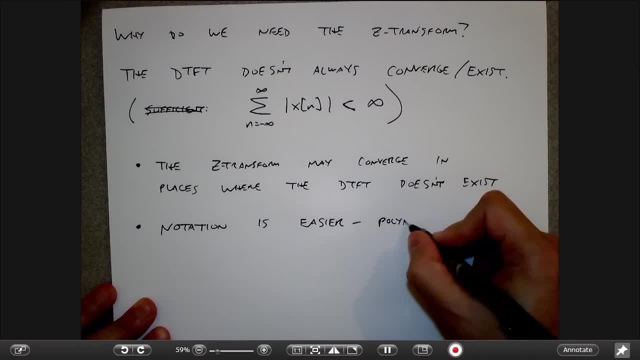 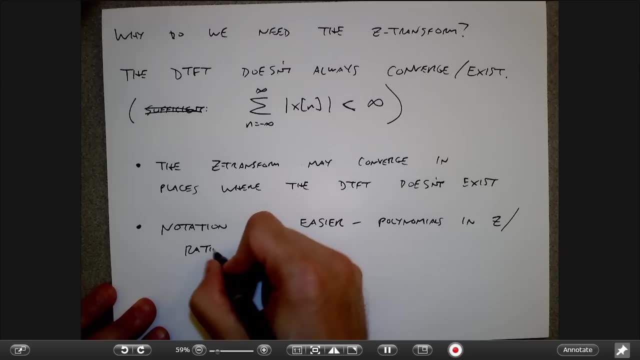 So you know we get a lot of polynomials in Z Or we get rational functions of Z. So in general, you know, you kind of lose all these e to the j omega things that were a little bit kind of tedious to kind of keep in mind. 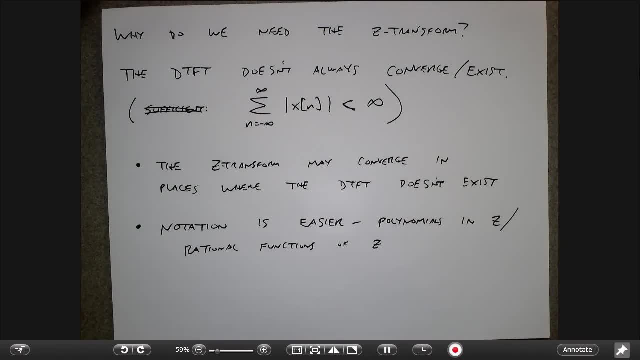 And you know, like when you were doing the homework on the DTFT, right, You see, you have to keep track of all these e to the j, omegas- It's kind of a pain right- Whereas Zs are much cleaner, just like manipulating polynomials. 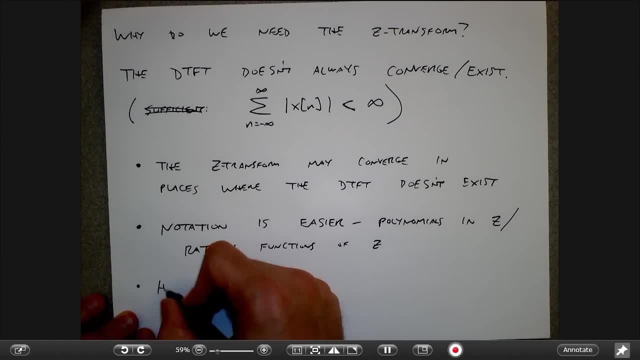 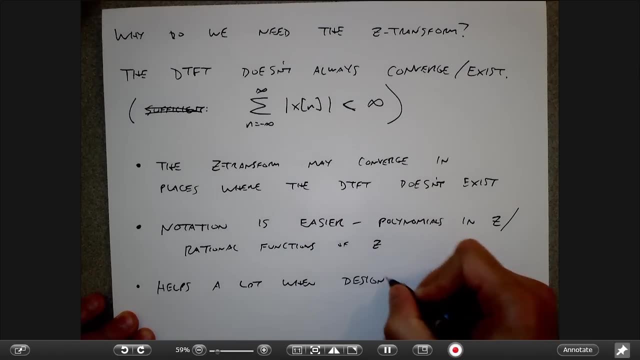 And the third one is that the Z-transform helps a lot when designing filters, And we're going to talk more about that after the first exam. But the idea is that, you know, I look at what are called the poles and the zeros of the Z-transform. 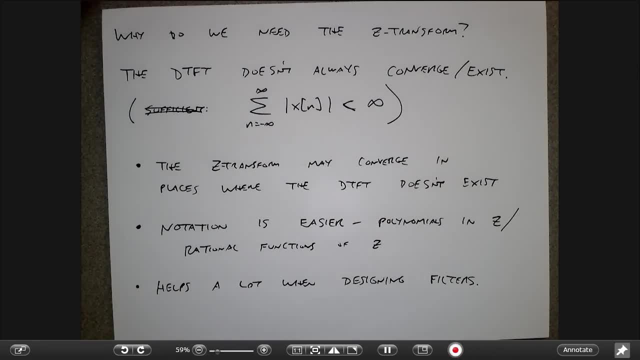 Understanding what those poles and zeros are doing helps me extremely in terms of designing filters that do what I want to do right. It's tough to design filters directly in the frequency domain, but it's a lot easier to do it in the Z world okay. 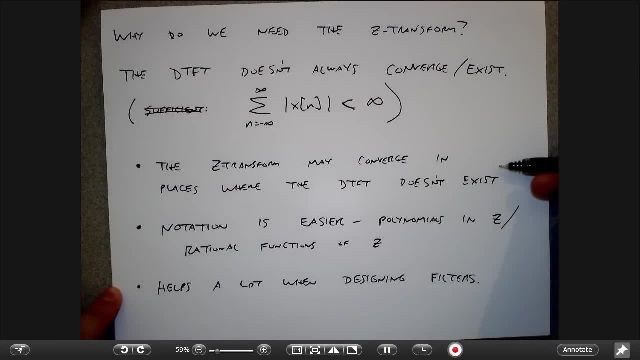 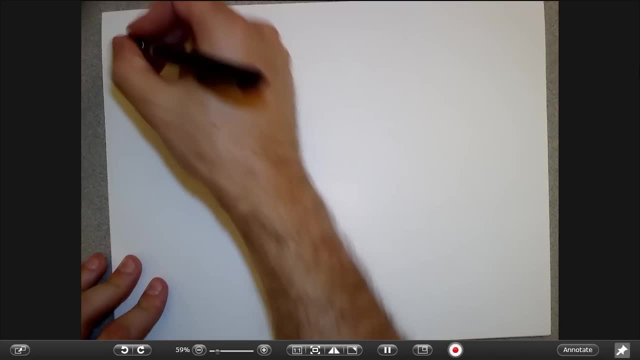 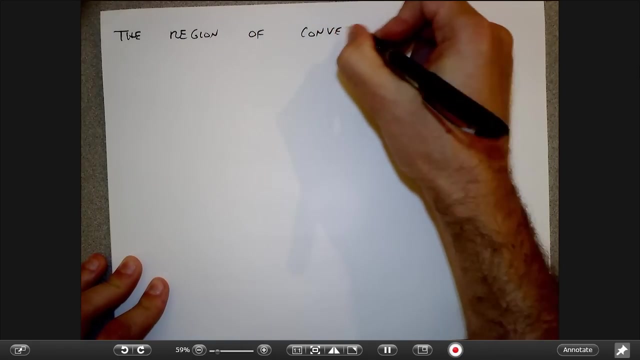 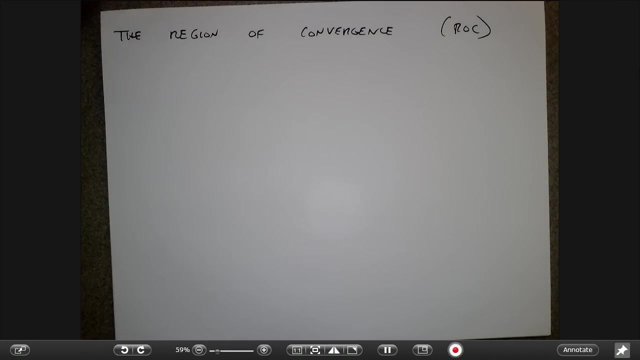 So let me drill down a little bit into this first point about when the Z-transform converges, Okay, And the critical concept here is called the region of convergence, Which we sometimes call the ROC, Okay, So again, this all kind of follows way back when from sums and series in calculus, okay. 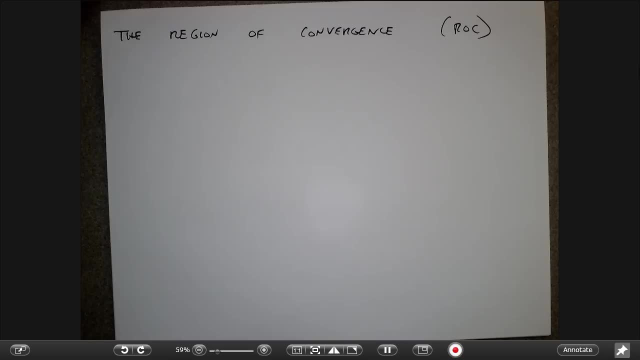 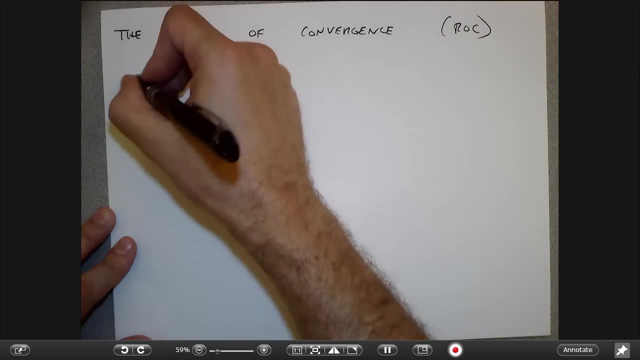 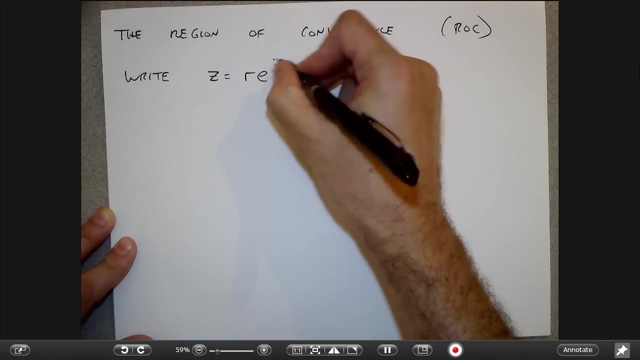 So I'm not really telling you anything that you couldn't have done in theory in like high school almost, or first semester of your freshman year. So here's the idea. Let's write Z in polar form, Some magnitude e to the j theta. 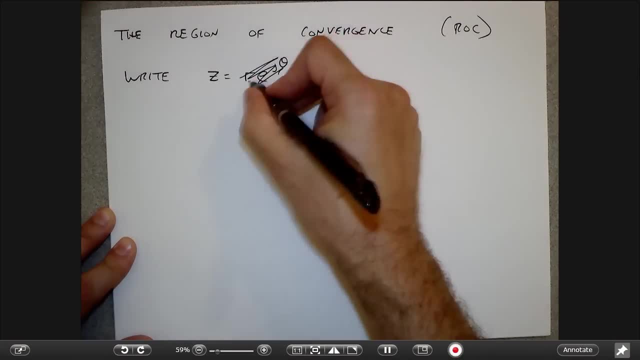 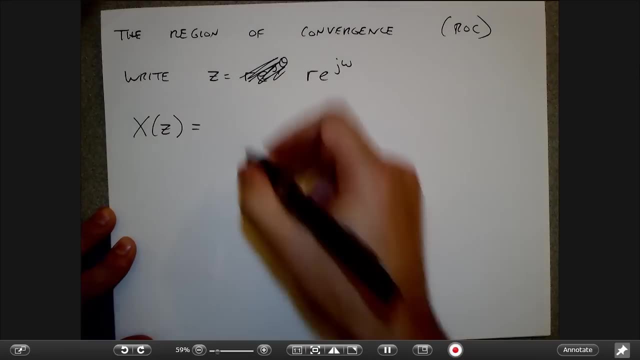 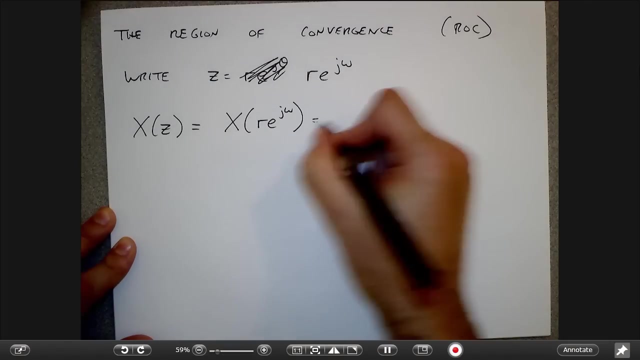 Or actually, maybe I should say r? e to the j omega. We always use omega here, And so now let's say: okay, let's look at the Z-transform in terms of writing Z in this way. Okay, well it's, you know, here's the regular Z-transform. 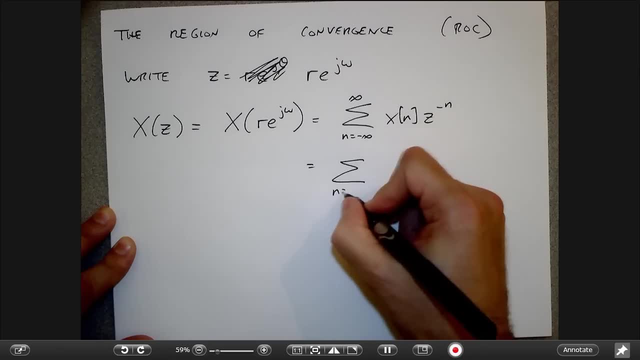 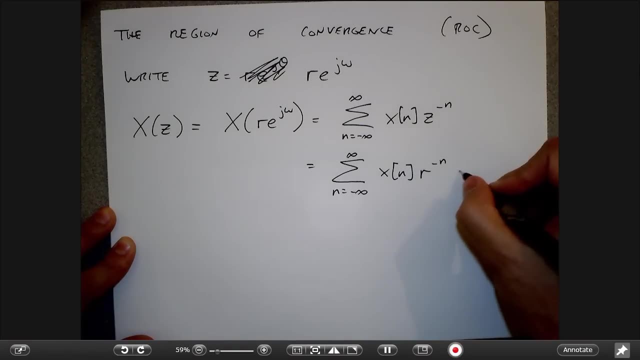 Z to the minus n. If I plug in, really being explicit about Z, I'm going to write this like r to the minus n, e to the minus j, omega n. And if I look at this, if I kind of draw parentheses around here, 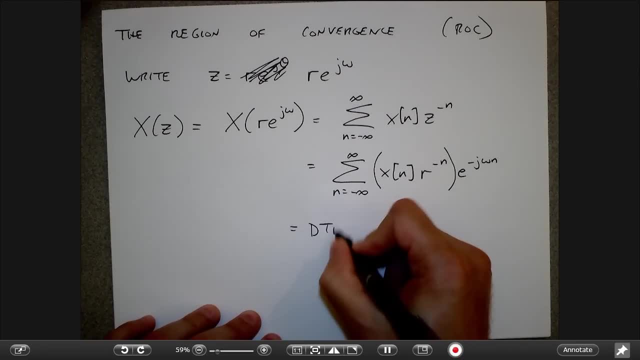 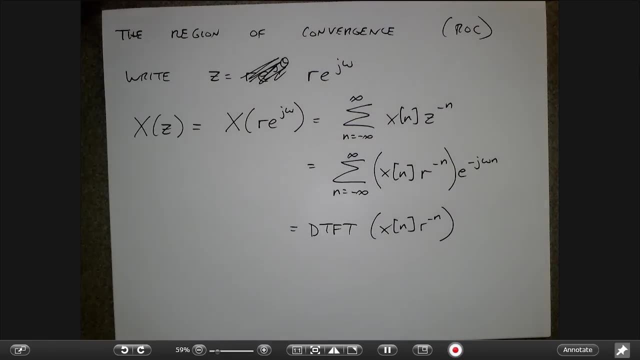 this is like saying, this is like the DTFT of some kind of modified signal, right? So in some sense, what I'm saying is I'm taking the DTFT of the original signal, kind of modified by this r, to the minus n. 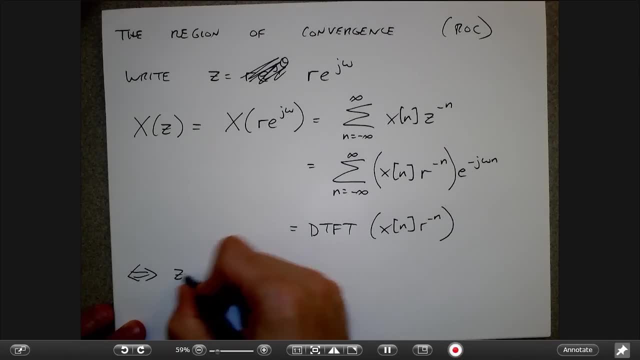 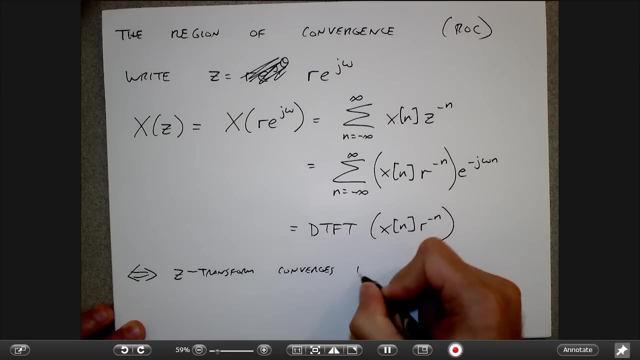 And so the way I think about this is that the Z-transform converges if I have the same condition that I had here before, And so here this is kind of making it clear that the Z-transform may converge in places where the Fourier transform doesn't right. 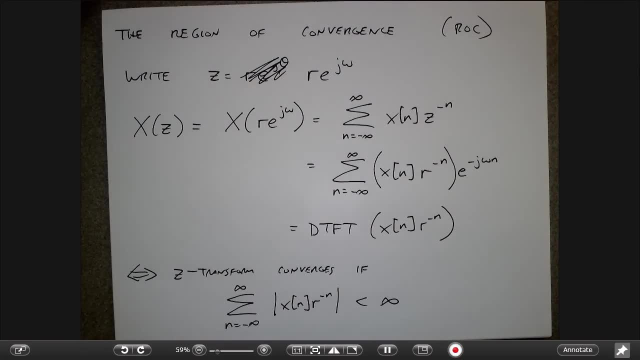 So if r equals 1, and this convergence thing at the bottom is true, then the DTFT exists and the Z-transform also has a region of convergence that includes r equals 1.. But it's also possible that for changing this value of r, 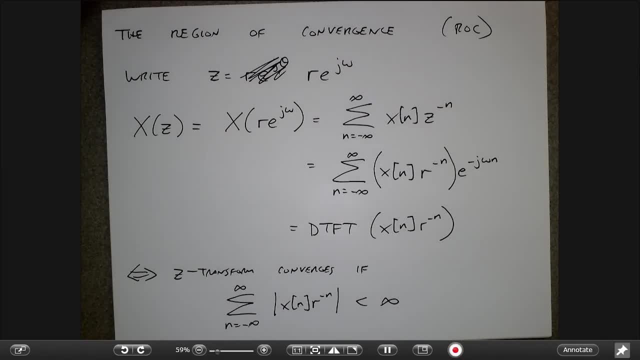 you know, it may be true that r equals 1 does not satisfy this criterion. but if I were to crank up r, basically if I were to, you know, dampen down the original signal by multiplying it by some decreasing exponential, 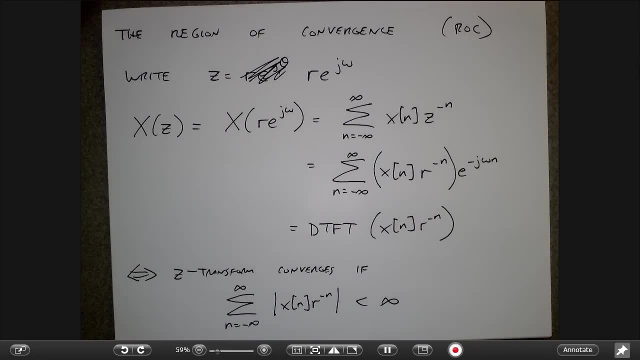 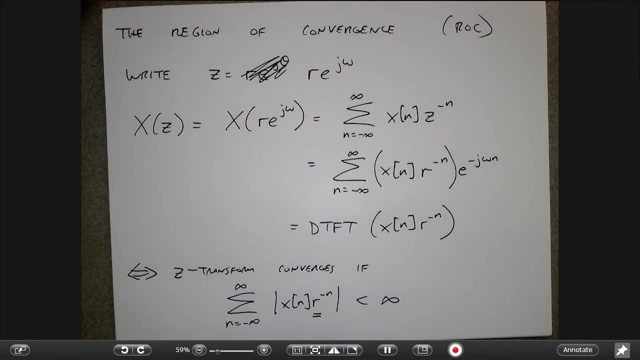 maybe I could get. maybe I could get the sum to converge and the Z-transform would exist for that certain value of r, right? So what I'm kind of doing is I'm looking to see what is the range of r for which this sum converges. okay. 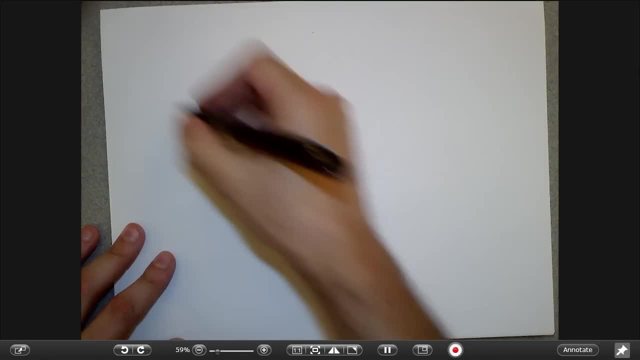 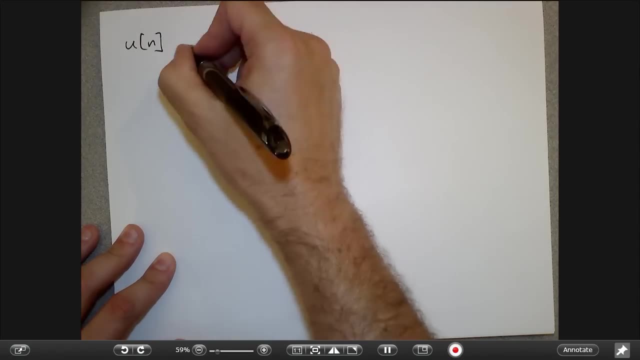 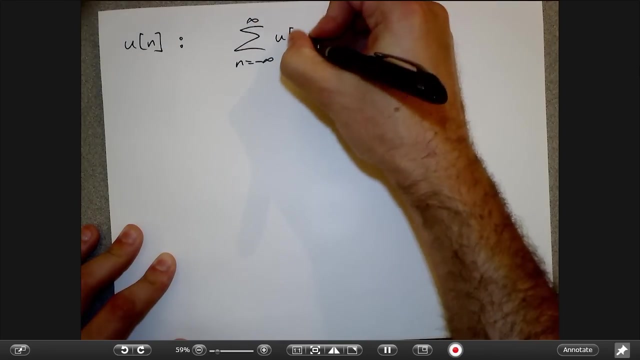 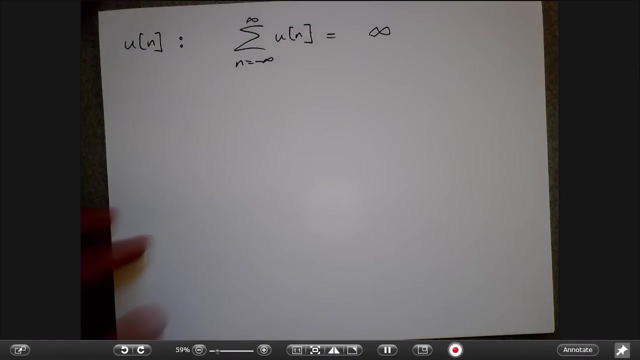 And so, just to make an example, so let's consider the step function. okay, So the step function. certainly, if I were to look at this sum right, well, I would get infinity Right, Because I'd be adding up, you know, all those numbers. 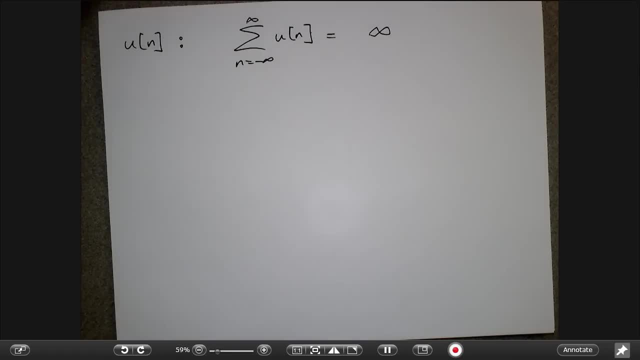 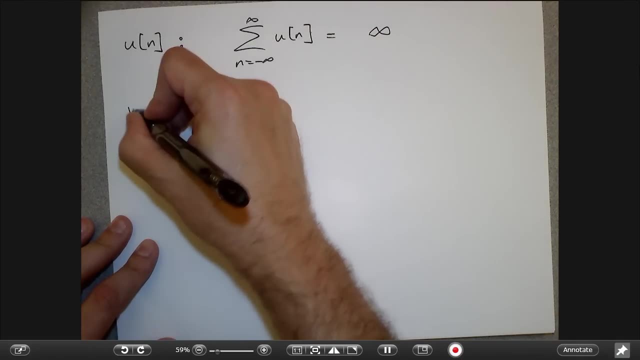 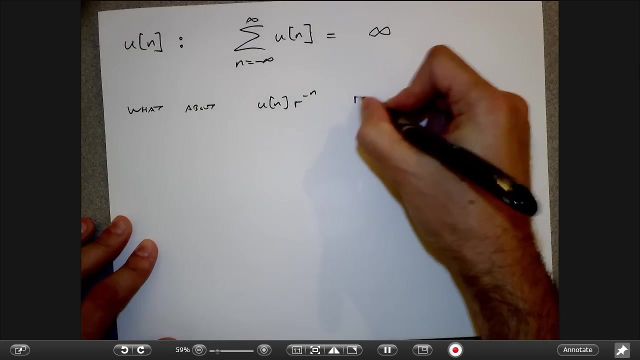 So I can't take the Fourier transform of the step function right. Not possible to do. However, if I were to look at, you know u of n? r to the minus n for some real r, well, I would get infinity. 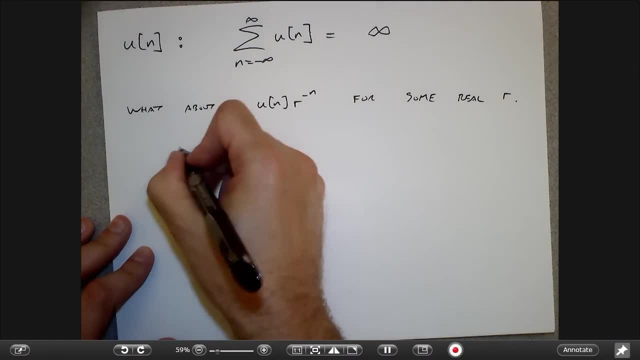 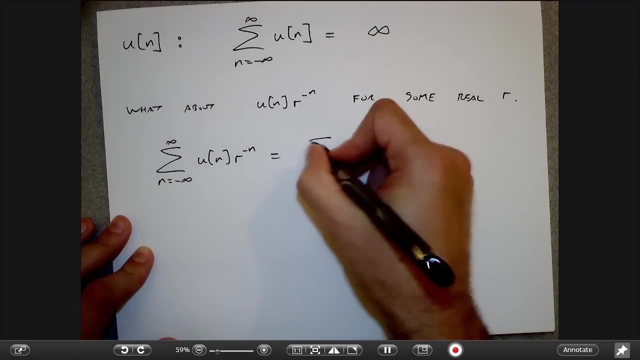 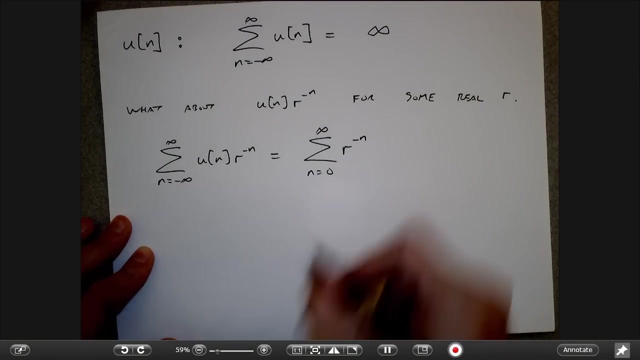 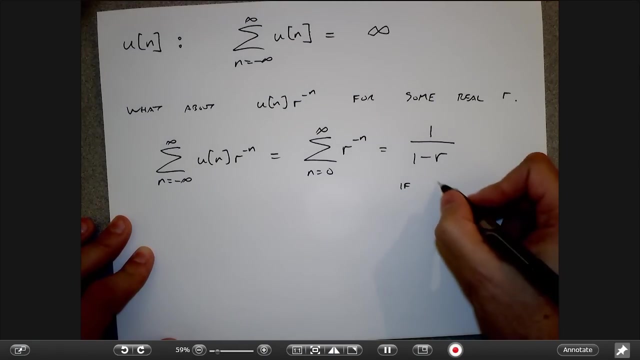 Right, Okay, In that case the sum would look like this, And I would kind of get up the step, function like this, And here I would say, okay, well, this would be equal to, you know, 1 over 1 minus r, if. 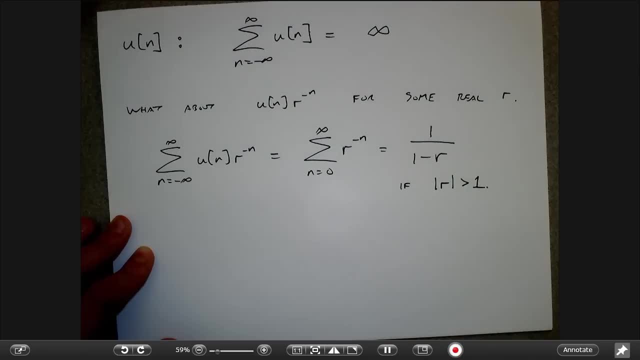 this magnitude was greater than 1.. Right, Because what I need to do is right. A different way of looking at this: is this right? I could also write it like this: Hopefully that makes it a little bit more obvious. When I have an infinite series like this, I need to make sure that each of these terms 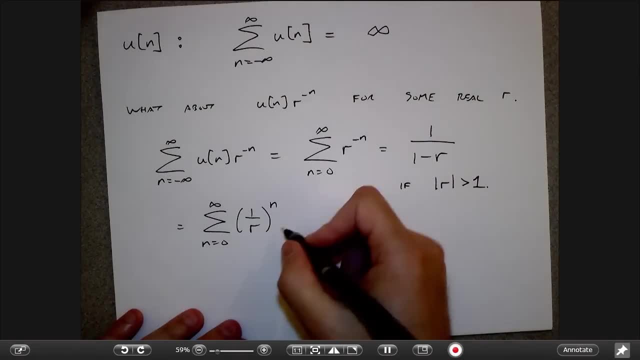 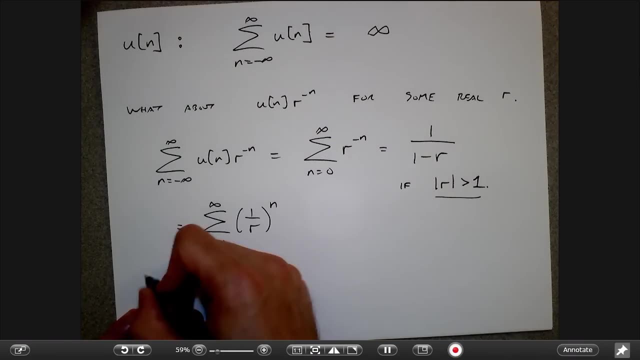 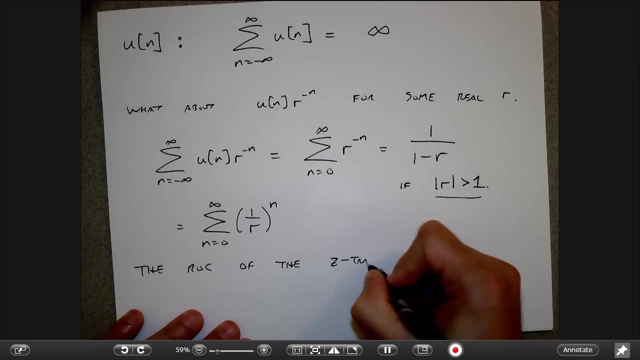 right is less than 1.. And so this is going to converge in this region, right. And so if I was going to say you know the ROC of the n-th right, Sorry, No, the Z transform of u of n is the magnitude of r greater than 1, and the way 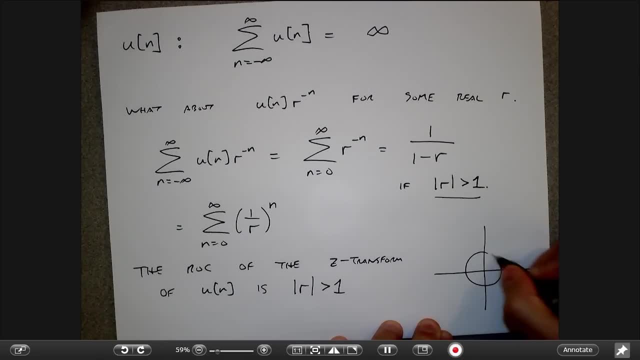 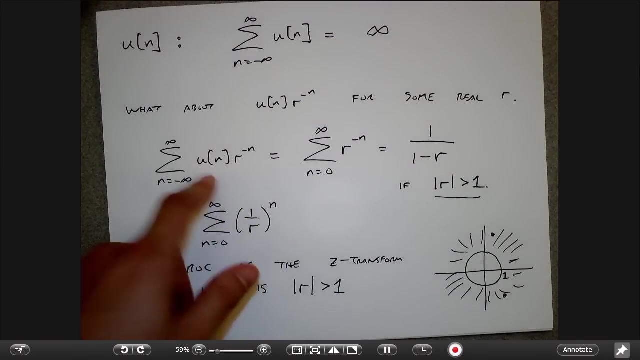 I draw. that is like so. So I draw a unit circle here and then I kind of draw this sunburst that says that any Z that I pick out here will satisfy this constraint and therefore this sum will converge and I can talk about the Z transform in this region. Anywhere in here I can't talk about, because the 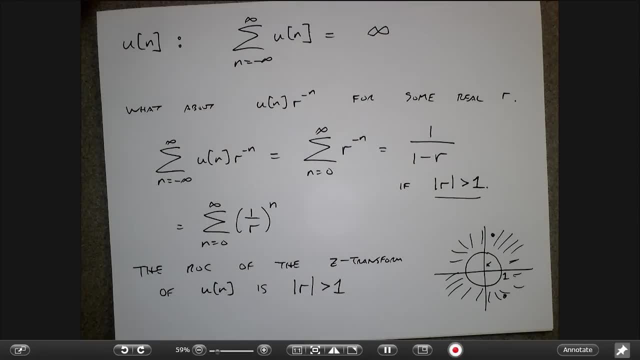 radius is less than 1 and this sum will just blow up. So again, this is a signal that I can analyze with the Z transform in certain regions of the complex plane, but I can't analyze with the Fourier transform. So, and here you can see, 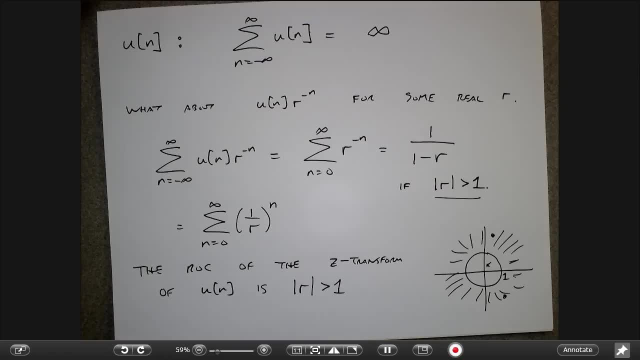 a question: Is this supposed to be called 1 over 1 minus 1 over r, instead of 1 over 1 minus r? Oh yes, this should be like this, right? Yeah? sorry about that. Yeah, that was a little bit too quick, So that's the same as this, right? Yeah, you're right, good. 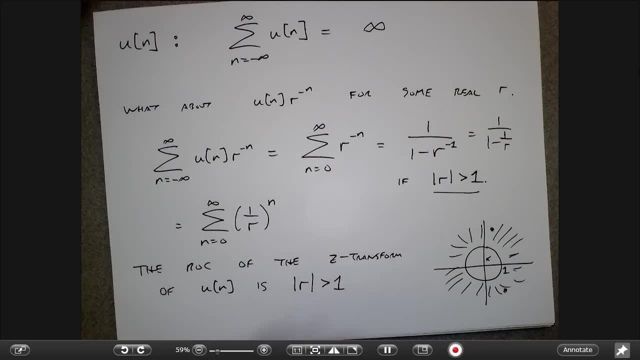 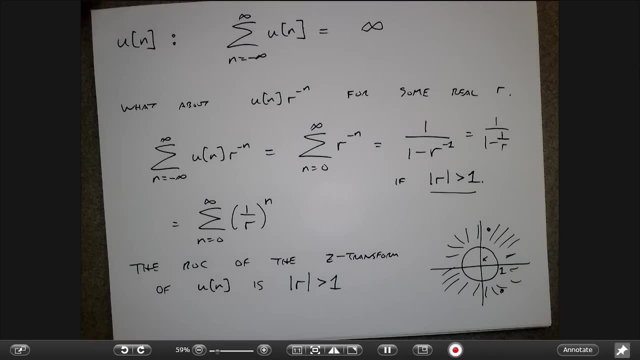 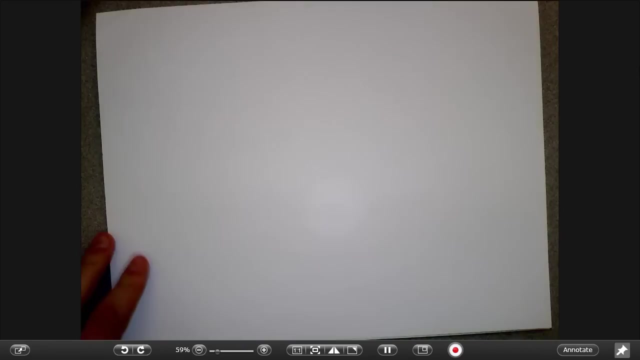 quick point, Sorry about that. Other comments or questions: No. So you can see here that because everything here depends on r, my regions of convergence always involve circles in some sense, Circles in the complex plane that are center to the origin. So a different way to say this is that you know. 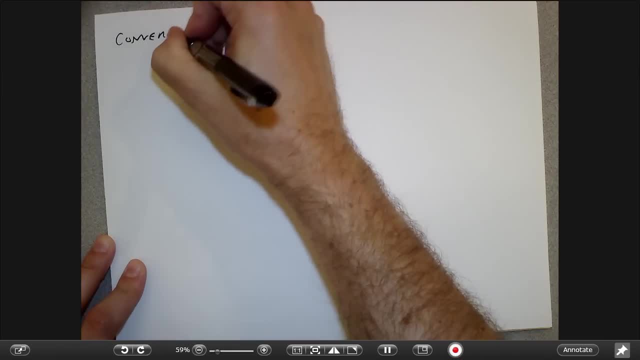 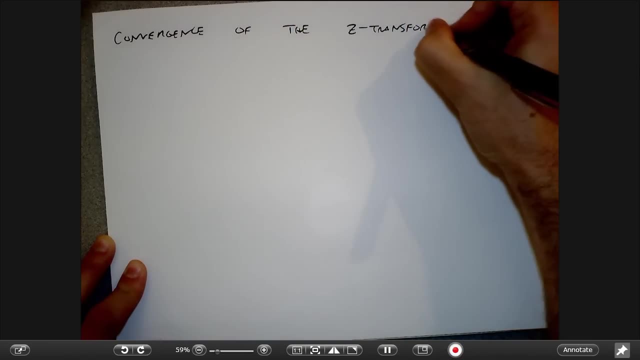 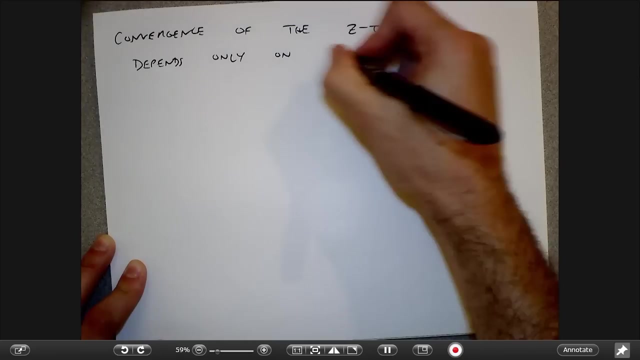 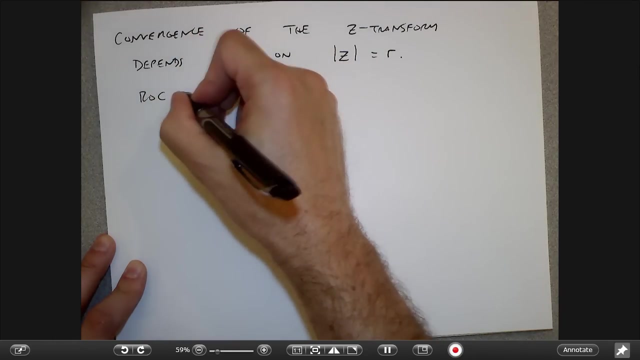 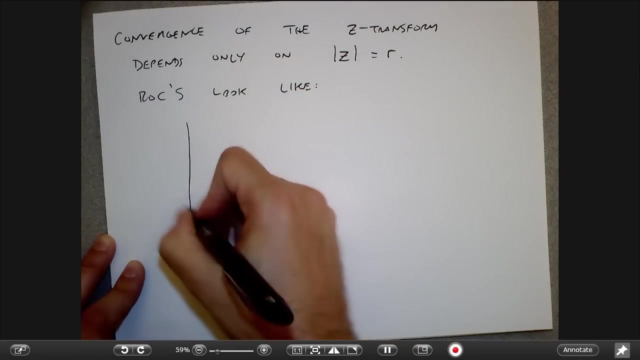 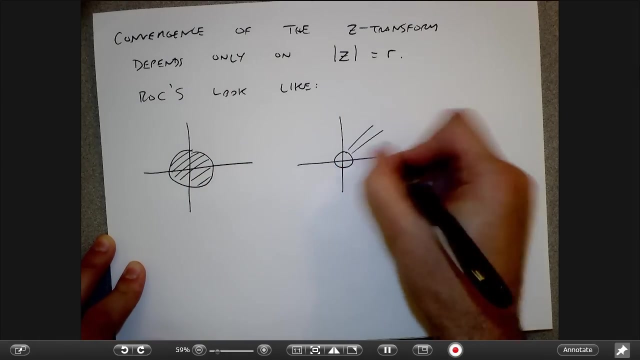 convergence of the Z transform depends on r. It depends only on the magnitude of Z, which I was calling r in the previous slide. So that means that regions of convergence look like things that only depend on the radius. So I could have a region of convergence that looks like this: The one I showed you in the previous example looks like everything outside of a circle. 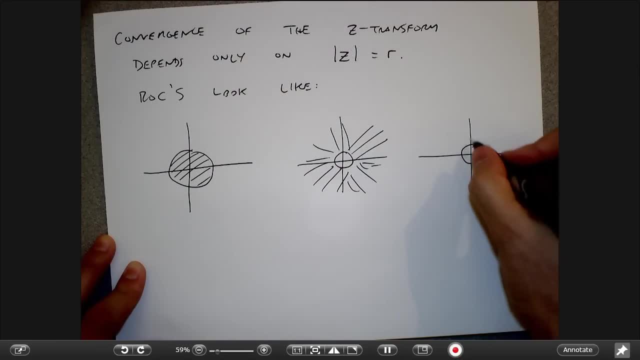 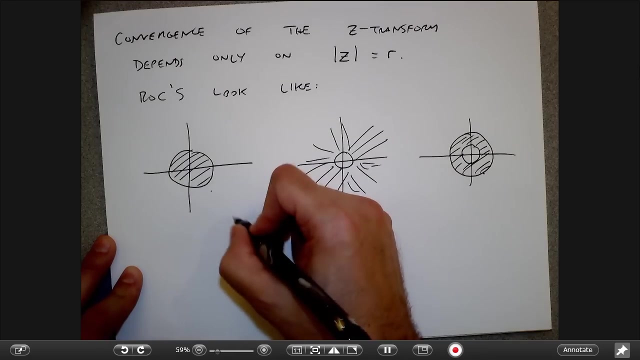 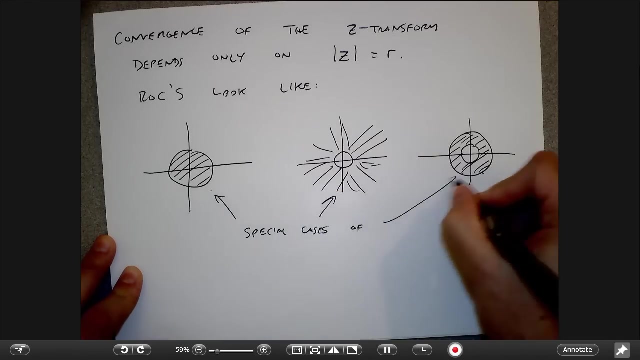 I could even have something like this, where I have things that are between two circles And so I mean, in some sense, these guys here are actually kind of like special cases of this guy here, right? So if I were to take this guy and say, okay, now I'm going to let the outer circle 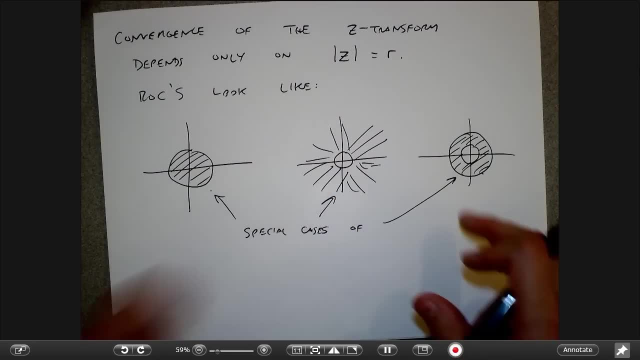 go on to infinity, I get a picture that looks like the sunburst. If I take this guy and say I'm going to take the inner circle and bring it down to zero, then I get this circle In some sense. ROCs generally look like this something. 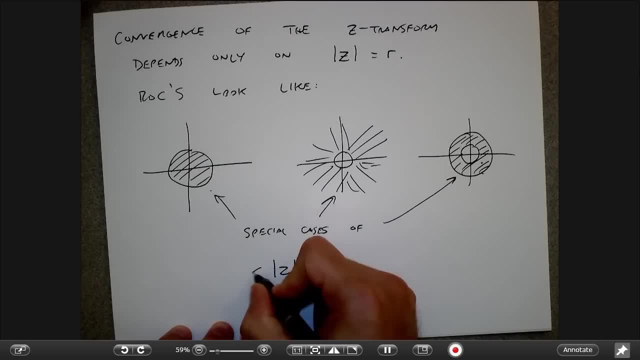 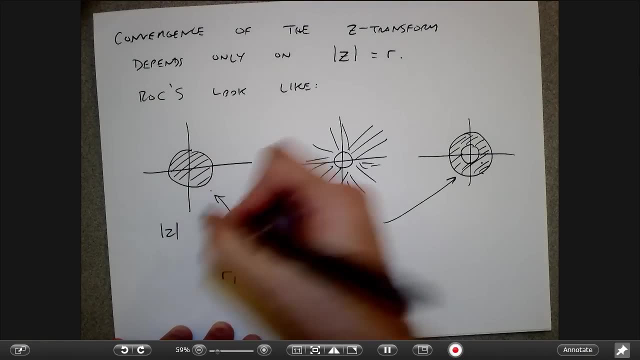 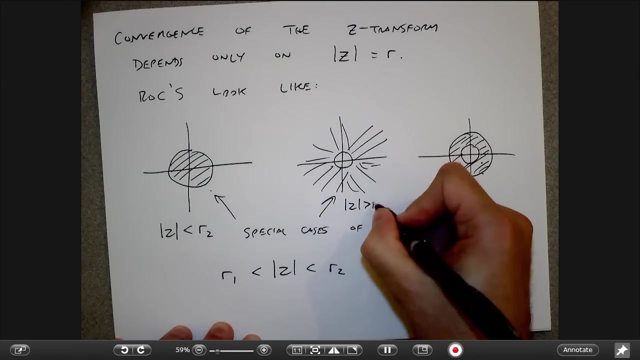 like the magnitude of values like this: It's possible that if I were to take in the limit, this is like saying I have the absolute value of z less than something, and it's like saying the absolute value of z is greater than something. Okay, And so. 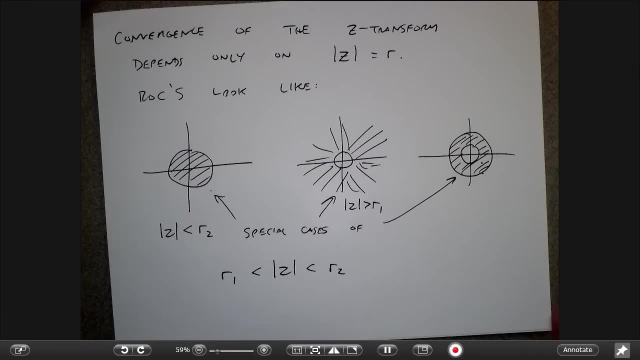 as I mentioned, kind of to motivate this, when the ROC includes the inner circle, that means I can talk about both the z transform and the Fourier transform. So if the ROC includes the inner circle, then the DTFT exists, Which is a way of saying that that DTFT 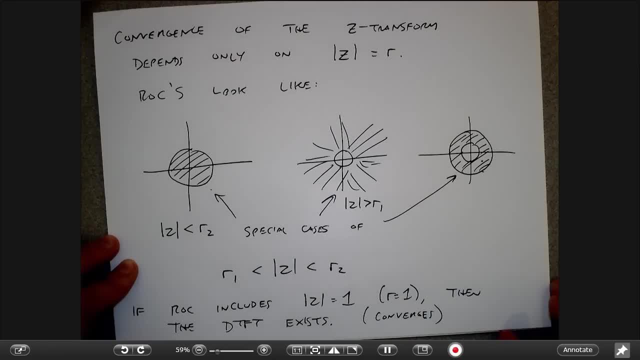 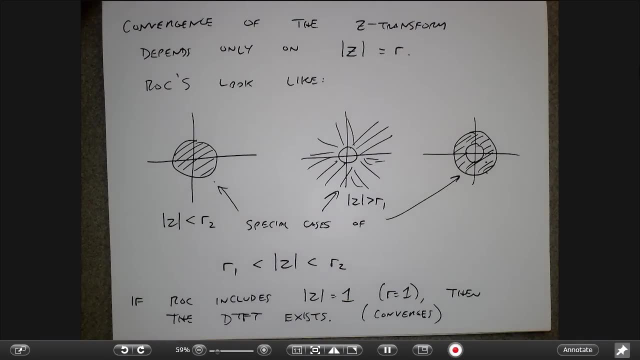 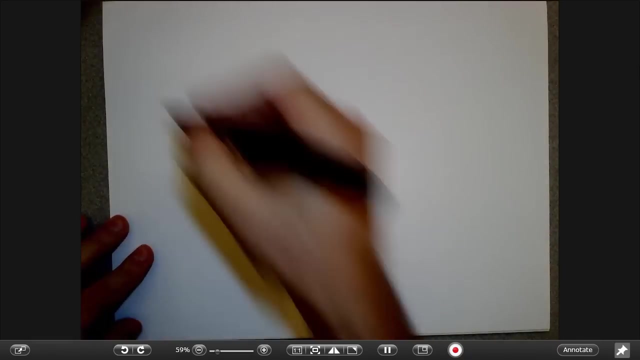 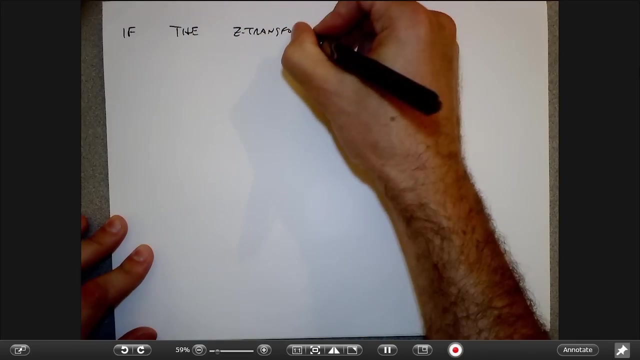 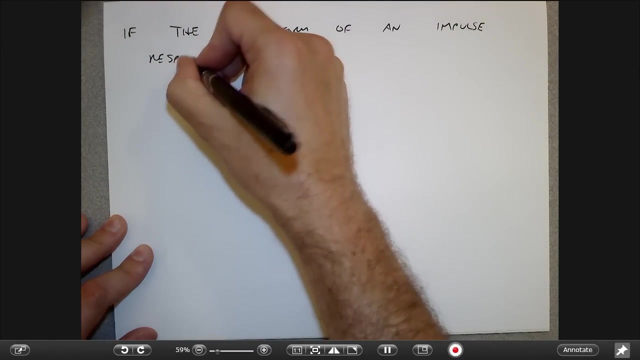 sum converges, Okay, And so this converges, And the convergence of the DTFT has a special name, Okay, And that's called stability. So if the z transform of an impulse response h of n for an LTI system, 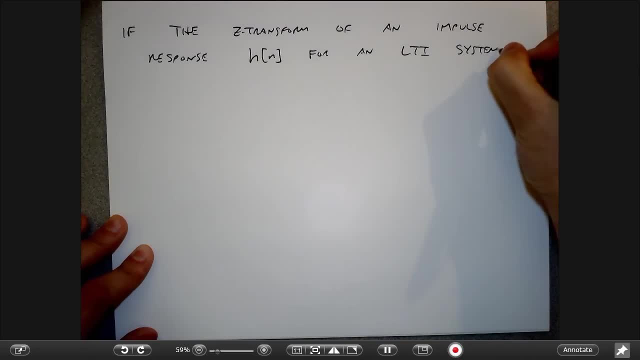 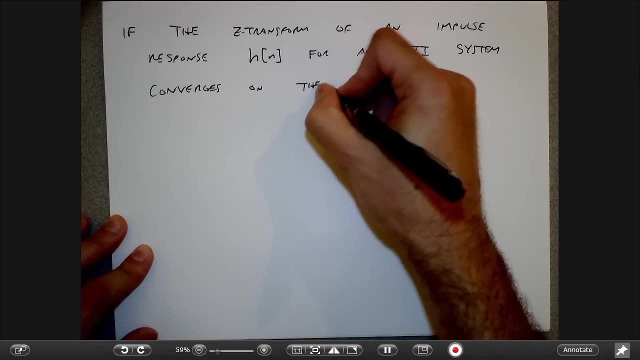 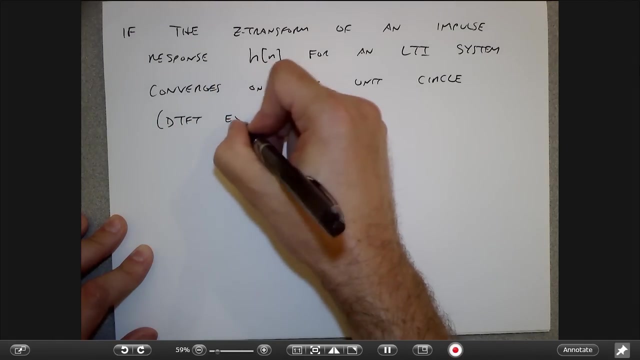 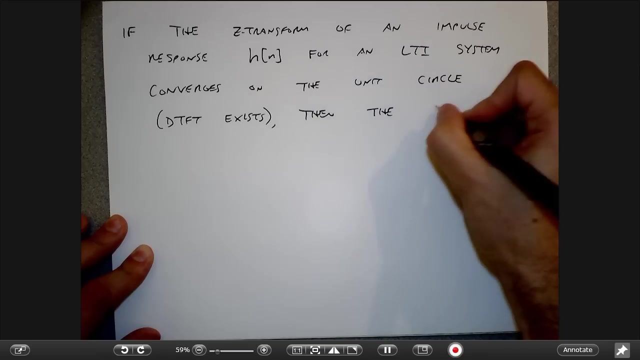 converges on the inner circle, which is another way of saying that the DTFT exists, then the system is stable. Okay, So if the z transform of an impulse response h of n for an LTI system converges on the inner circle, 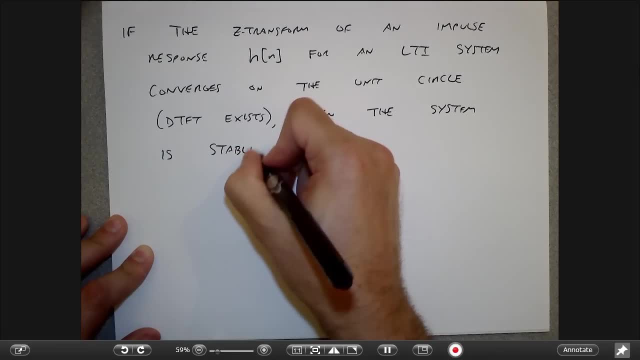 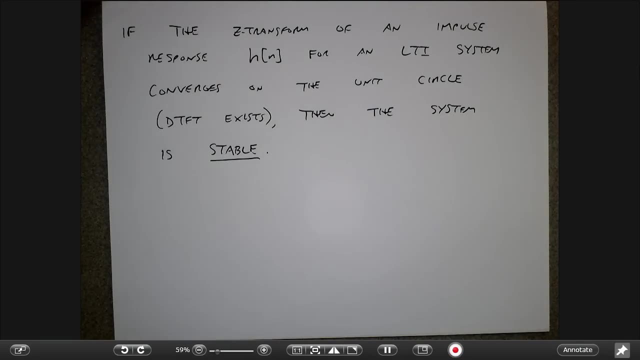 which is another way of saying that the DTFT exists, then the system is stable. Okay, So we're going to talk a lot more about stability and what it means in future lectures. Right now, this is more of a definition than anything else. 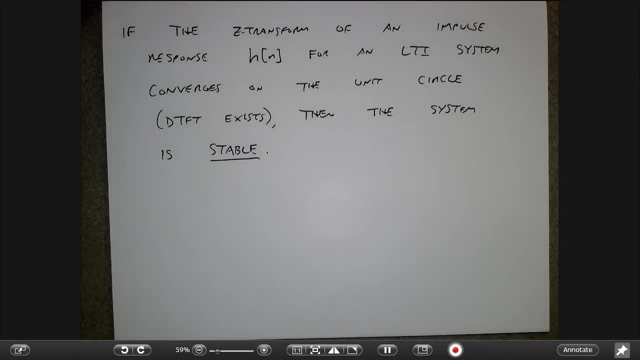 Right, Just saying that. you know, we call the system stable if it has a Fourier transform, Okay. And in some sense the stability of the system means the system is doing good things. It means that if I put some arbitrary input in the system, 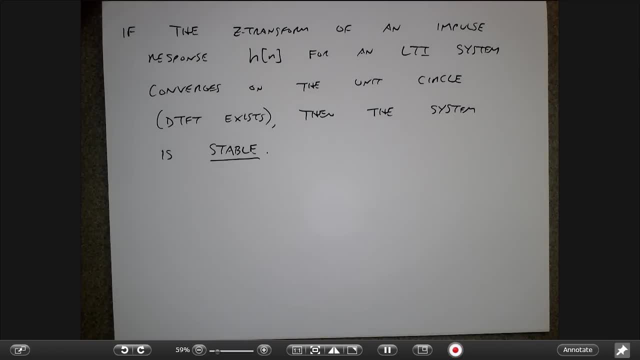 it can't do crazy things that produce some output that explodes out to infinity Right. It kind of means that the system is in general well-behaved. I'll talk about kind of more what that means in just a second Or in a few lectures maybe. 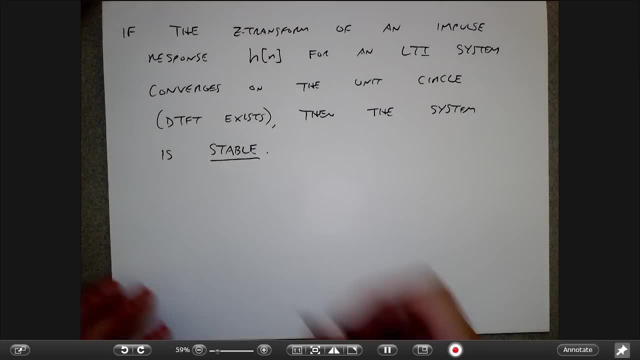 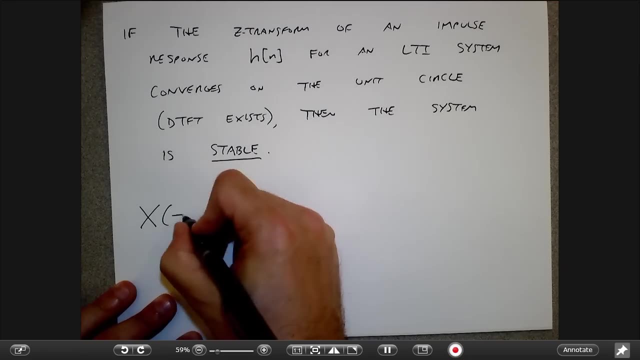 Okay And so Okay. So, as we're going to see- I'm just going to make a note of it now- that a lot of times we can write the z transform as some numerator over some denominator, Where the z transform is a constant. 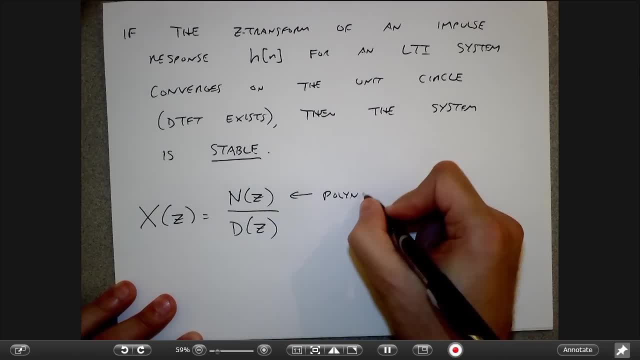 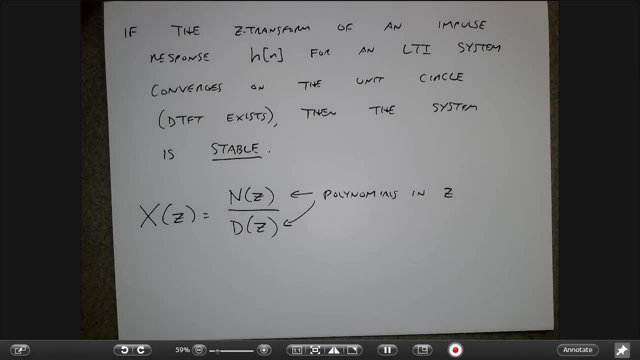 Where these are both polynomials and z, And some of the examples that we're going to do next are going to be in this form. Okay, And so there are kind of two interesting things Right. One is that when the numerator is zero, 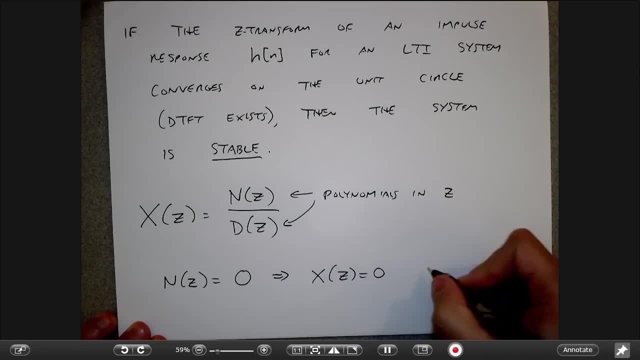 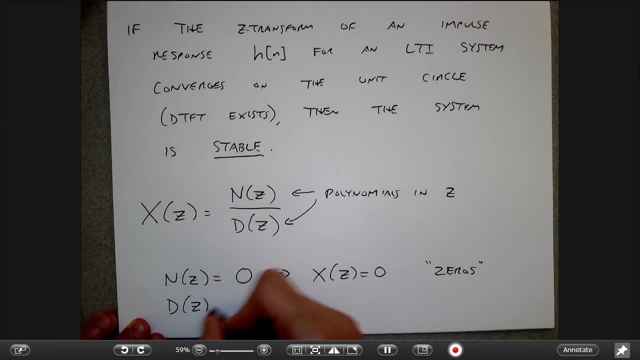 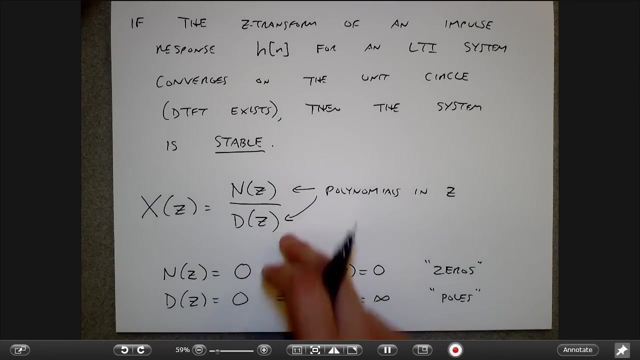 that means that the z transform is zero, And these are naturally called zeros of the transfer function. And when the denominator is zero, that means that this thing blows up to infinity, And we call these poles, And so there are important connections between the zeros and the poles of the polynomials. 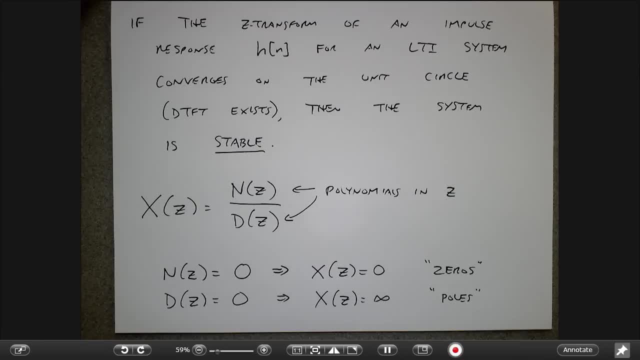 and the ROC of the z transform. So we're going to talk about that in a moment here. But as you'll see, especially when we come to filter design, a lot of filter design is all about understanding where the zeros and the poles of the transfer function are. 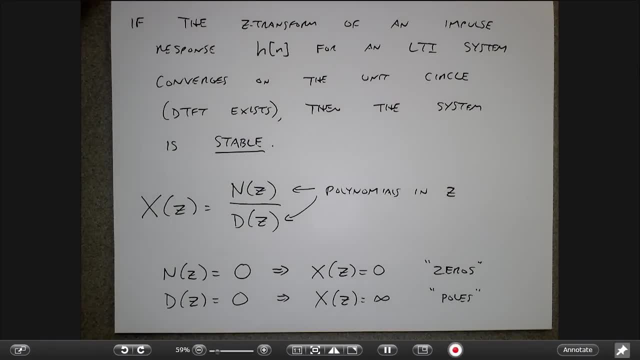 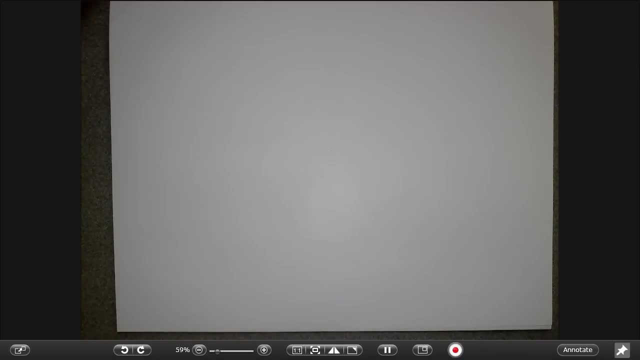 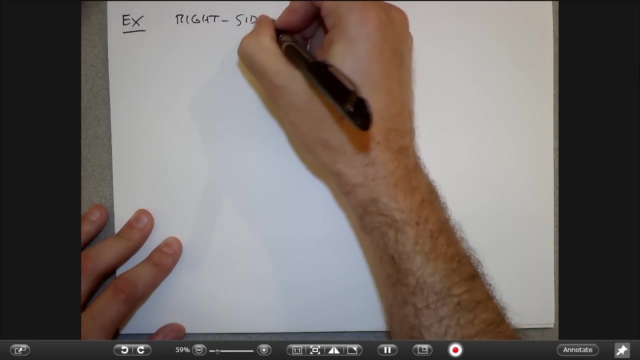 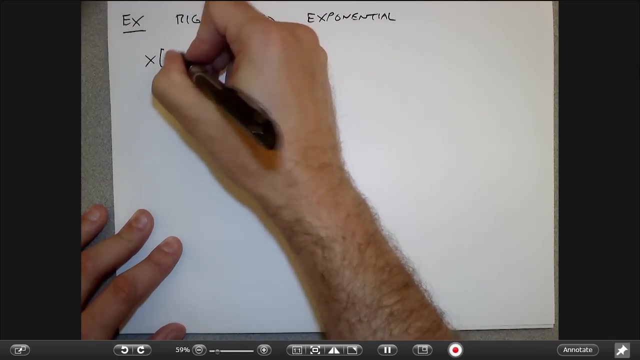 in order to make the filter do what I want it to do. So let's do an example of an exponential sequence. So what I'm going to call this is a right-sided exponential A to the n? u of n, And so 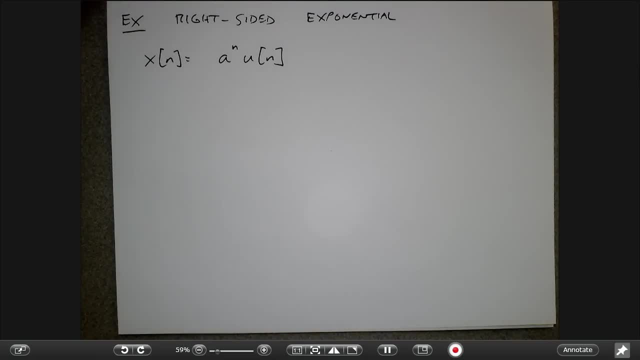 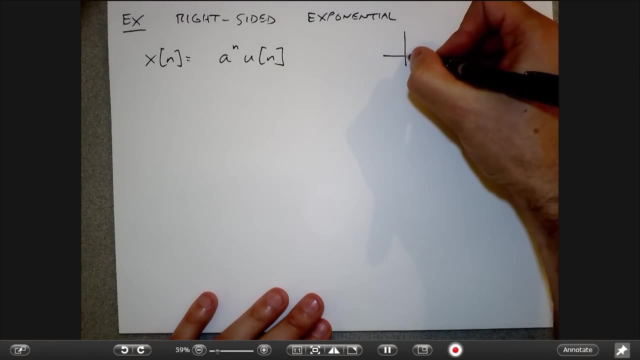 it's called right-sided because it only starts at zero and then it goes on to infinity off to the right-hand side, And so when the magnitude of a is less than one, I get kind of a decreasing exponential. When the magnitude of a is greater than one. 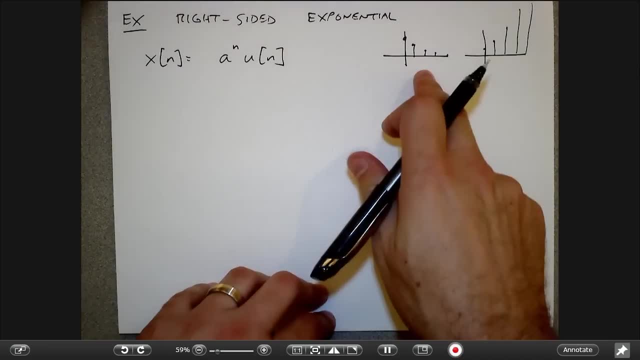 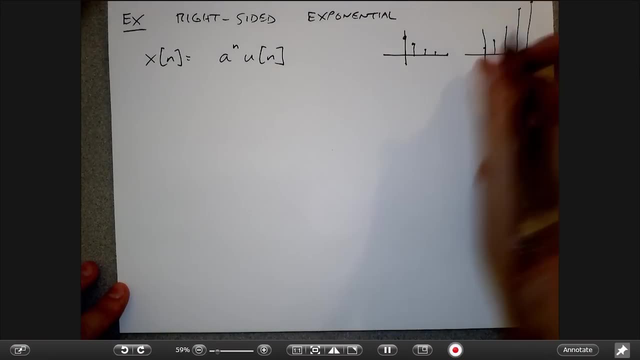 I get an increasing exponential, And so you can kind of already predict that the ROC has to do with when a is less than one Right. Otherwise I'm never going to get sums that converge with pictures that look like this. So 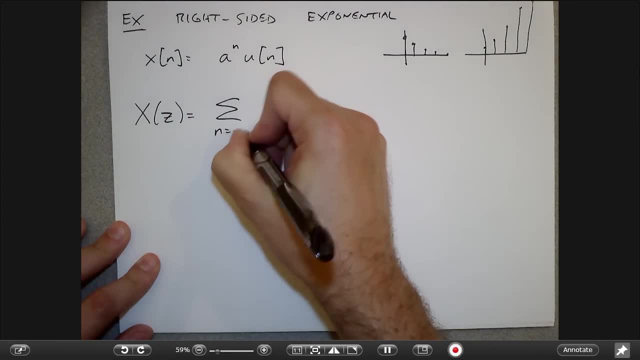 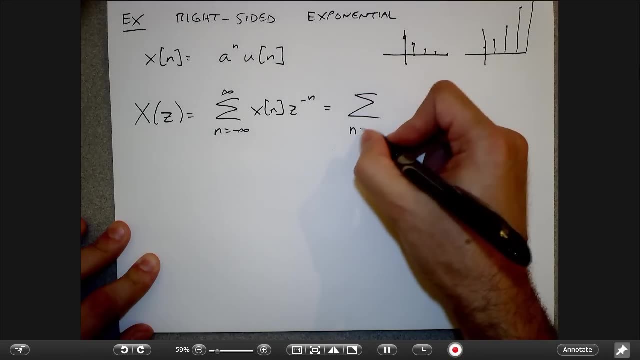 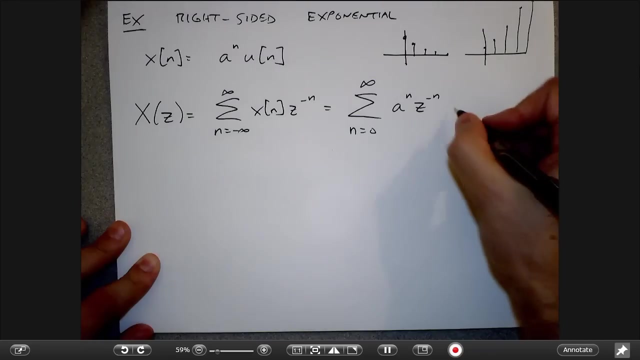 let's actually compute the Z-transform X of n. Z to the minus n. In this case, this turns into: from n equals zero to infinity, a to the n, Z to the minus n, Which is a different way of looking at it as. 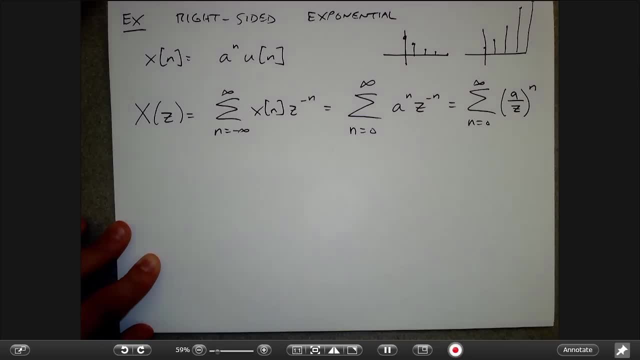 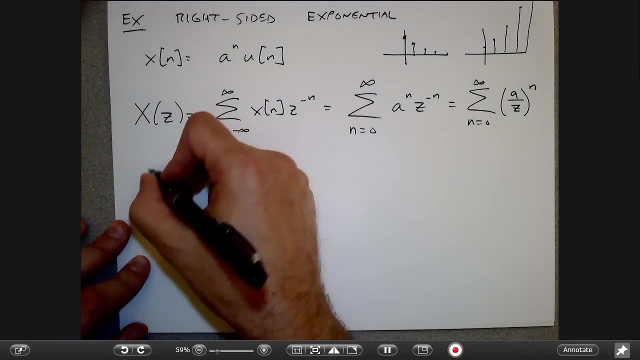 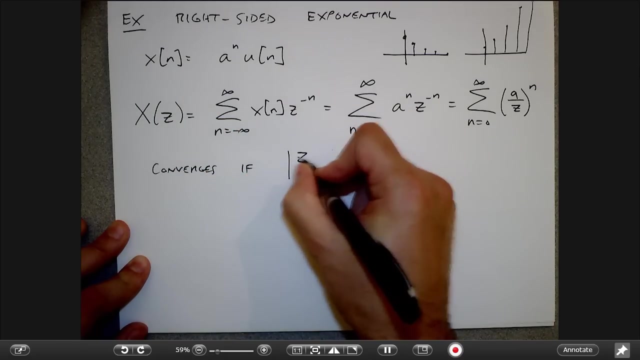 a over z To the n Right, And so what I need here is so this will converge, If I guess I should say it this way- if this absolute value here is less than one right, We know that from our infinite sum formula. 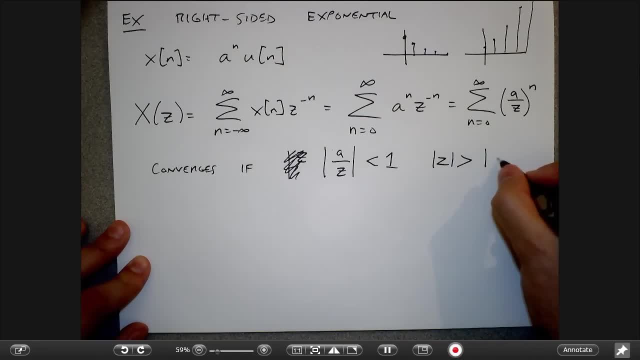 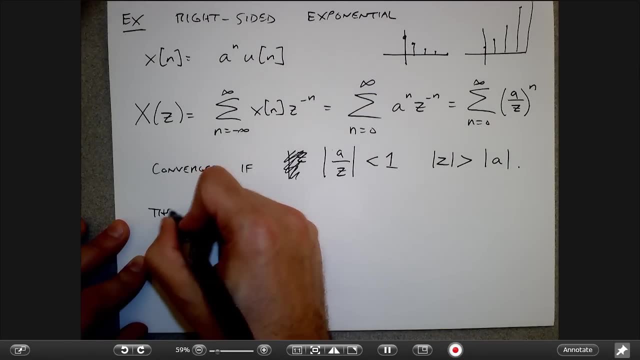 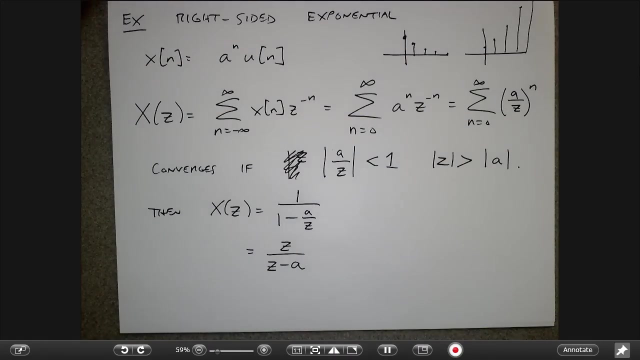 which is a different way of saying, must be greater than the magnitude of a. and if that's true, then the value it actually converges to is this: 1 over 1, minus a over z, which is, if I multiply by z, all the way through like this, and now here I can draw what's called. 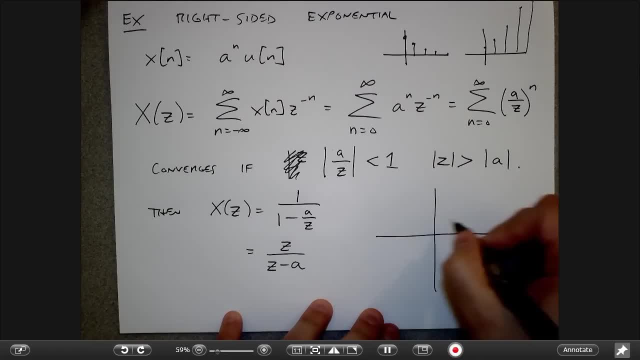 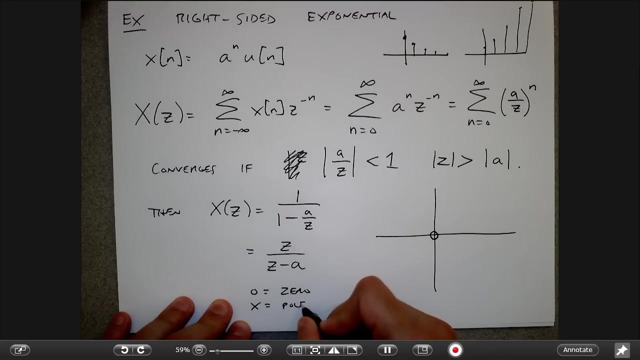 the pole zero diagram, which means that I can make a plot of say: okay, there's only one place where the z transform is zero, that's z equals zero. and I draw this circle here to indicate a zero, and I draw an x to indicate a pole, and so I have a pole over here at a. 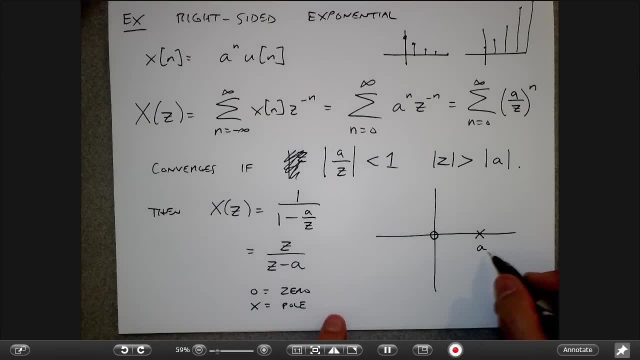 here. in general, a could be some complex number- I'm drawing it right now as if it's a positive number- but in general looks like this: and then my RO c is going to be a circle like this and everything outside of that circle is going to be in the ROC. 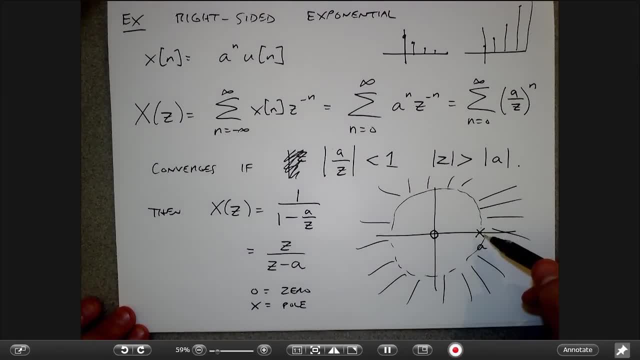 so I can see here that if a is strictly less than one, then the ROC includes the unit circle, because that sunburst is going out beyond the unit circle and the Fourier transform exists. otherwise the Fourier transform doesn't converge right, and so we already kind of saw that. 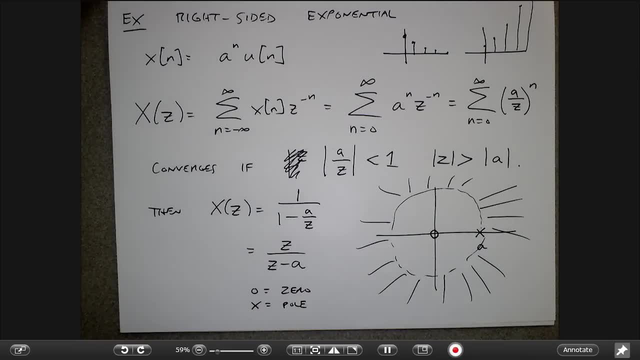 when you were doing the DTFT, that I could only look at the DTFT of signals where this number was like a quarter or a third or a half. right, I couldn't do this with a being two, otherwise the Fourier transform wouldn't exist, right, okay, so questions or comments about this. 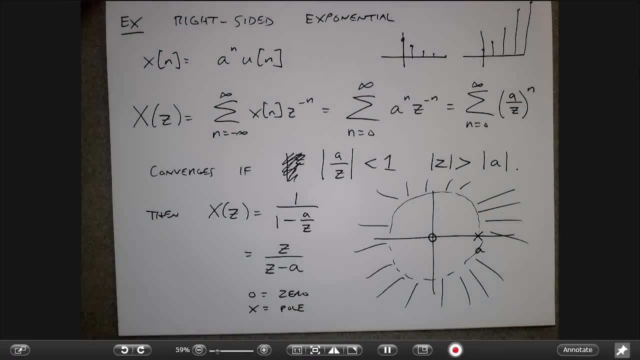 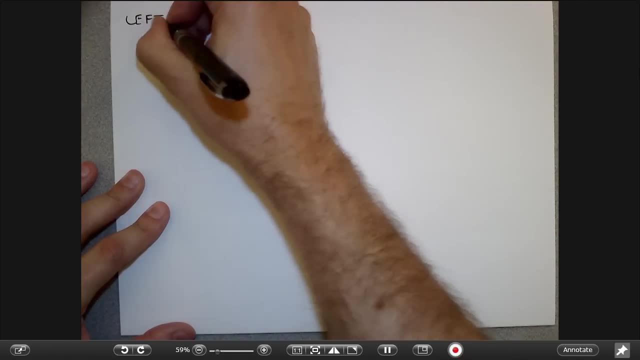 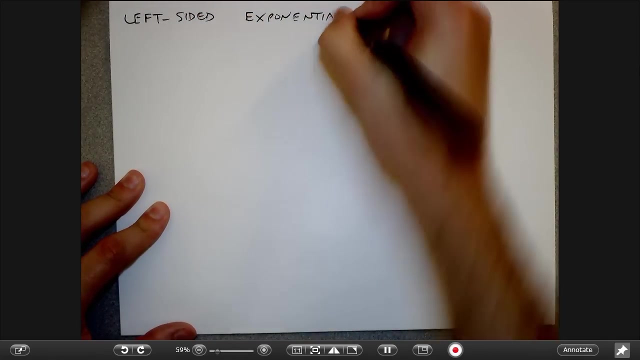 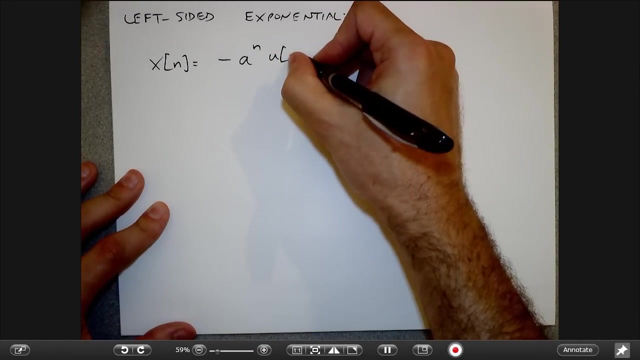 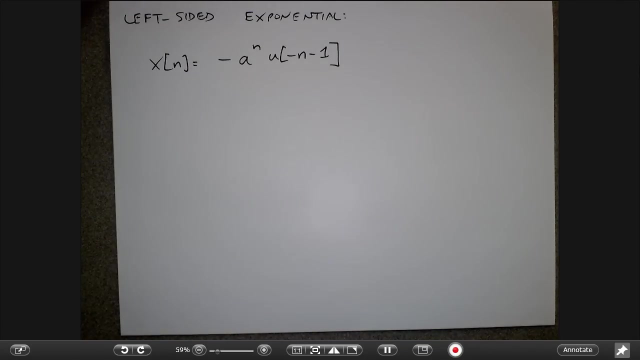 so I showed you a right side exponential. let's talk about left side exponential, right. so left side exponential, when you have مثل. but lets be positive: moins on começa, it's AL. they're not there. interesting, alright, let's keep going. the first thing I can do is let's see what are the vulnerabilities. 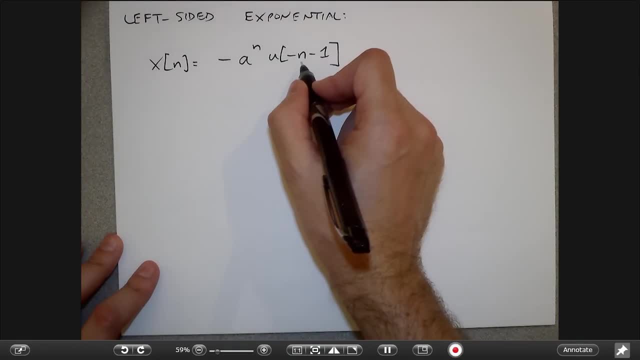 of the E 14. now let's make sure that this is true. okay, first of all, let's think about this right. so minus one right, Step function at minus one, that's zero. When n equals one, I get step function at minus two right, which is also zero. So, basically, any n greater than or equal to zero. 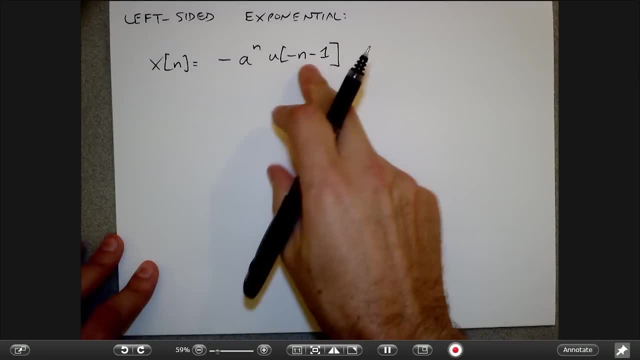 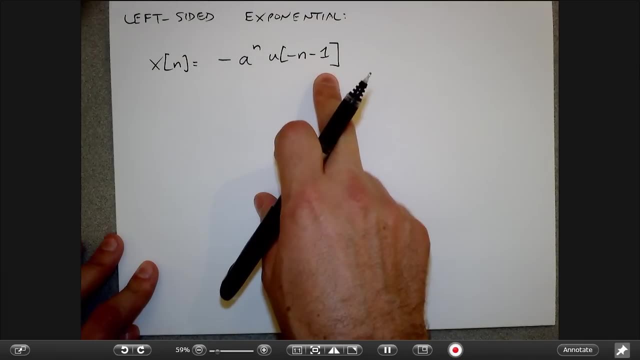 the number inside these brackets is going to be negative and I'm going to have to get any contribution, Whereas when n is minus one, I'm going to get. u of one minus one is zero. That's the first time the step function turns on right. When I have u of minus four, for example, I'm 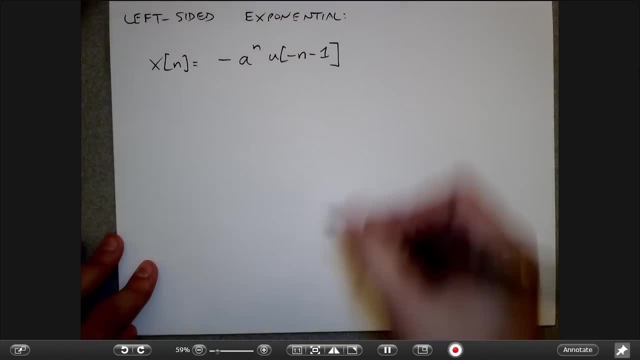 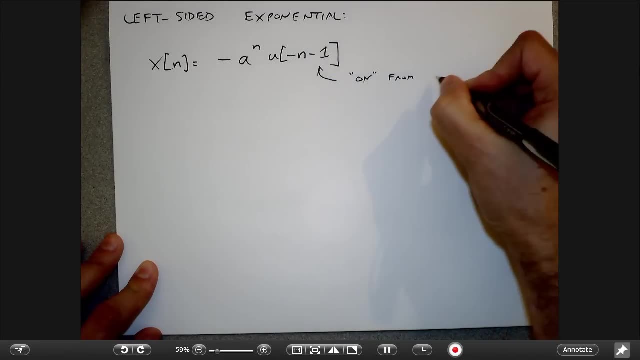 going to have u of four minus one is three, so step function will also be on there. So this is a function that basically, you know, is on from minus infinity to minus one and that turns off at zero. And so, again, I'm going to get functions that look kind of like, you know, depending on 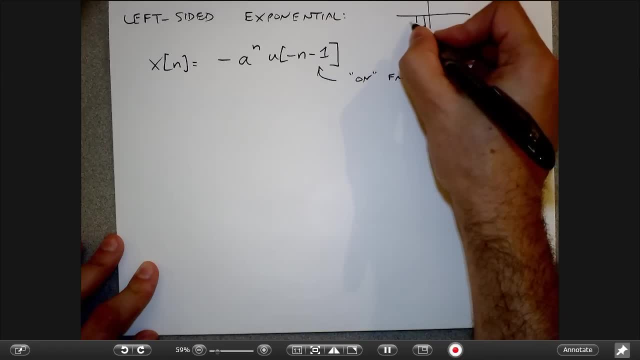 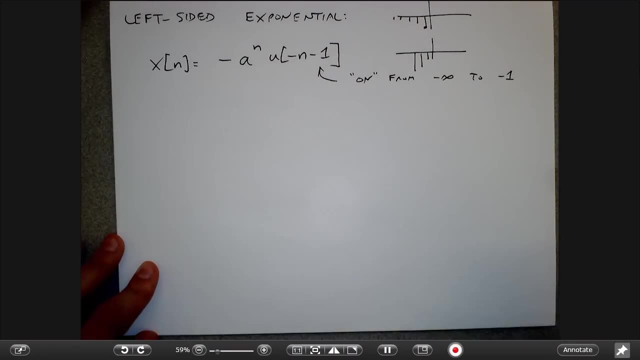 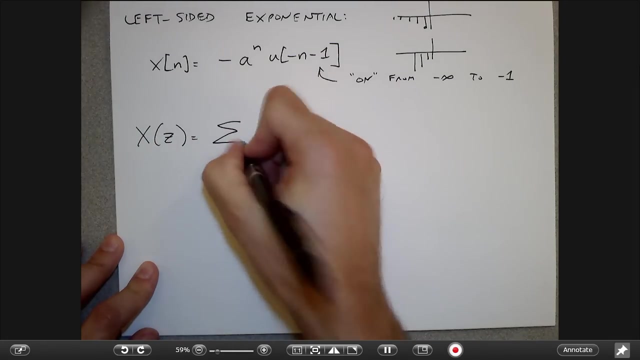 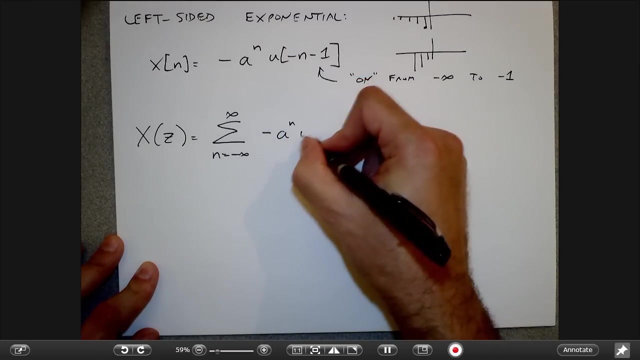 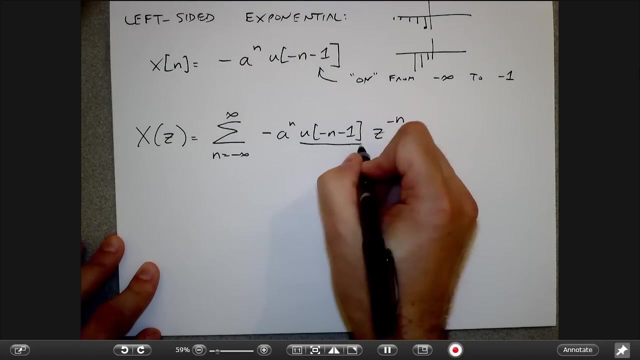 the size. it could look like something that's decreasing, like this, or it could look something that's increasing, Like that. And so let's compute the z transform. So my x of z is going to be this sum x of n, z to the minus n. And now I'm going to say, okay, well, this thing, because I know that. 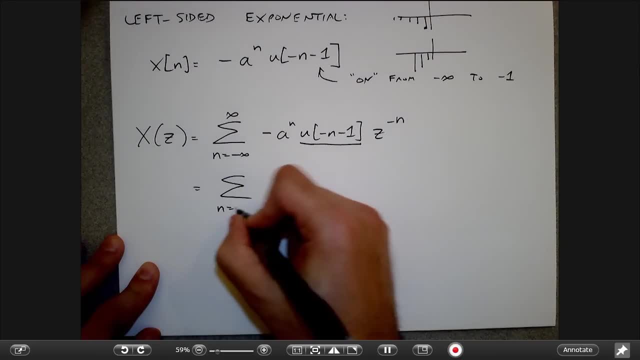 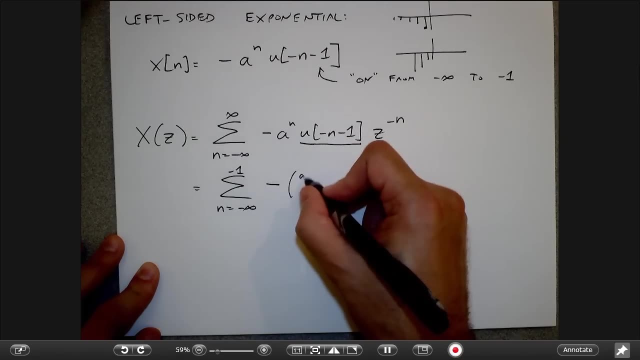 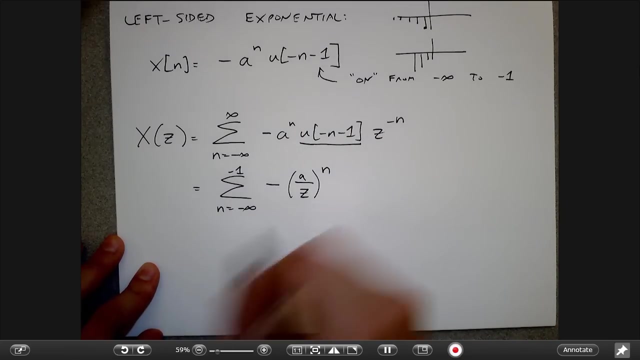 this is a step function that only turns on this way. it's going to look like this, And I'm going to have minus a over z to the n, and now I'm going to just kind of re-label what I call n Right. So instead of going from minus infinity minus one, I'm going to 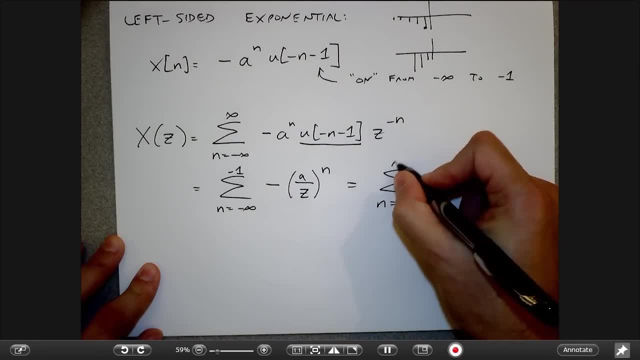 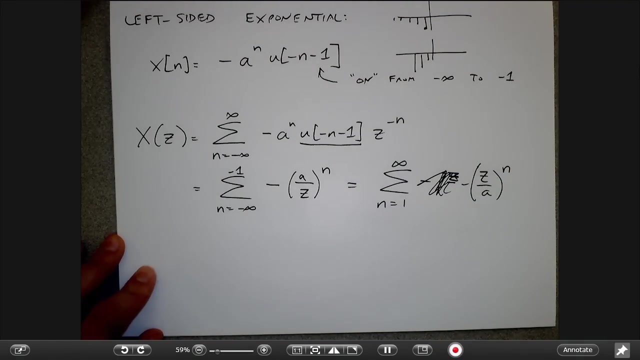 just flip this, and now I'm going to have z. sorry, I'm going to have z over a to the n. That's good, Let me write it in this part: over a to the n- power. And now this thing almost looks like a sum I can do right. So 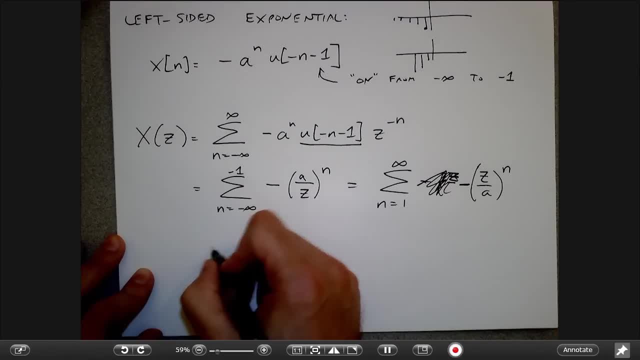 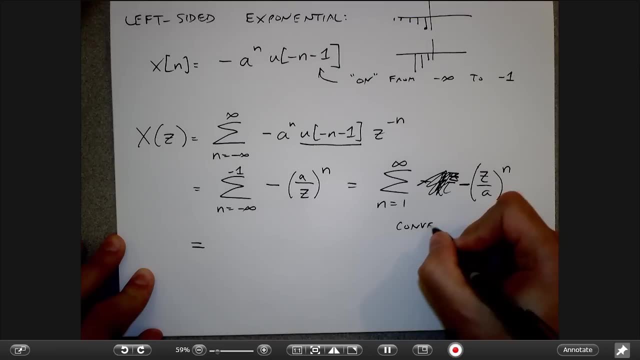 what I want to do is I'm going to say: well, first of all, again, when does this sum converge? So this converges if the absolute value of z over a is less than one right. I need to have each of these terms getting smaller and smaller, And then what is the actual value? 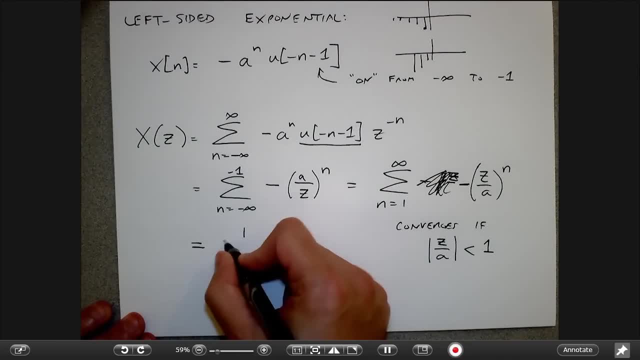 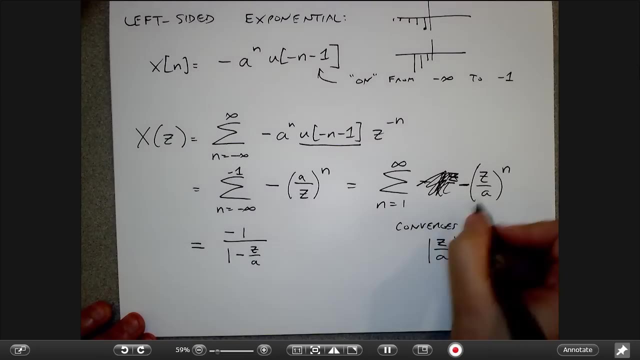 of the sum. Well, it's like one over one. Again here I've got a negative sign that comes out this way. so it's like this Minus this, And I have to subtract off. you know, actually that includes a minus one that. 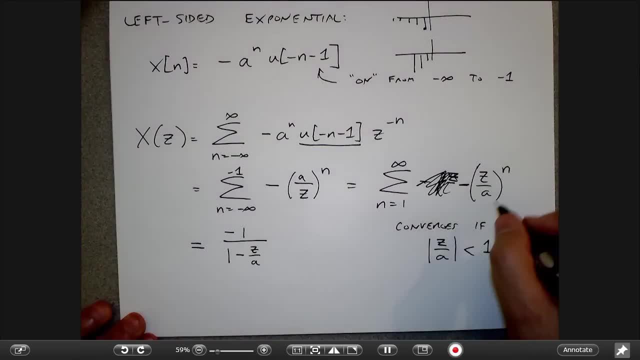 I don't let me try to do this, right? Yeah, this includes a minus one that I have to add back in right, Because normally the sum formula goes from n equals zero to infinity, And so if I write this out, what I have is minus a over. 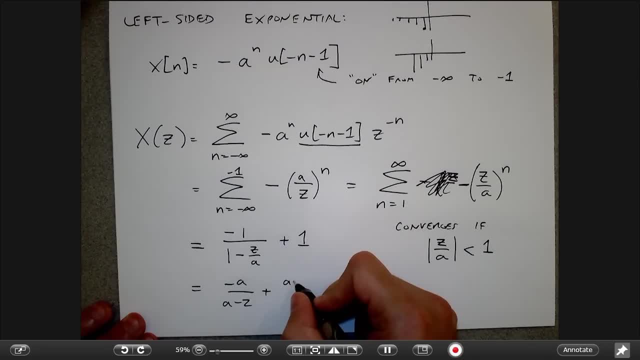 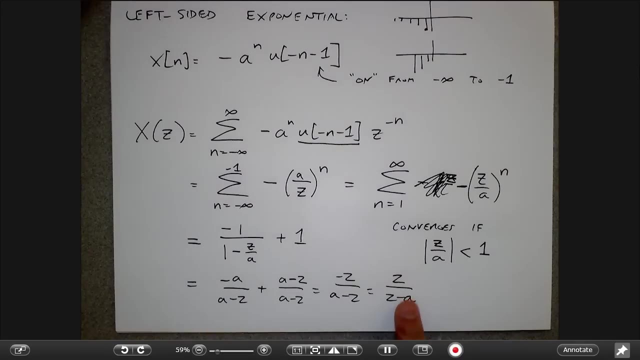 A minus z plus a minus z over a minus z, And what I get is minus z over a minus z, which is the same thing as z over z minus a. And so here's a part where I stop and say: well, wait a second. This is actually the very same z transform that I got last time, right? So 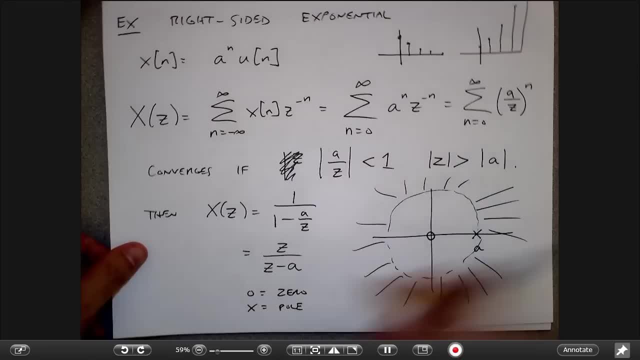 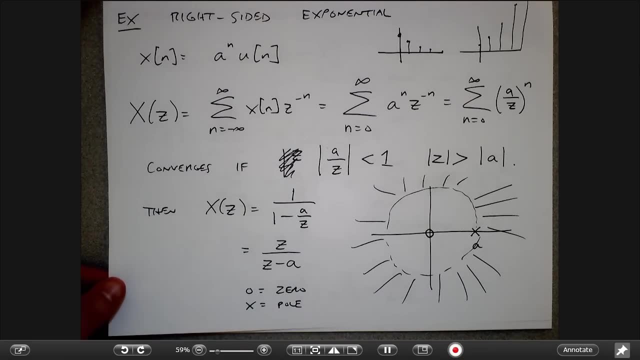 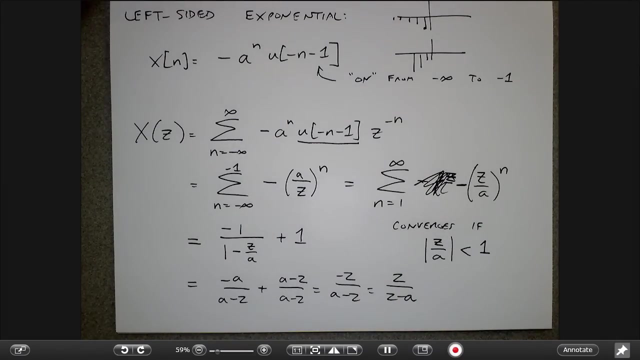 if I look back at my other example, right, I ended up with the z transform being z over z minus a right, So that seems wrong, right, It seems like I shouldn't be able to get two discrete time signals that have the same z transform. But the key idea here is that they don't have 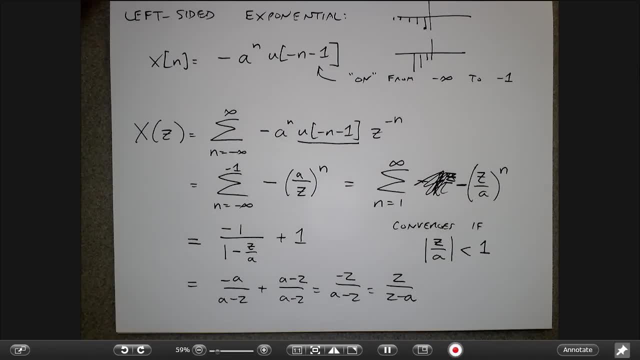 the same z transform, because the z transform comes in two parts, both this function of z and the region of convergence. And here the region of convergence is actually opposite of what we got last time. Last time we got the region of convergence being z outside. 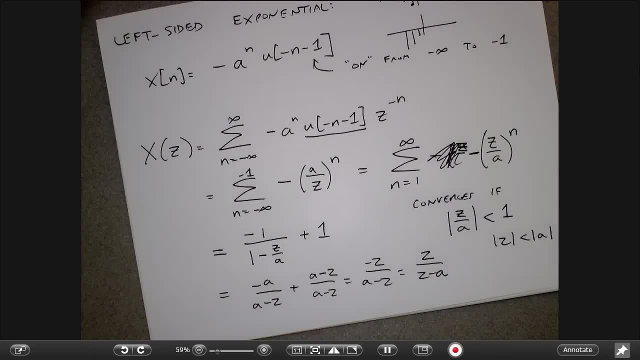 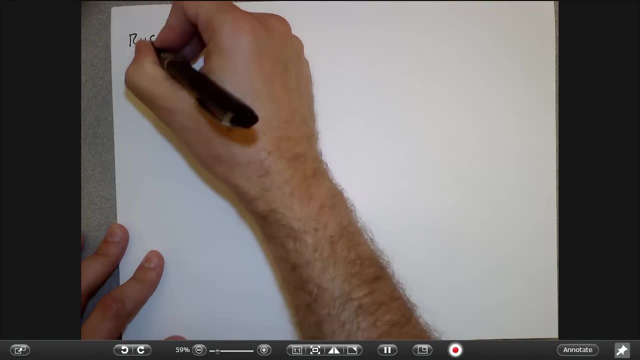 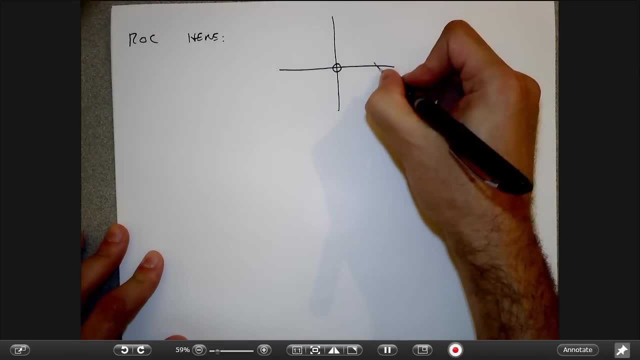 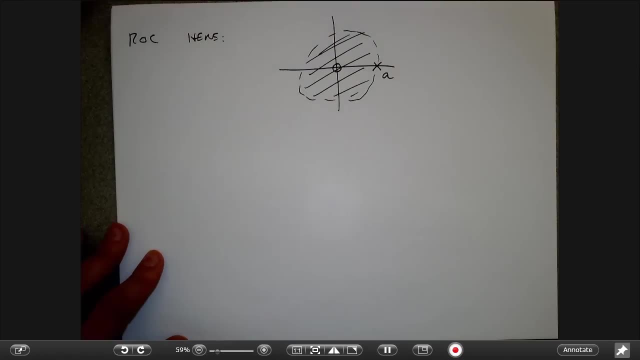 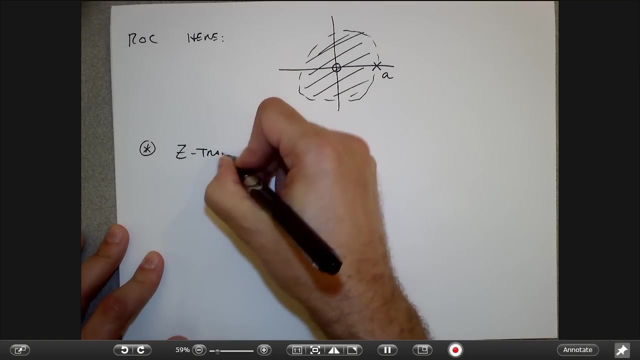 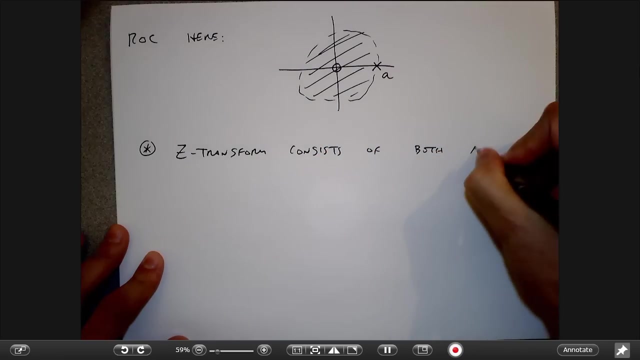 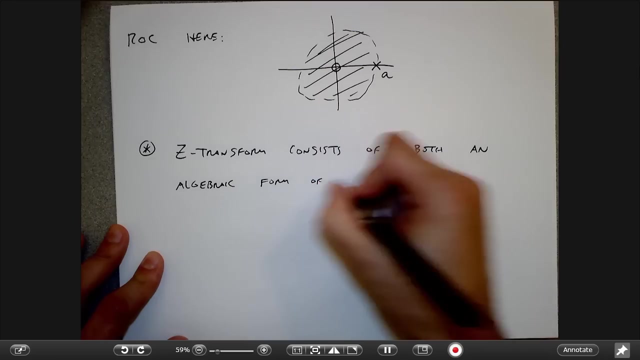 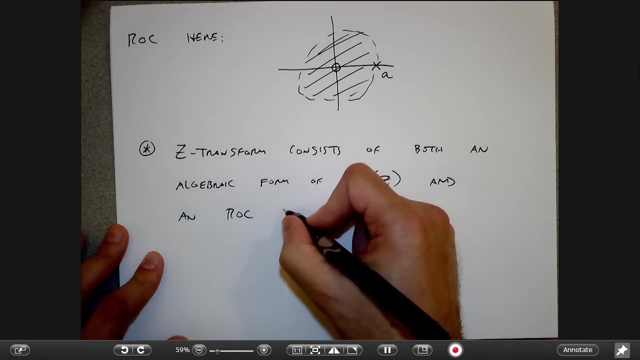 looks like. again I have a zero and a pole, and this time the ROC is inside this circle. So the key idea is that z transform is the same thing as the z transform. All right, consists of both an algebraic form of x, of z and an ROC region of convergence that says where this is valid. 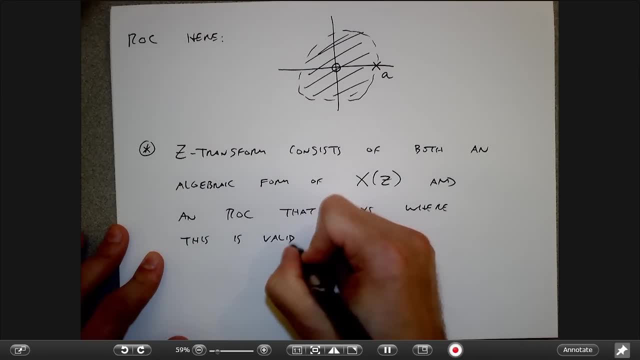 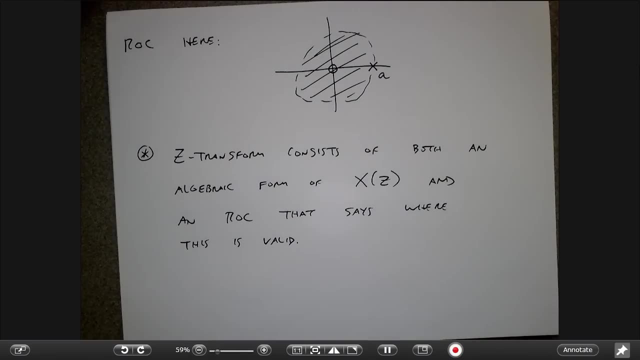 So the conclusion is that I can't just tell you: hey, the z-transform of a signal is blah. this function of z compute the inverse z-transform. The reason I can't do that is because I need to tell you what is the ROC in order to disambiguate which of the possible time domain signals I might mean. 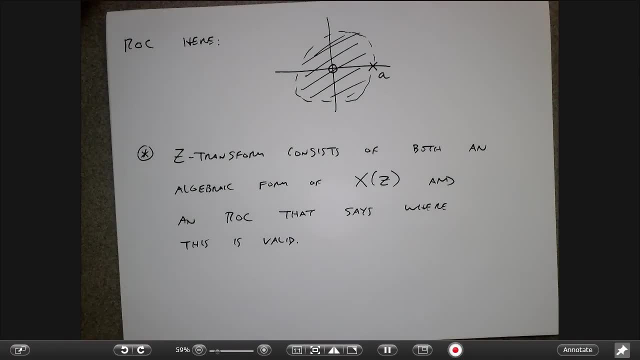 So that's why you always have to make sure that you note the ROC when you're working on a problem like this, otherwise it can get confused. Now it's fair to say that in a lot of the problems that we do, we're going to deal with right-sided signals. 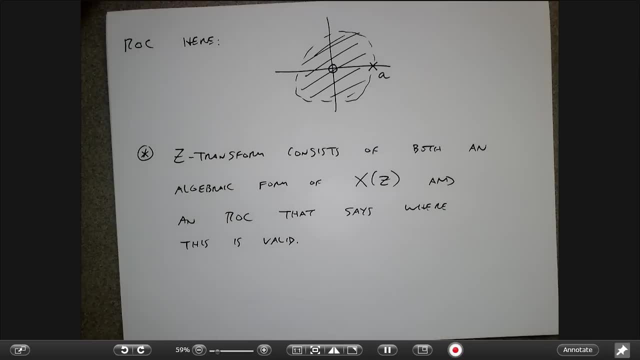 And so maybe what I may say in some future problems is something like: here is this function of z, and it's a right-sided signal, As you'll see, that pins down what the ROC is, And so that means I don't necessarily have to tell you exactly what the ROC is. 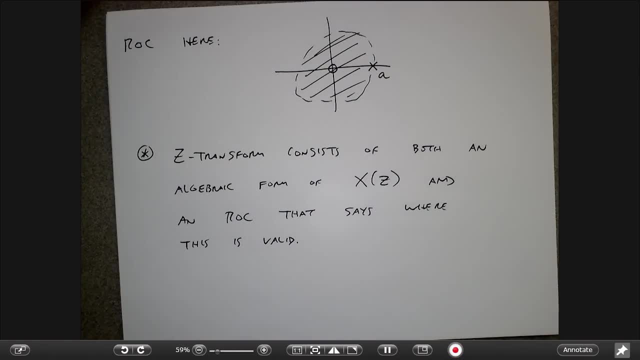 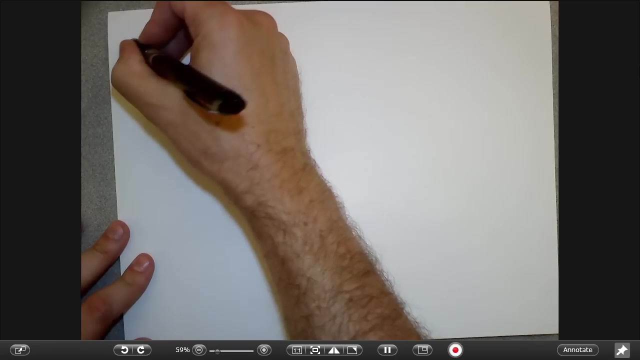 I just have to tell you: am I looking for a right-sided signal or a left-sided signal And that distinguishes between this and the sunburst pattern? Okay, So questions or comments. So let's do a little more complicated example. So here I'm going to kind of just use the linearity of the z-transform. 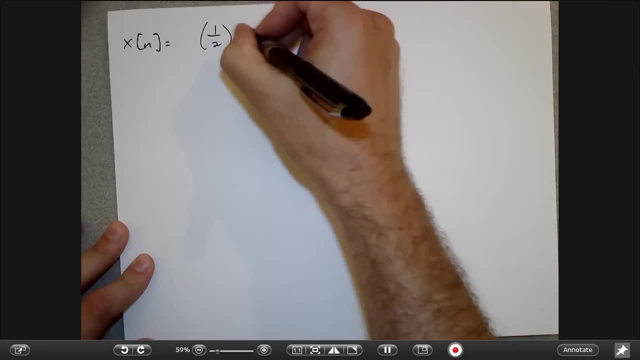 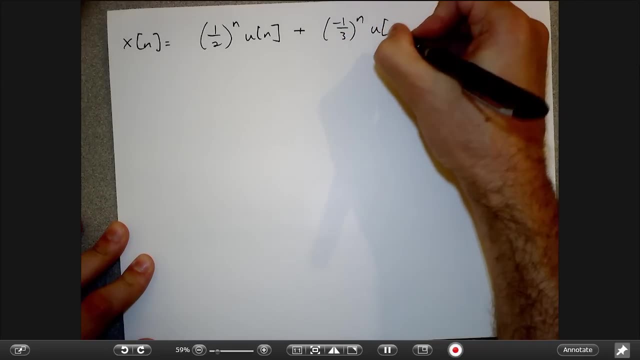 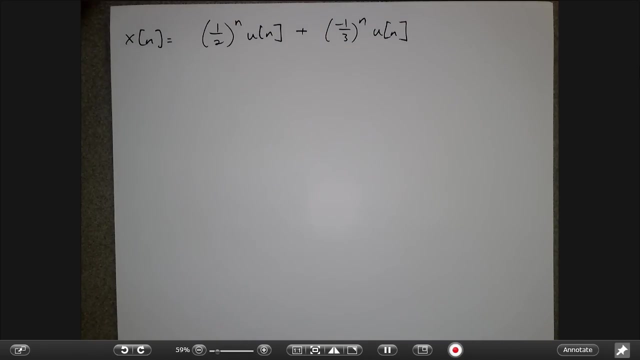 So here, let's suppose that I have this signal, Okay, And so again, just like with the Fourier transforms, after you've kind of learned what a property is, I'm going to allow you to use it. You know, this is not about just grinding through. you know algebra. 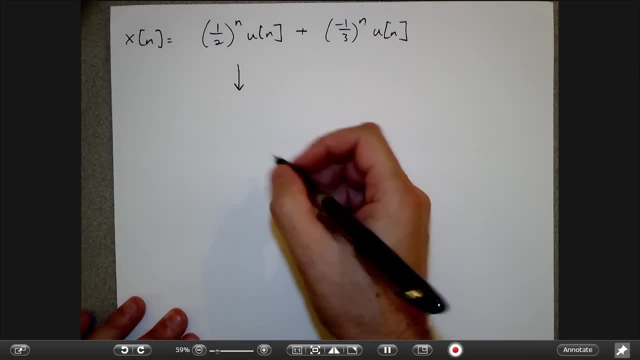 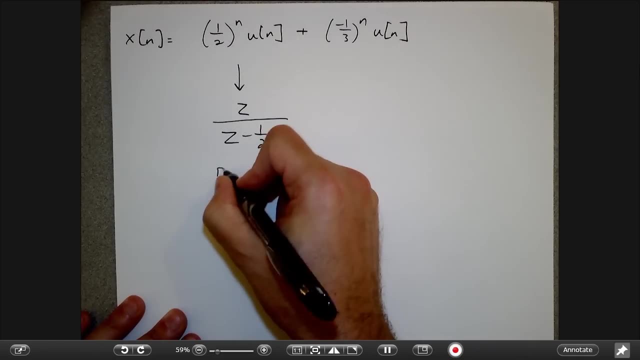 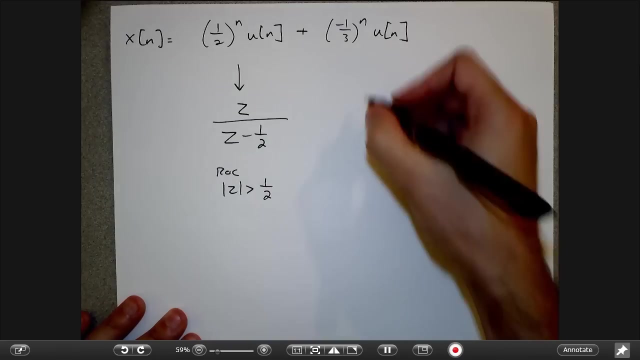 So here we can immediately conclude that this signal has a z-transform of z over z minus a half, with the ROC being the absolute value of z greater than a half. right, That's kind of what we've learned just before This guy has the. 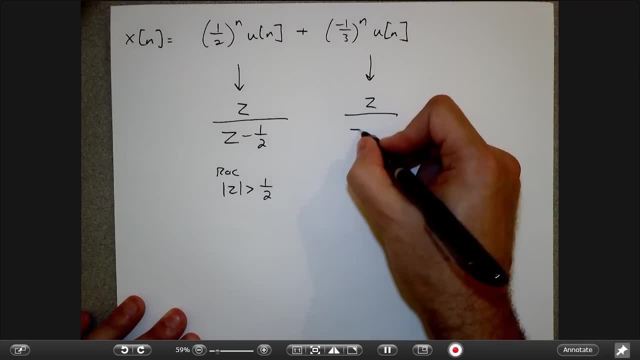 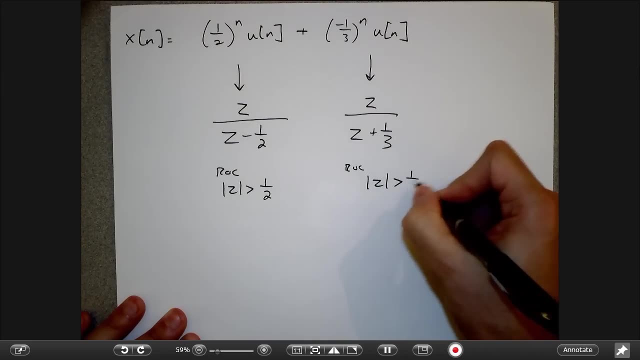 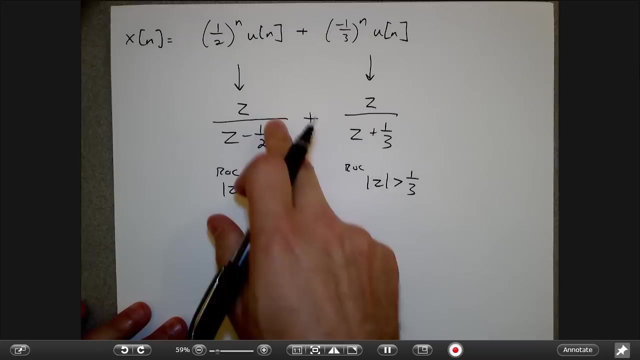 This is the ROC, z over z plus a third, And the ROC here is going to be z greater than a third. Okay, And so now I have to think about: okay, well, the z-transform is going to be the sum of these things, whatever it is. 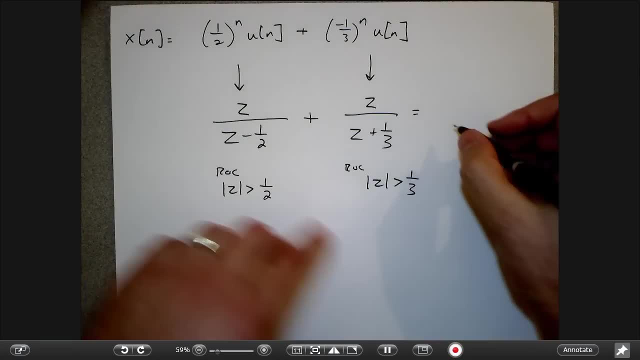 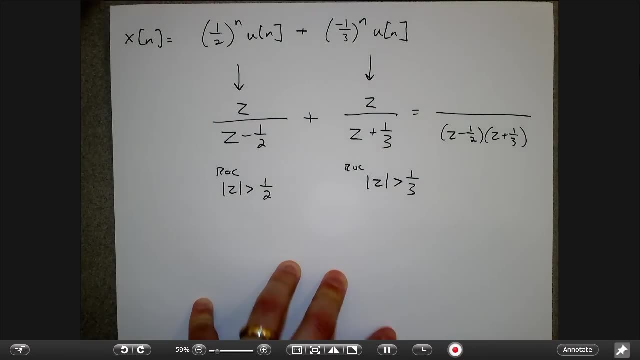 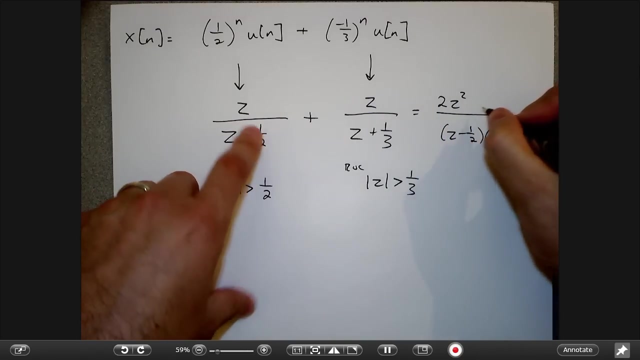 And so I can just kind of compute stuff out. I'm going to get a z minus a half over a z, plus a third in the denominator And in the numerator. I'm going to get whatever this turns out to be. So I guess I'm going to get a 2z squared minus a half of z, plus a third of z is going to be minus a sixth of z. 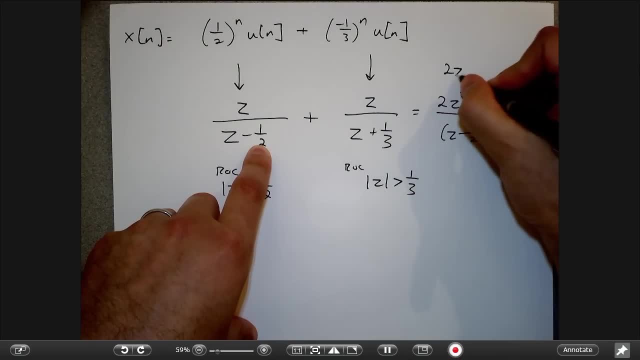 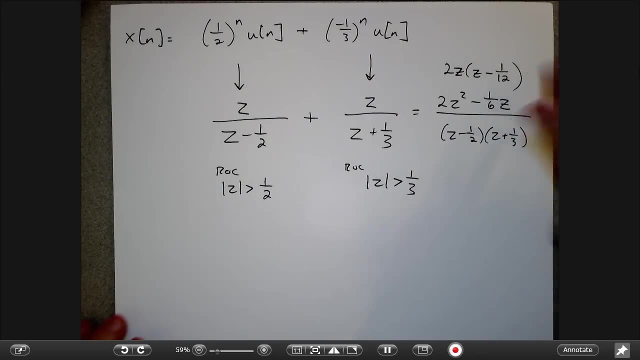 And so if I factor out the z, I get 2z z minus 1 twelfth. So I figured out what the you know, I figured out what the algebraic form is. Now, what is the ROC Right? So for the ROC I need to have both of these things existing at the same time, right or in the same place. 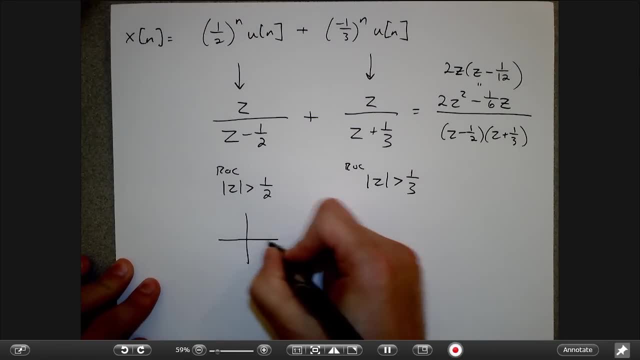 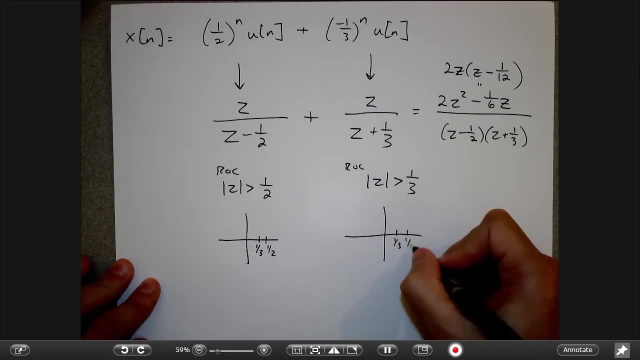 So I have to draw my two ROCs, right? I have if this is a third and this is a half, right? So one of the ROCs looks like this And one of the ROCs looks like this, Okay, Okay. 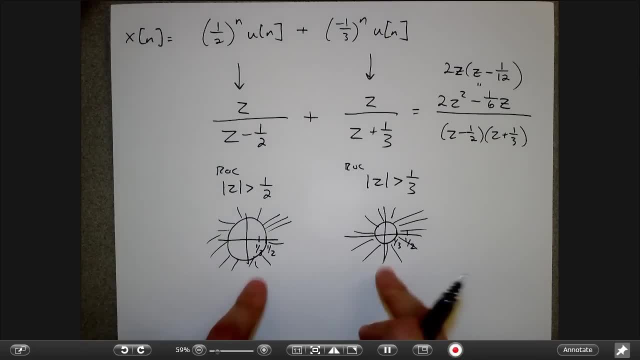 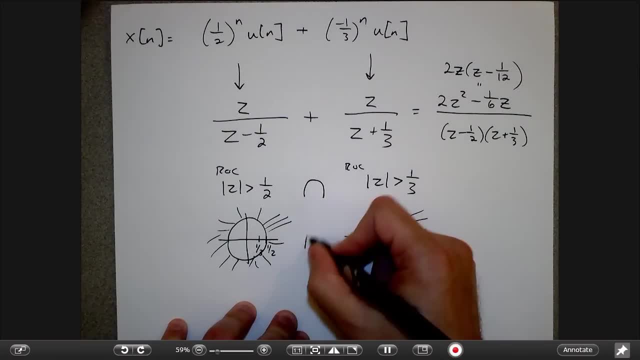 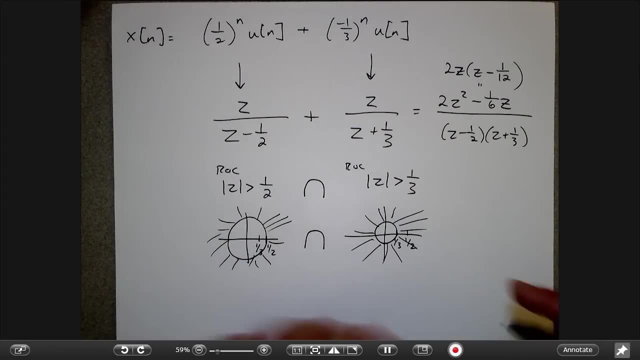 I'm sorry. I look at the intersection of these two things. These things both have to happen at the same time And so, looking at this, this guy over here is the one that's more restrictive, right? So the final ROC looks like a starburst that's outside of a half. 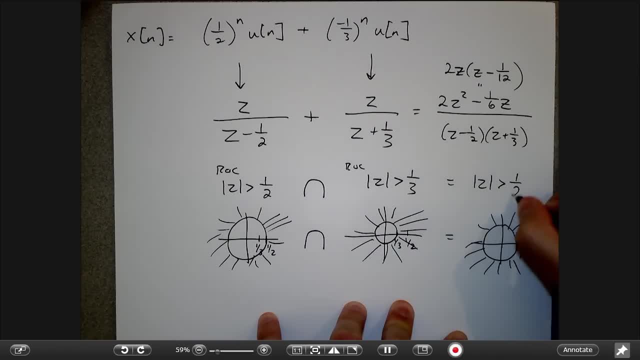 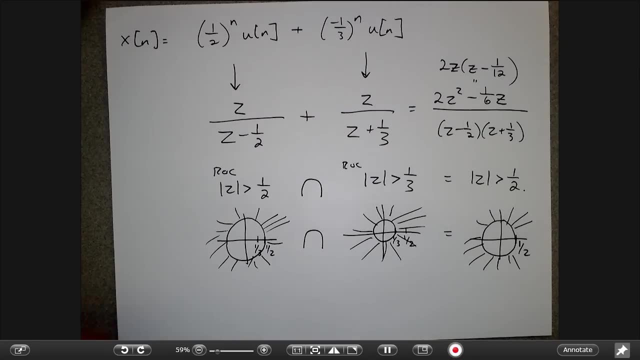 And this intersection is this guy. Okay, And so again, if I were to draw the pole zero diagram, what I would get would be the following: So I guess I didn't leave myself that much space, but I guess I could try and do it over. 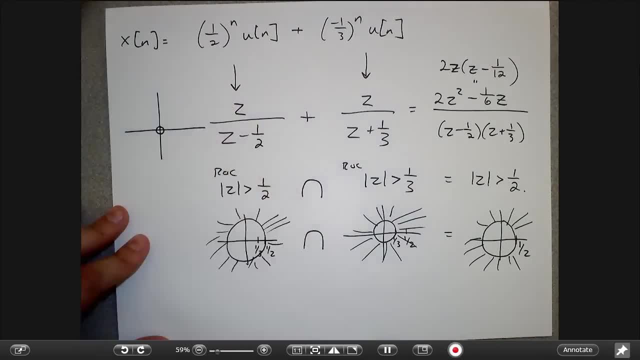 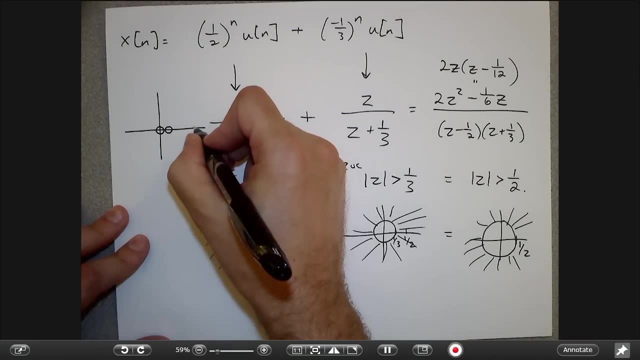 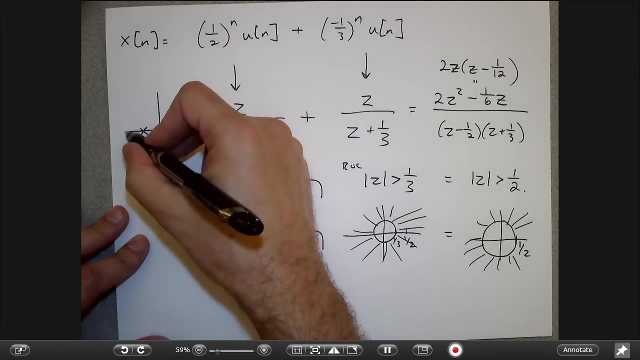 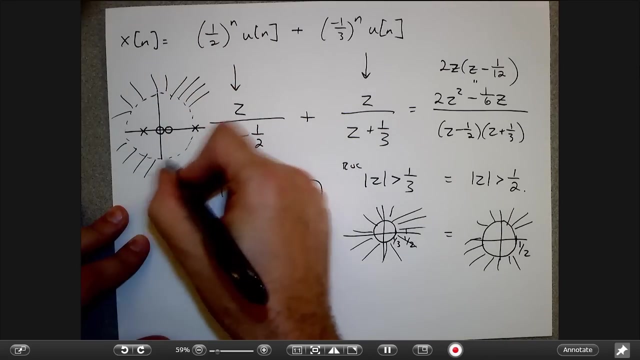 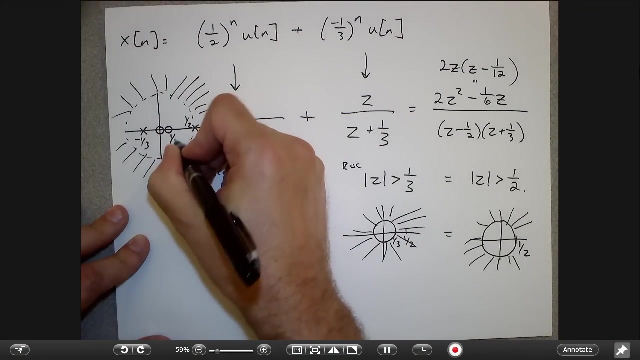 here. So I have a zero over here at zero, I have a zero at 1 twelfth, I have a pole at a half and I have a pole at minus a third, And then my ROC looks like a circle that extends out from a half. 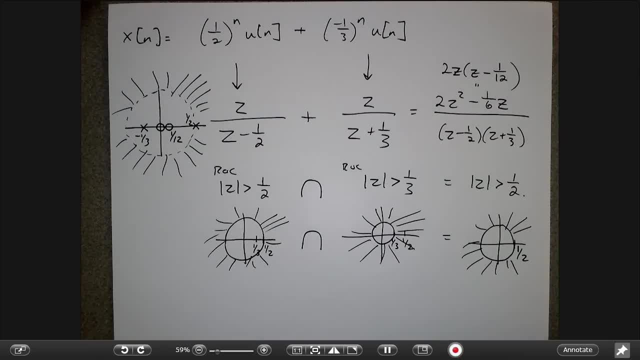 And so, as you can see here, Um, You know, somehow the ROC is related to the poles, right, And we're going to see that more generally. So the zeros don't really play any role in what the ROC could be, but the poles are what. 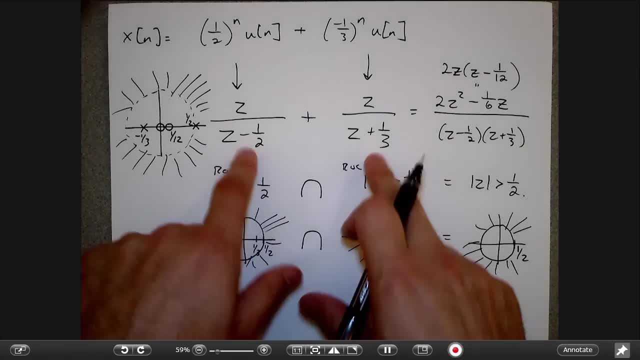 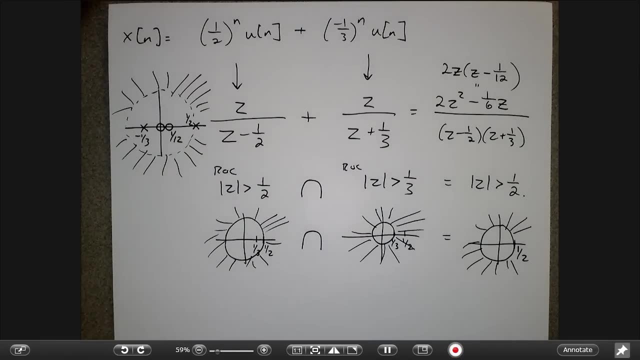 play a huge role. right, Because I need to look at the things that involve the denominator And just to illustrate the point that, again, just as I had in the previous example, a right sided thing and a left sided thing that gave me the same algebraic form of z, but different. 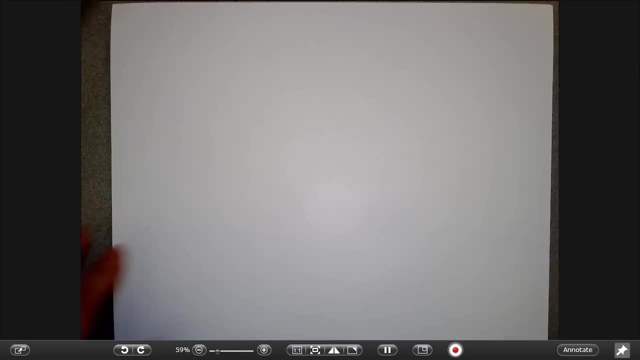 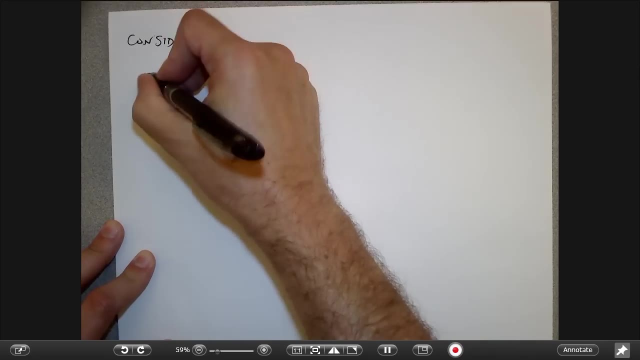 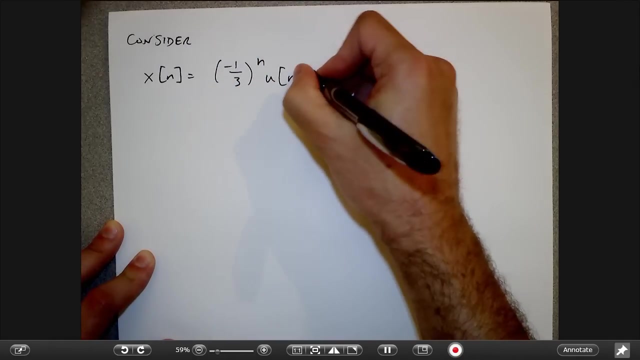 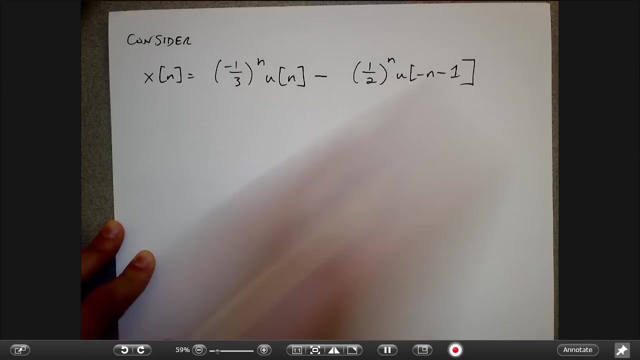 z transforms, I can consider a signal that also does the same thing here. So I'm not going to work out all the algebra, but if I consider this signal, this signal kind of has a part that is right sided and it has a part that is left sided. 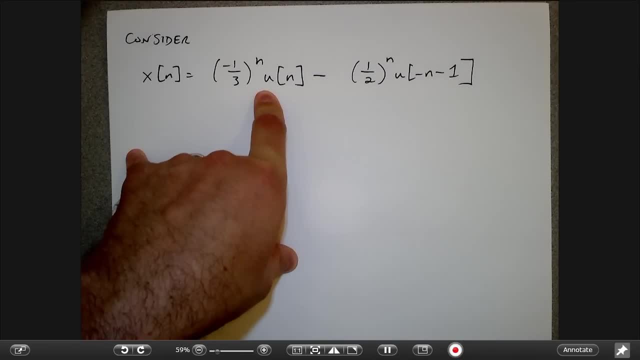 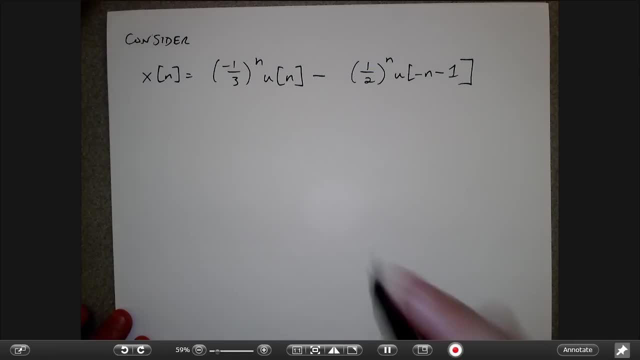 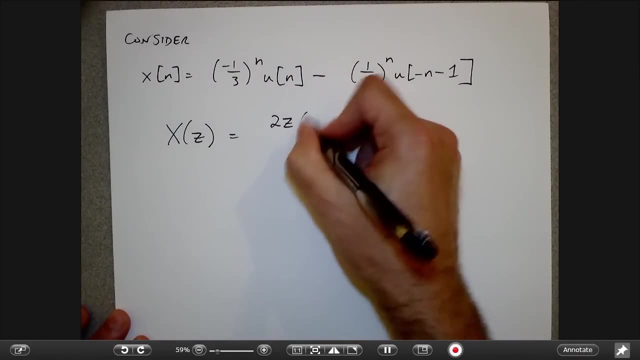 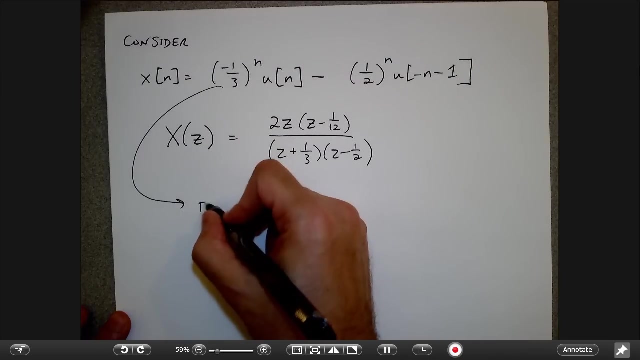 Or greater than or equal to zero. This covers what's happening when n is less than zero, And it turns out that I can work this out to the very same algebraic version. The ROC is different, right? because the ROC for this guy is again the absolute value. 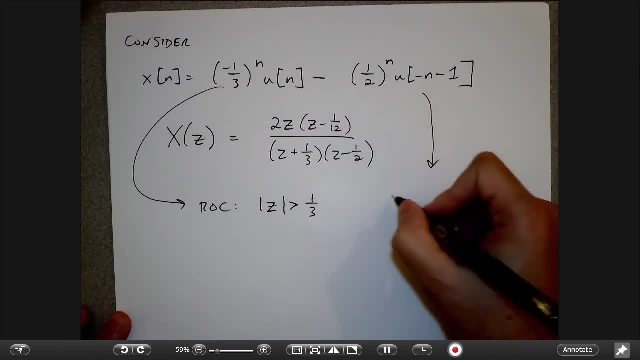 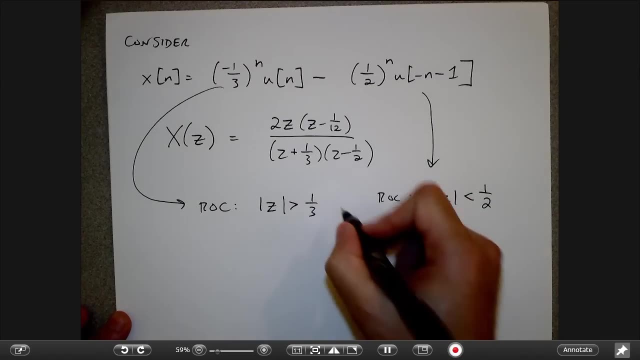 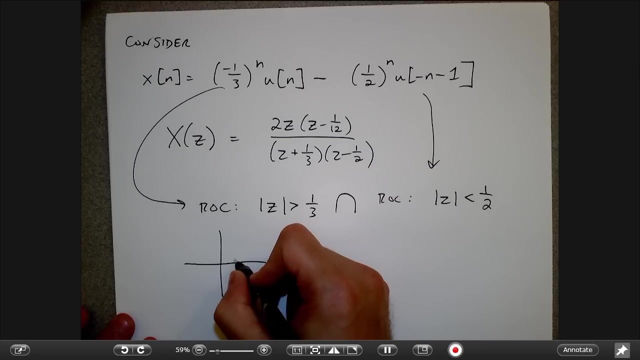 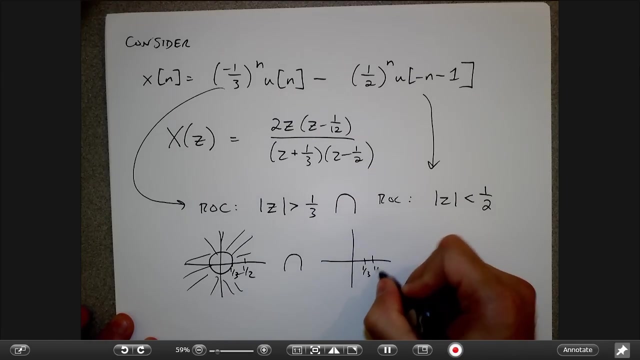 of z greater than n a third. the ROC for this guy is the absolute value of Z less than a half, And I have to look at the intersection of those things. So here, one of the ROCs looks like this and the other ROC looks like this. 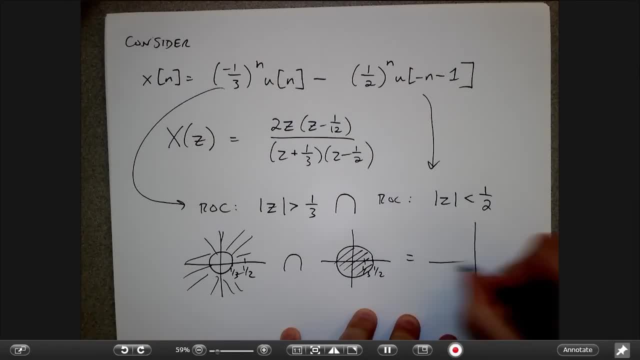 And so if I look at the intersection between those two guys, then I get this kind of a ring where I have a third and a half And the intersection of those two things is all the stuff that's inside this ring shape. And so again, even though I have very much the same pole zero diagram here, I get a very 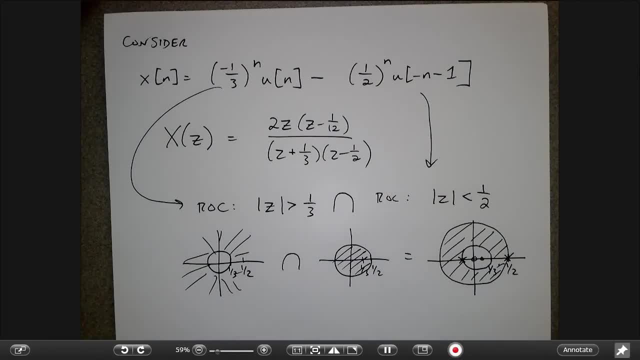 different ROC And in fact, if I wanted to, I could consider a purely left-handed signal that had again the same algebraic thing and the same pole, zero plot. but the ROC would be basically zero, It would be just inside this circle here. 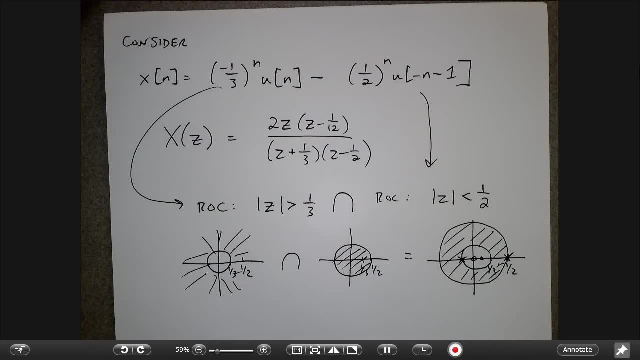 So, fundamentally, there are actually three possibilities for valid Z transforms that have the same pole: zero plot. So, like I said, I'm not going to drive you crazy with lots of left-handed and double-sided signals. I mean, most of the stuff we do in this class is still going to be assuming that things. 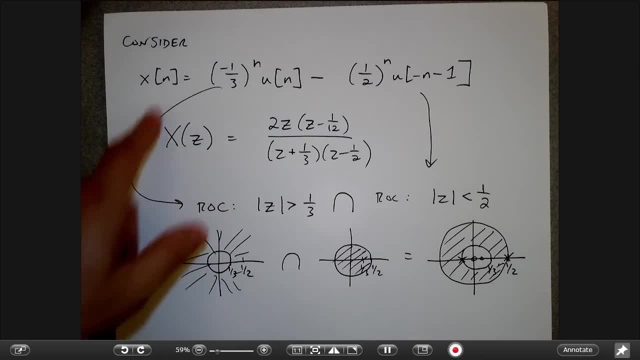 start at zero, And one of the reasons for that is that, again, most of the time the signals that we care about are impulse responses, And for impulse responses, I don't want impulse responses to correspond to causal systems. I have signals that are right-sided. 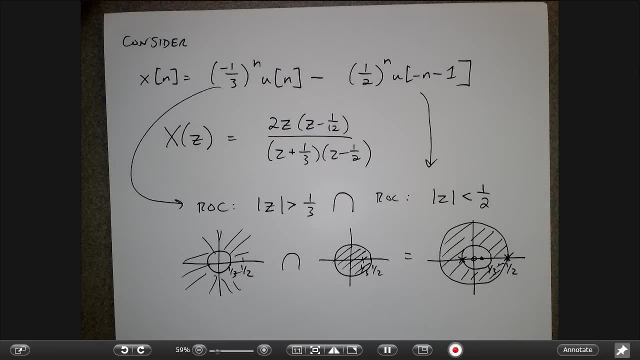 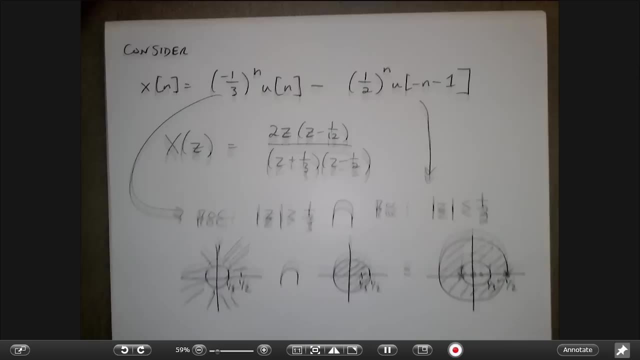 I don't want to have impulse responses for which H of n is non-zero, for values of n less than zero. So I kind of want to make sure that my impulse responses are all right-sided. That means that I'm going to get nice kind of ROCs that are always like these sunbursts. 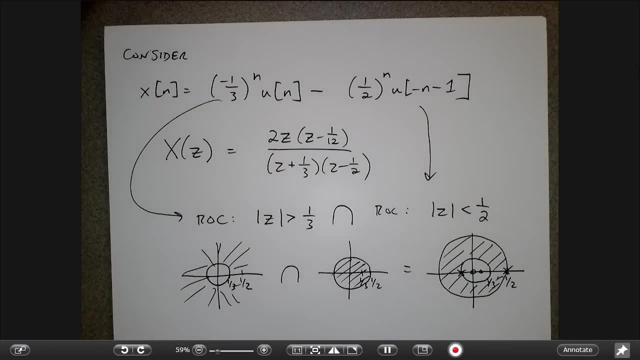 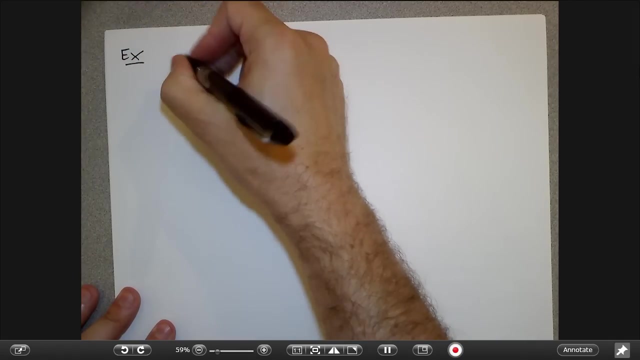 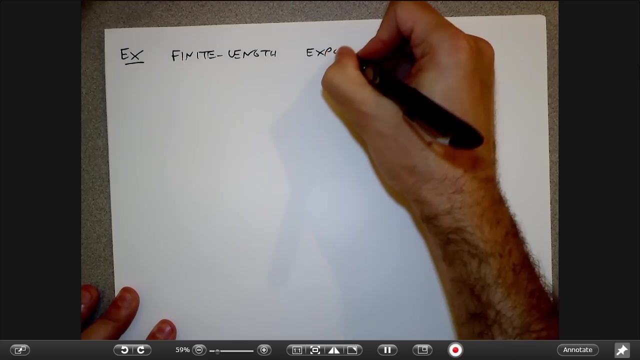 going out, Okay. So comments or questions? Okay, All right. So let's do a slightly trickier one. So what if we have a finite length exponential? So everything I've done so far has been some signal that extends to infinity in one direction. 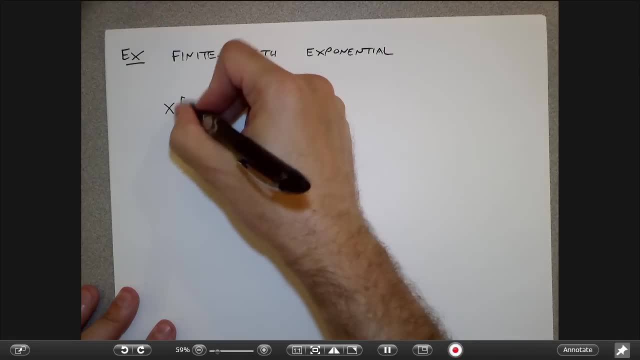 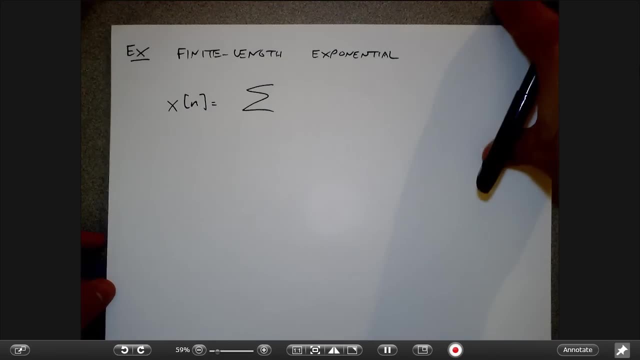 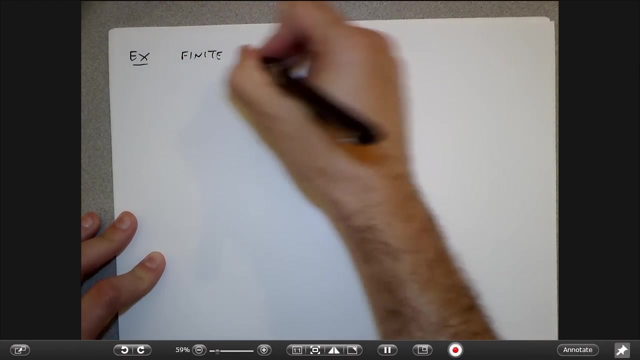 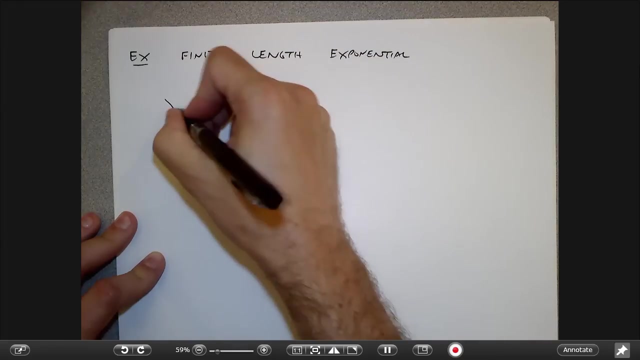 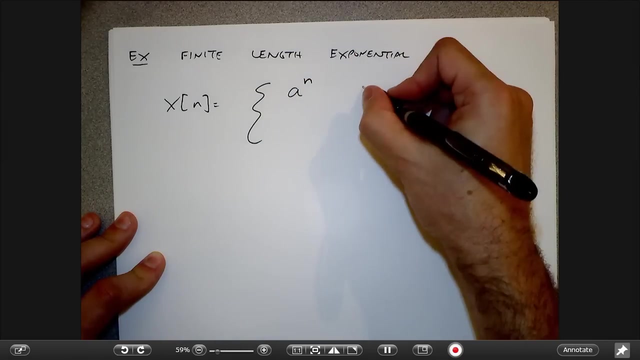 or the other, or both, But what about something like this? So here, Oops, Sorry, Okay, Let me just redo this picture here. So here, what I wanted to do was something like this: This equals a to the n for n within this range. 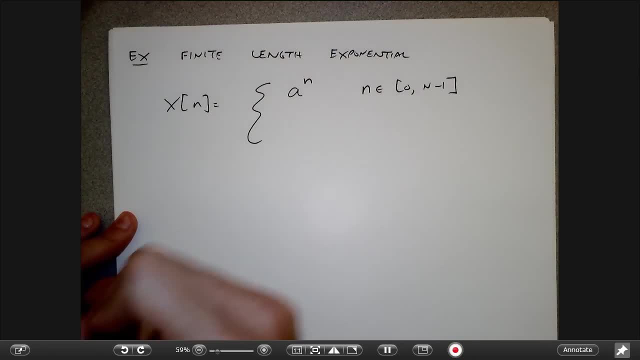 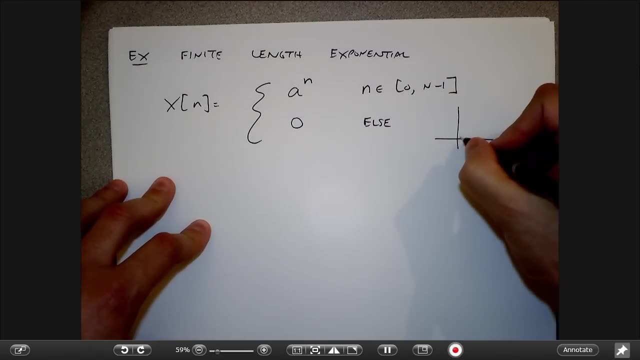 And zero otherwise. So this is a to the n for n within this range And zero otherwise. So this is a to the n for n within this range, And zero otherwise, And zero otherwise. So what that looks like is just something that turns on at zero. 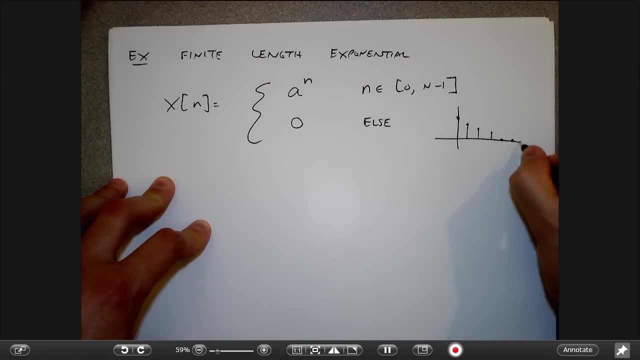 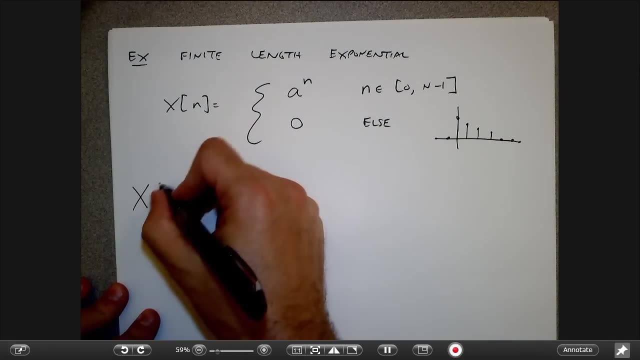 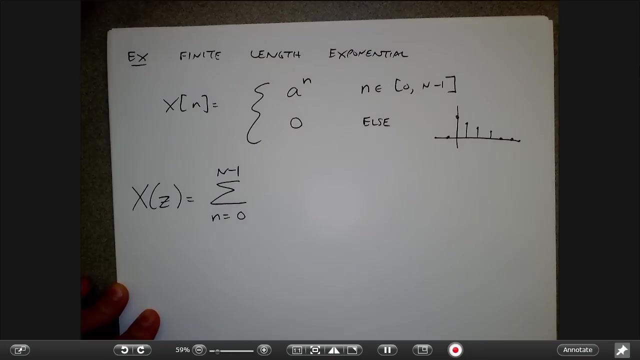 It exponentiates for a while and then it turns off at some point, and then zero afterwards. So this is only a finite number of non-zero elements. And so what is my x of z going to be? Well, I'm going to have this guy: a to the n, z to the n. 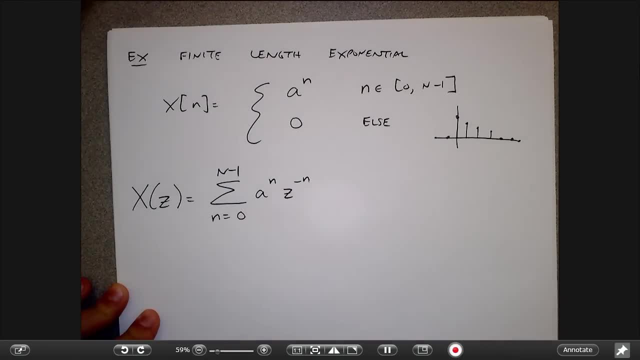 Or z to the n. I'm going to have this guy a to the n, z to the n Or z to the n. Okay, So I'm going to have this guy a to the n, z to the n. 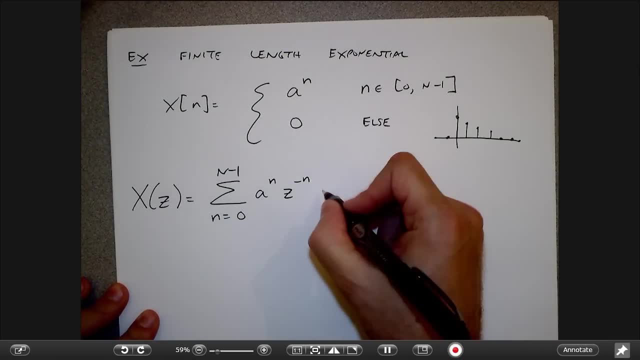 Okay, So I'm going to have this guy a to the n? z to the n. Okay, So I'm going to have this guy a to the n, z to the n. So here I kind of just noticed that this sum can only be non-zero in these places. 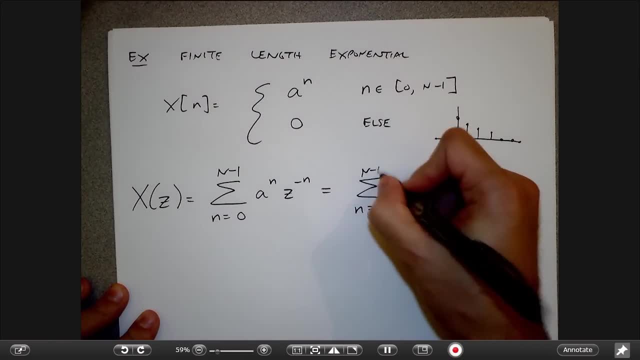 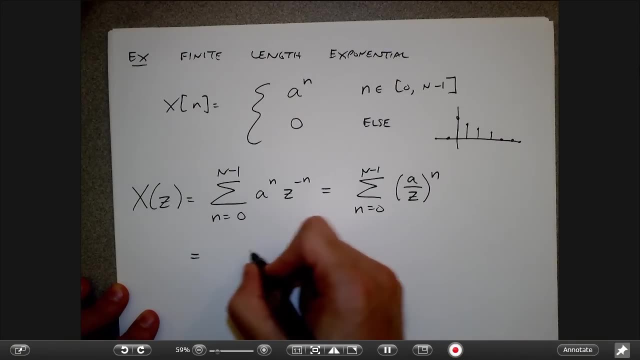 And again this kind of looks similar to what I had before, except now I'm going to say: well, I can write the answer, which is going to be 1 minus this thing, to the n power over 1 minus this thing. 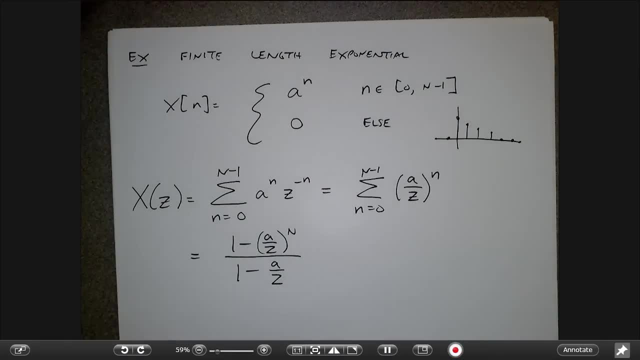 This is going to be true, no matter the value of a Right. The reason is that the finite sum formula is valid. this formula is valid no matter what the value of this is, because there's only a finite number of terms in the sum. 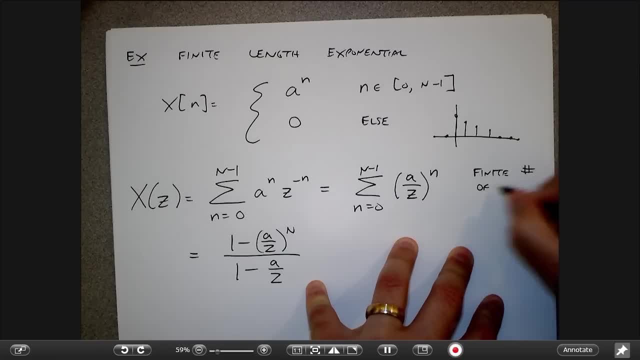 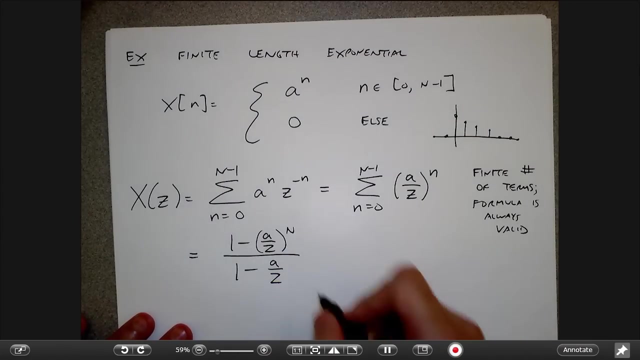 So there's only a finite number of terms. the formula is always valid, And so if I kind of multiply everything through by a z to the n power, what I can get here is I have z to the n minus a to the n over, z to the n minus a, z to the n minus 1.. 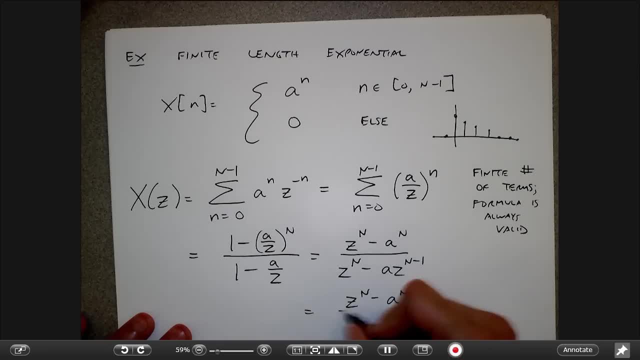 Which is a different way of saying z to the n minus a, to the n over, z to the n minus 1, z minus 1.. And so here I would take a look at this and say, okay, well, again now I have a polynomial. 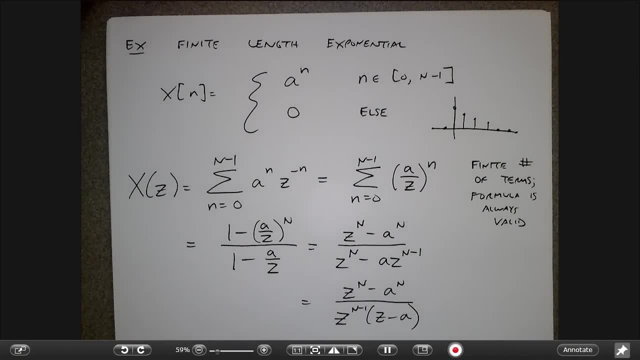 in z over a polynomial in z. So I'm going to have capital N zeros, which are the zeros of this top polynomial, and capital N zeros, which are the zeros of this bottom polynomial. So my pole zero plot is going to be a little more complicated. 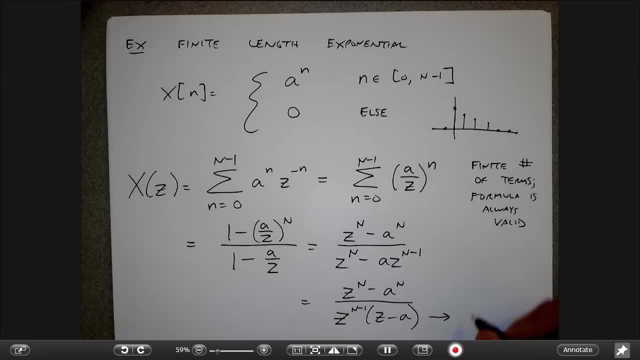 So I have to ask myself: okay, I'm going to get- let's look at the poles first- So I'm going to get n minus 1 poles And I'm going to get a pole at z equals 0, right? 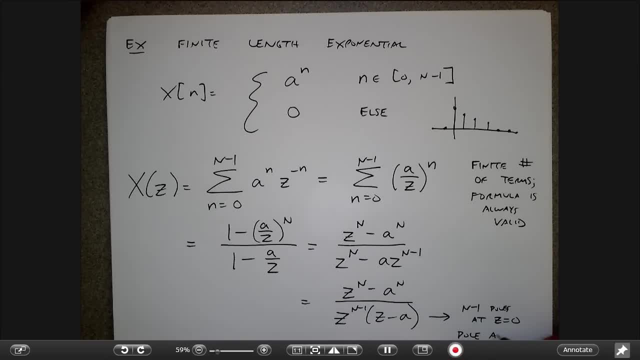 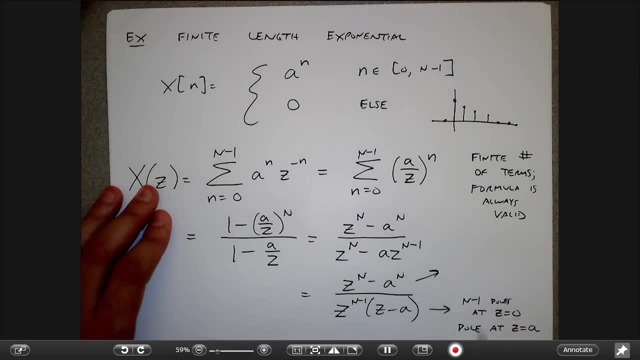 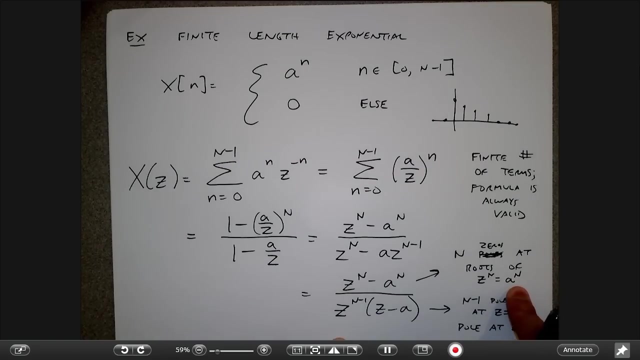 A conjugate for this And I'm going to get a pole at z equals a, And here I'm going to get n poles, I'm sorry, n zeros at the complex roots right. So here I've got a complex number to the n power equals this number here. 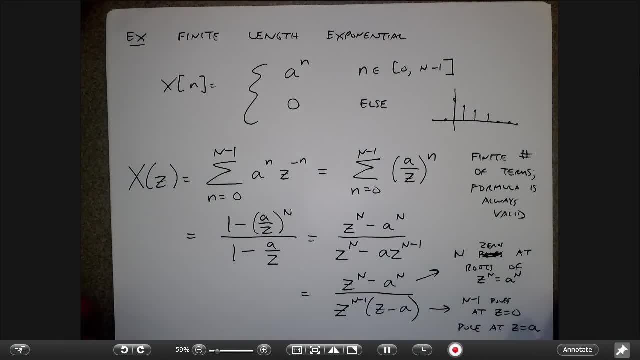 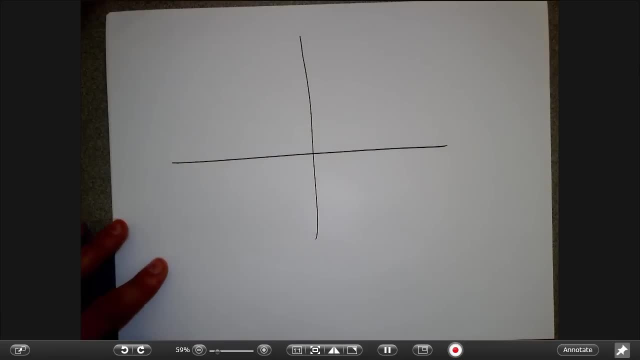 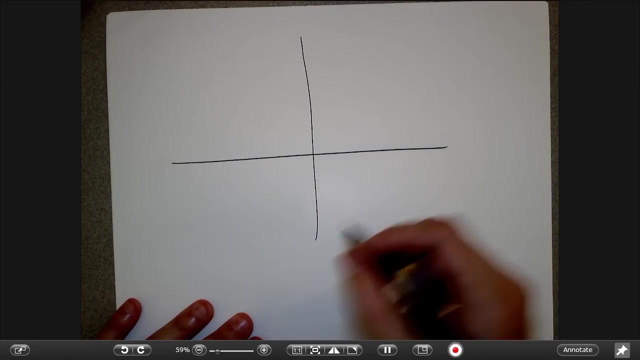 And so this may be something that is not familiar to you, but you know, the nth roots of some number are generally distributed around the circle like so. So here um say I have n roots, so say I have n equals 8.. 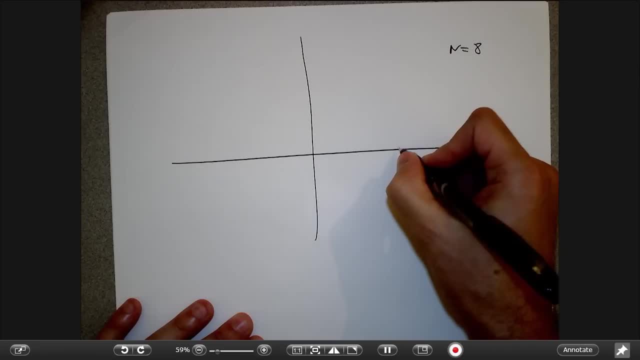 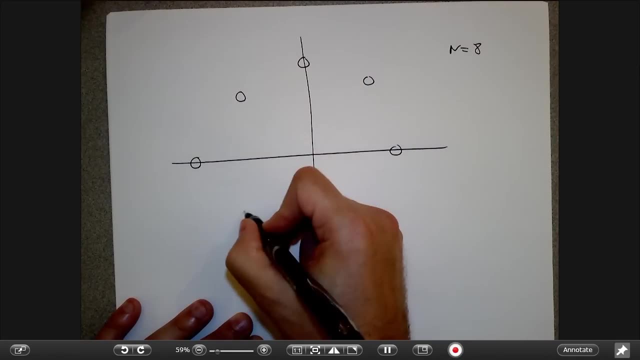 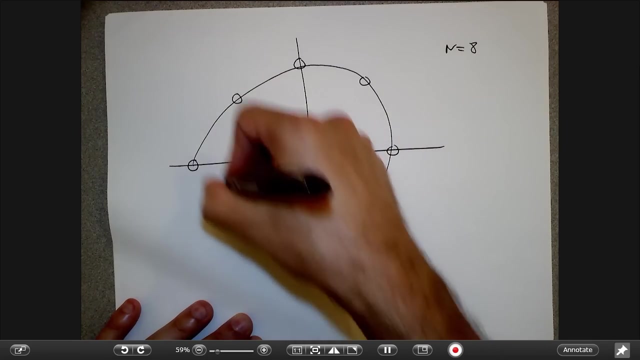 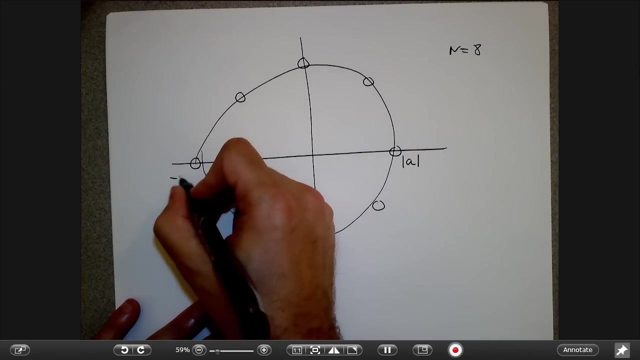 What that means is that I'm going to have a pattern of things that look like this, Kind of evenly spaced around the circle. This is going to be like um, absolute value of a. This is going to be a minus a. This is going to be the absolute value of a j. 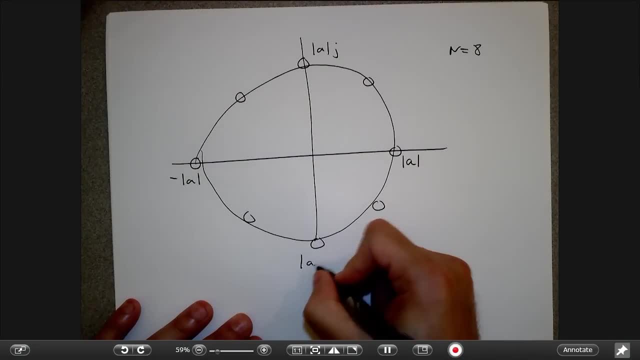 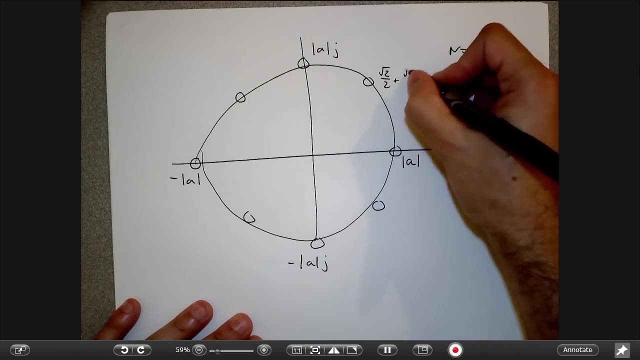 This is going to be minus the absolute value of a, j, And these guys are going to be, like you know, square root of 2 over 2, plus square root of 2 over 2, j times the absolute value of a. 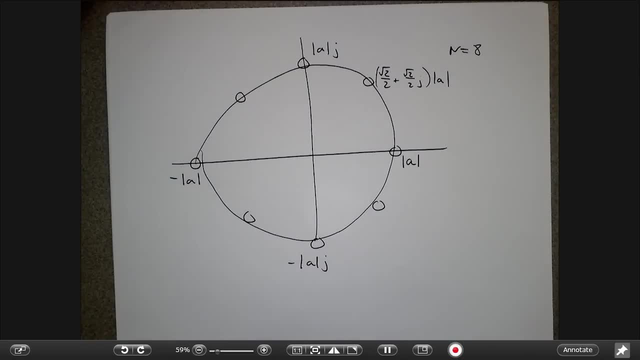 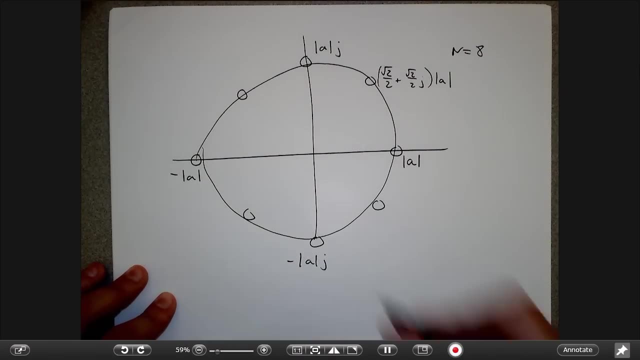 So it's just they're going to be 8 complex numbers that give me the zeros of that top polynomial That are generally evenly spaced around the circle, And then my poles. I'm going to have basically a whole bunch of poles at 0.. 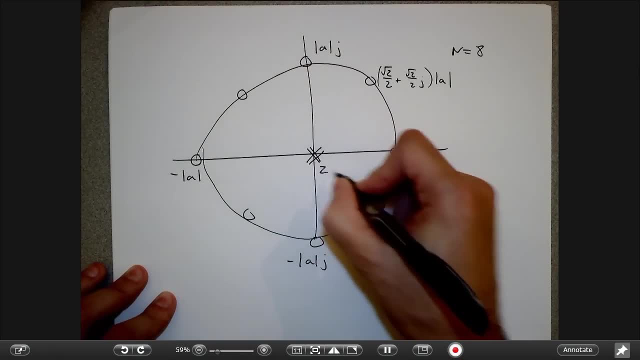 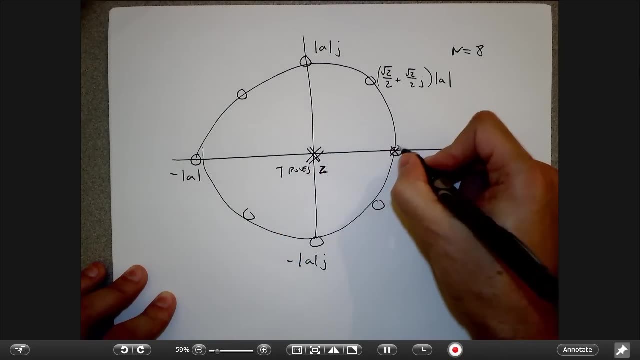 And then I'm going to have a whole bunch of poles at 0.. I'm going to have, um, let's say, 7 poles If n equals 8.. And I'm going to get a pole, as we talked about, at z equals a. 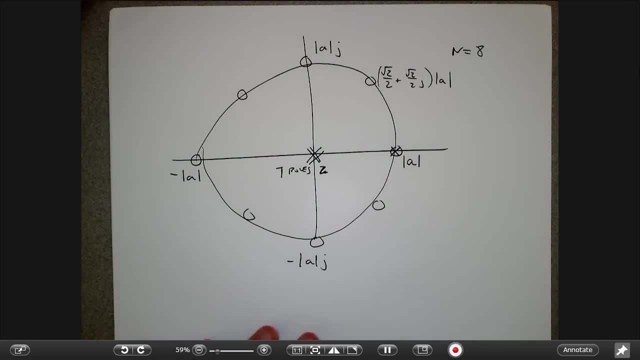 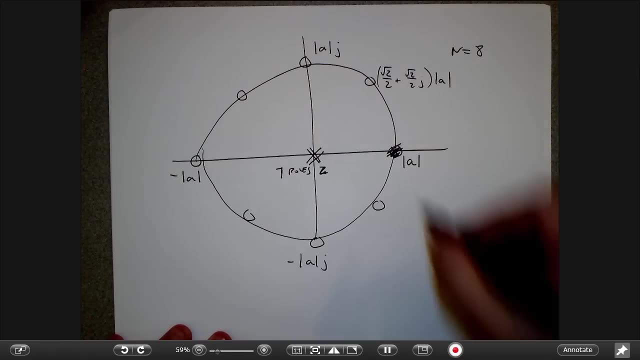 Right, I have this extra pole here, And so here I see that this location has both a pole and a 0 on it, And so these things are basically going to cancel each other out, Right? So there's not going to be a 0 here or a pole here. 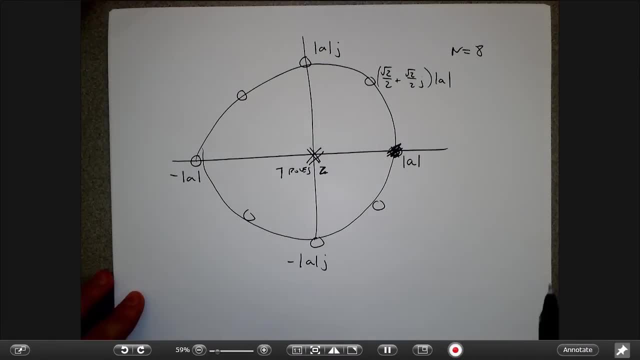 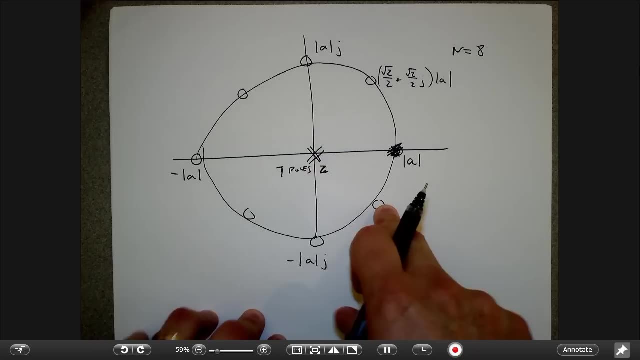 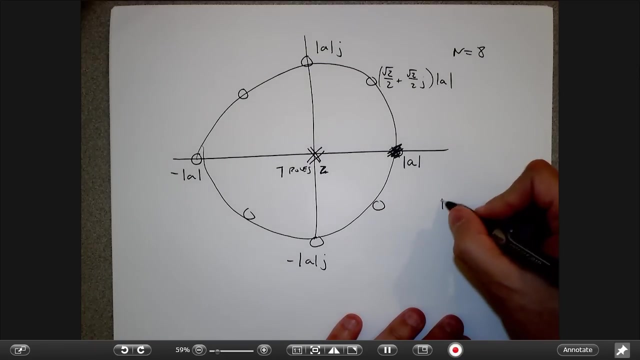 Because the numerator and the denominator both kind of cancel each other out, Those terms vanish, And so actually what I have is 7 poles at the origin And 7 zeros scattered around the complex plane, And one thing to observe here is that, you know, the ROC is any value of z that is not 0.. 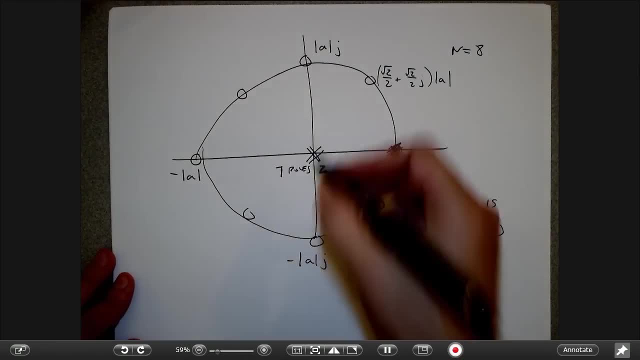 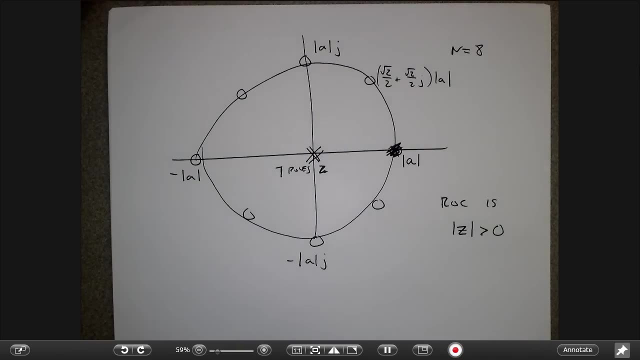 Right, And so that means that fundamentally any value of z I can look at the z transform for this signal, And so this is generally true when my input signal is only finite length, Right. So the problems come in when the input signal is infinitely long. 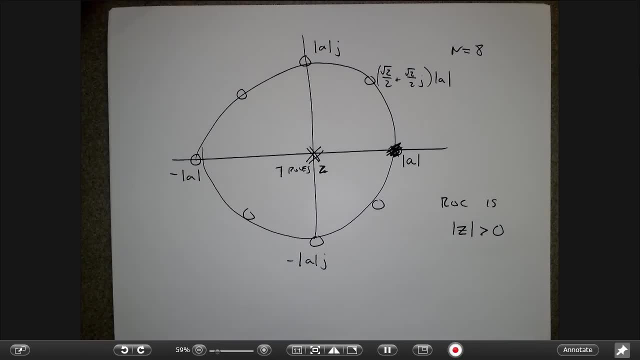 In that case I have to think about things like convergence and sums. But the intuition is that if I have only a finite number of terms to add up, nothing can ever go wrong unless I'm adding up kind of infinity plus infinity all the way through. 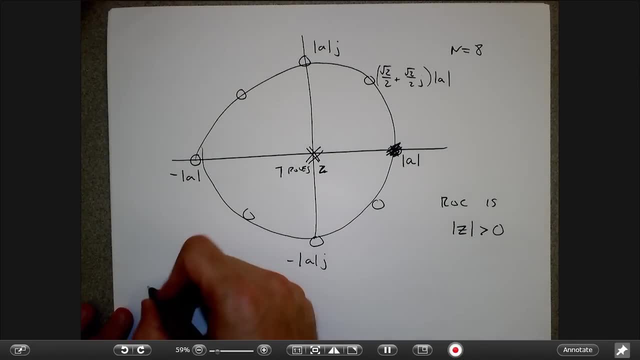 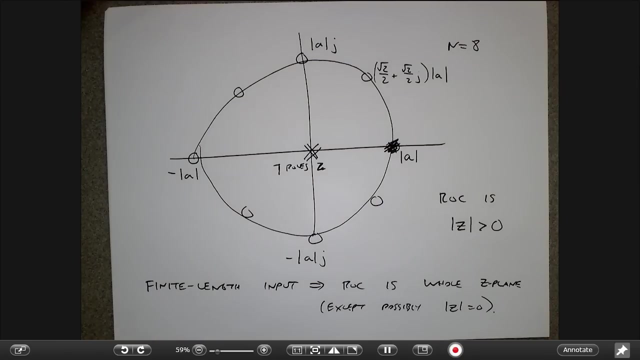 Right. So here this is an illustration of, you know, finite length input, And if I have this infinity, that means that ROC is the whole z plane, except possibly z equals 0.. So in some sense, when I have a finite length input or a finite length impulse, response. 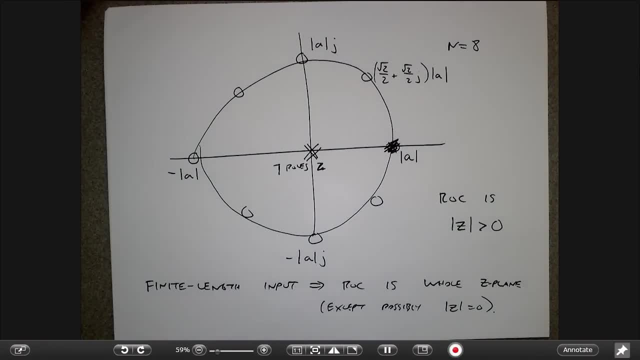 life is always pretty good, Right? There is no need to worry about poles, because all the poles are clustered together- clustered together. so we're going to talk more about pole zero patterns in later lectures. Comments or questions about this example? Let's make it a little more complicated. What? 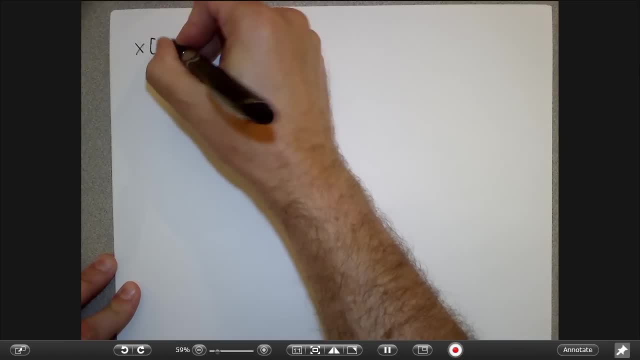 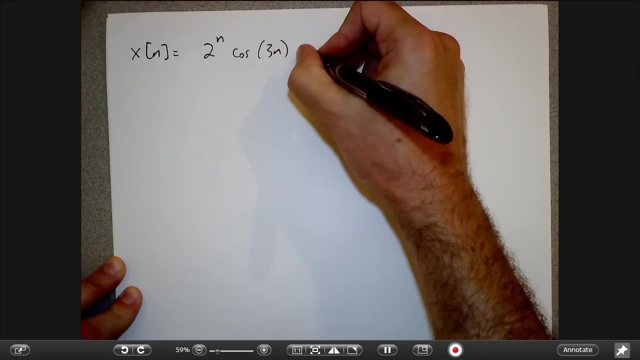 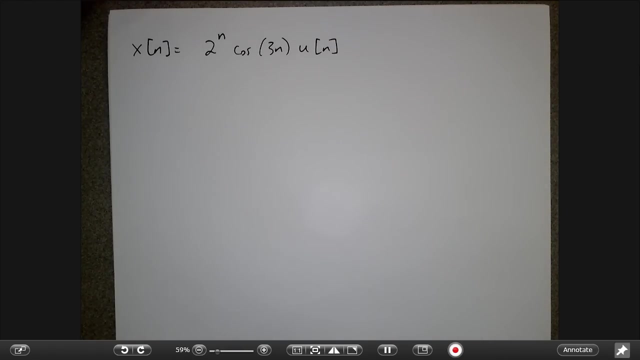 about this: signal 2 of the n cosine 3m u of n. This looks a little more complicated but again, the first step is always to remember that whenever you see a cosine or a sine, you can turn it into an exponential, because a cosine is like the sum of two exponentials. 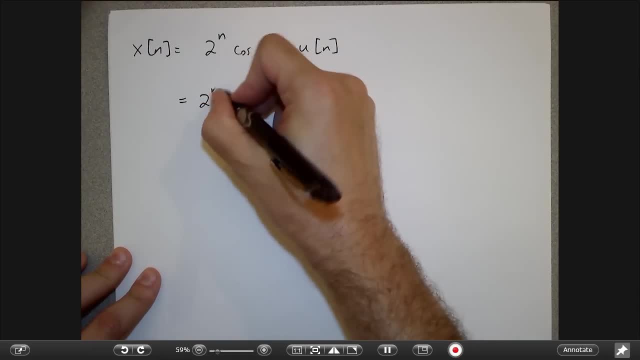 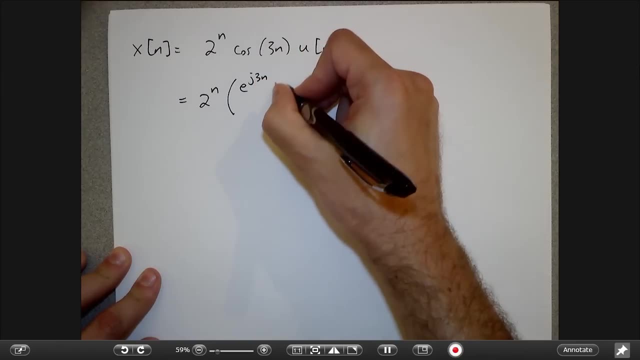 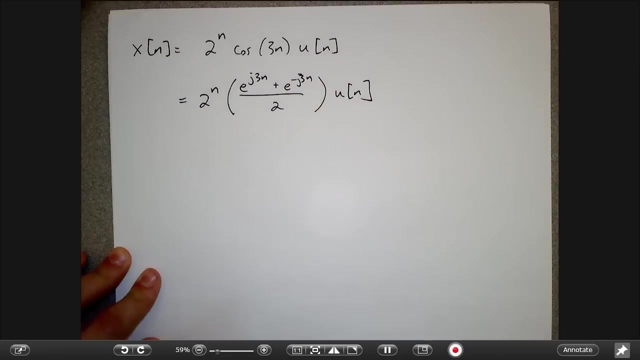 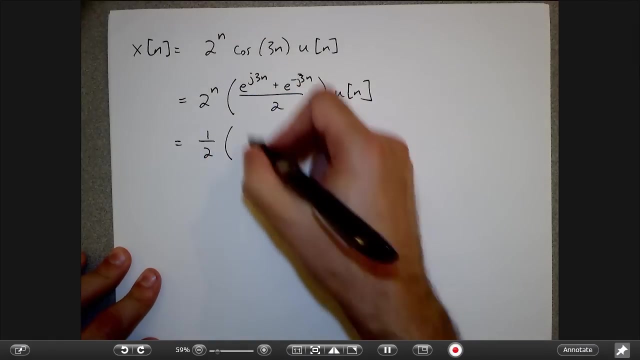 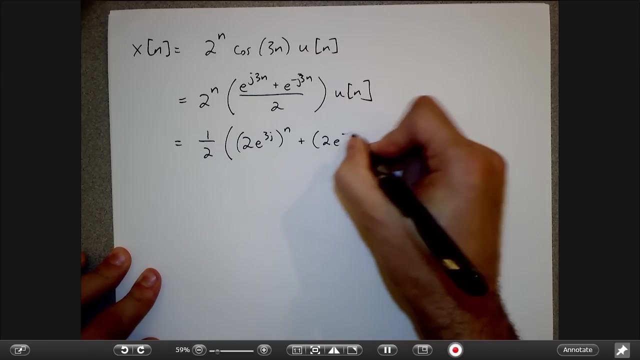 over two. I can immediately say this is like 2 of the n? e to the j, 3m plus e to the minus j, 3m over 2? u of n. I can immediately say this is like one half times 2. e to the 3j to the n plus 2 e to the minus 3j times 2? e to the? 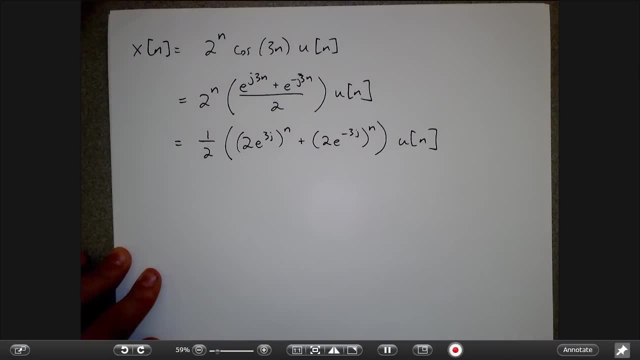 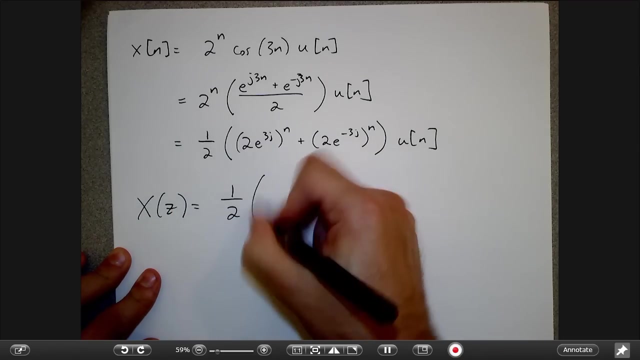 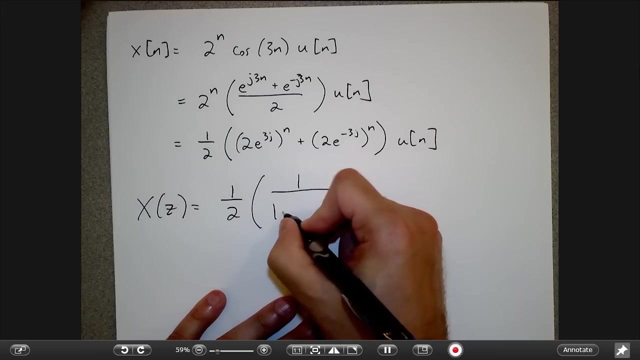 minus 3j to the n. And now each of these terms is in the form of something to the n times, a step function, which I already did in the previous problem. So my x of z, I can immediately conclude, is 1 half times. well, what was my formula? It was like saying 1 over 1 minus 2 e to the 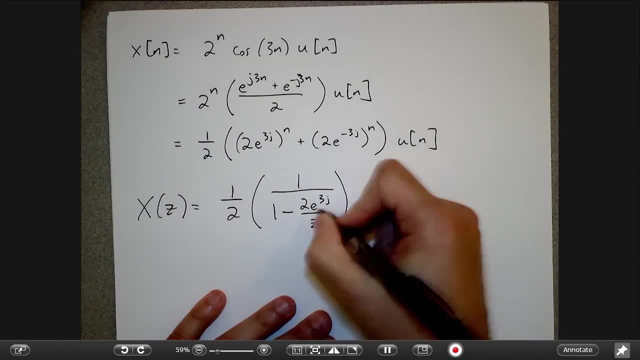 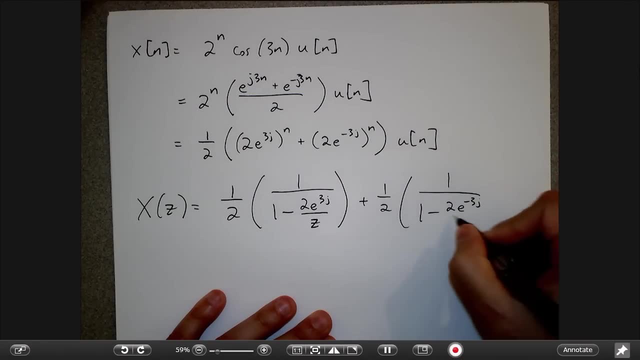 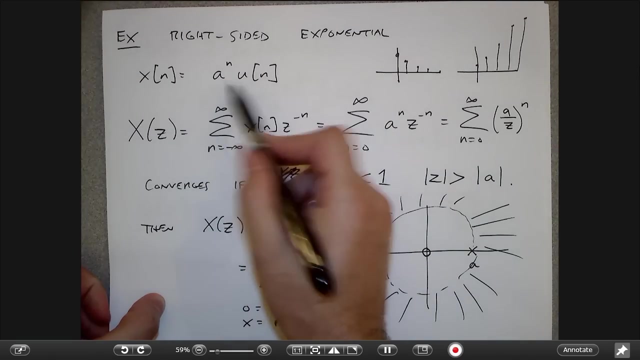 3j over z? Oops, plus 1 half 1 over 1 minus 2. e to the minus 3j over z? Right, all I'm doing is applying This formula right here, right, So I've got a to the n? u of n. Nothing here says that. 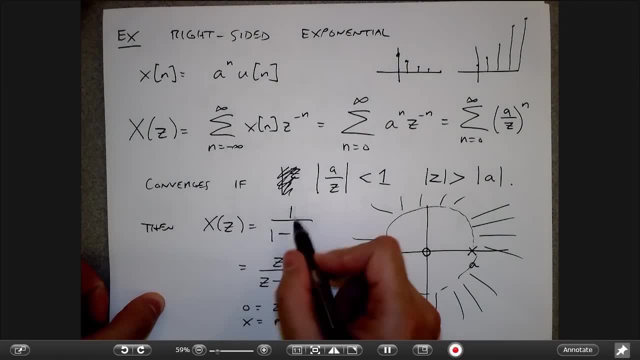 a has to be a real number. right A can be any complex number And my z transpose 1 over 1 minus a over z. that's exactly what I have: 1 over 1 minus the a, which is this over: 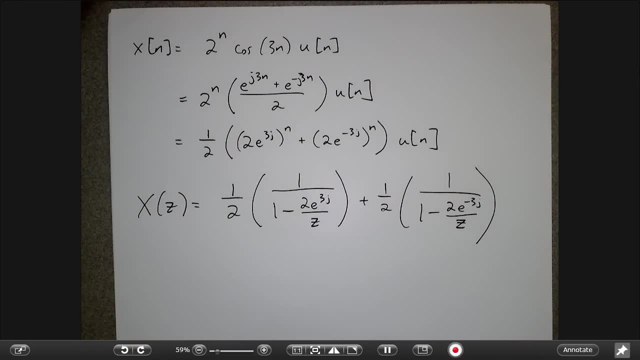 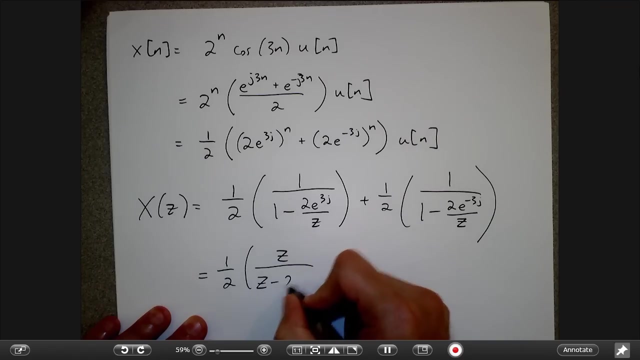 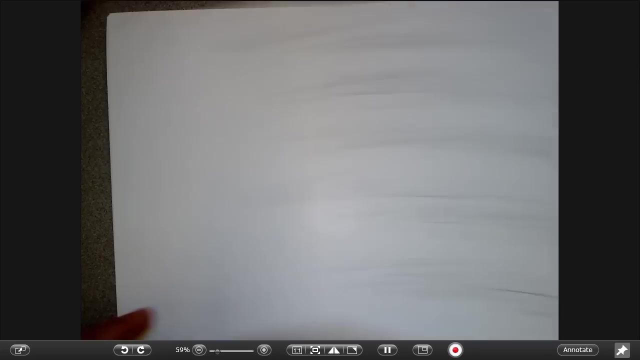 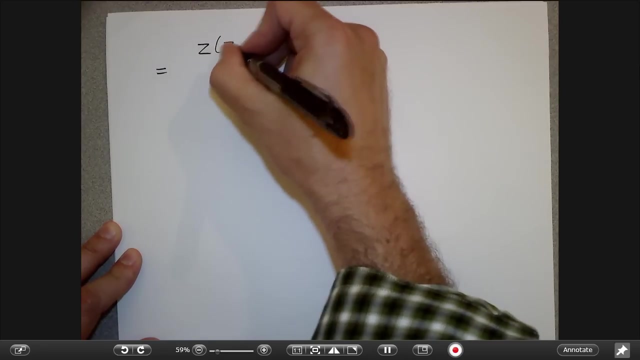 z. And now what is this thing going to turn into? Well, I'm going to have to multiply through by some stuff. So I'm going to multiply each of these guys by a z. And now I'm going to multiply through to get a common denominator. So I'm going to get z z minus 2 to the minus. 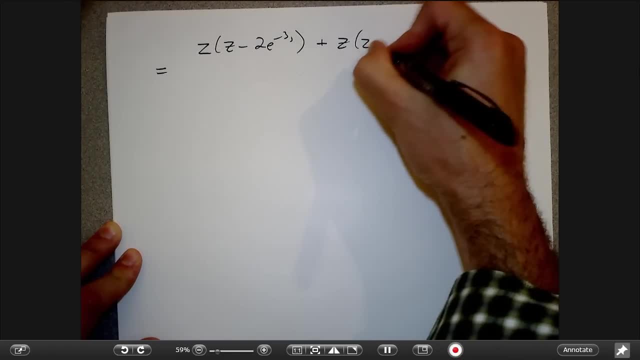 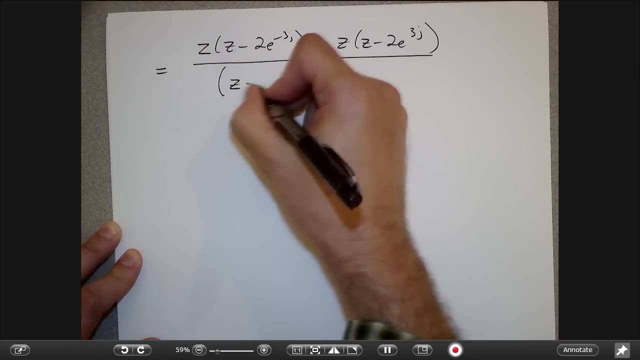 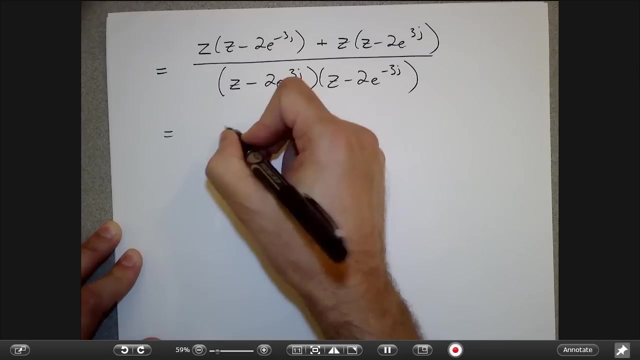 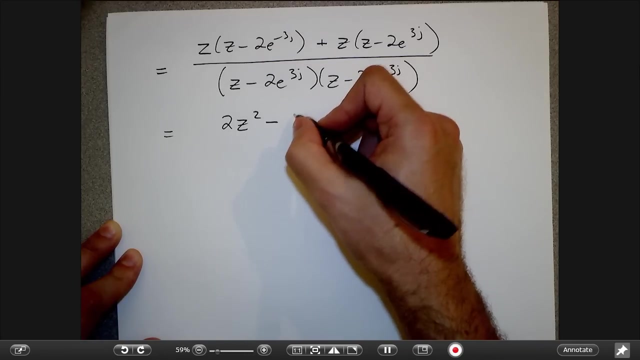 3j plus z, z minus 2e to the plus 3j over the product of these things. So I'm going to get 2z squared minus. well, let's think about this for a second. So what I'm going? 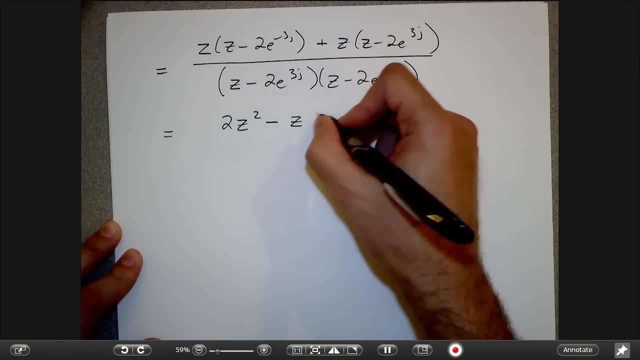 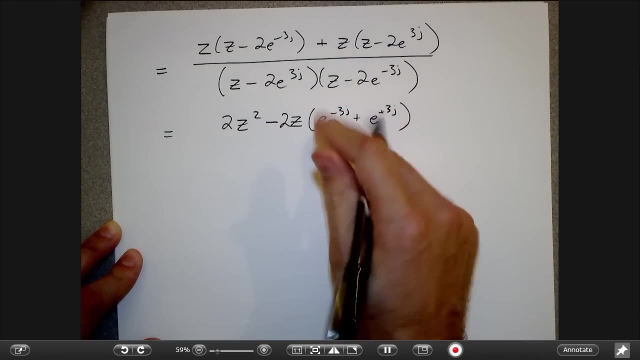 to have is I'm going to have a z Right, Or I guess a 2z times e to the minus 3j plus e to the minus 3j Or, I'm sorry, minus plus right. So again here I'm going to get my cosine coming back at me And the same thing. 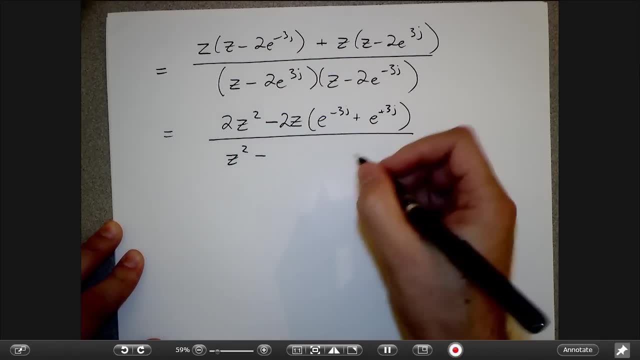 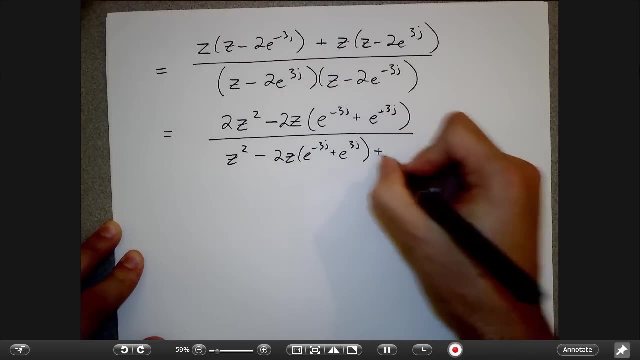 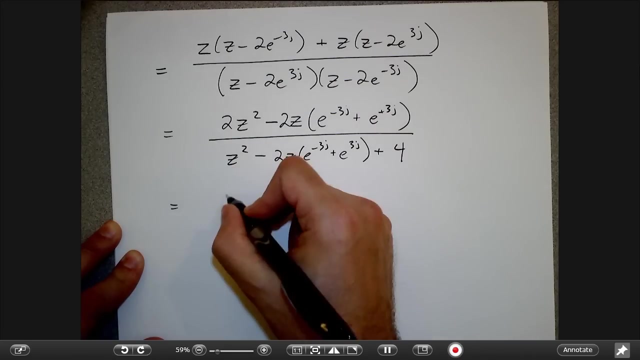 here I'm going to get z squared minus 2z, this thing plus 4.. And then when I multiply these things together, they cancel each other out. So what I'm going to have is I'm going to have a 2z squared minus 2z, plus 2z squared. 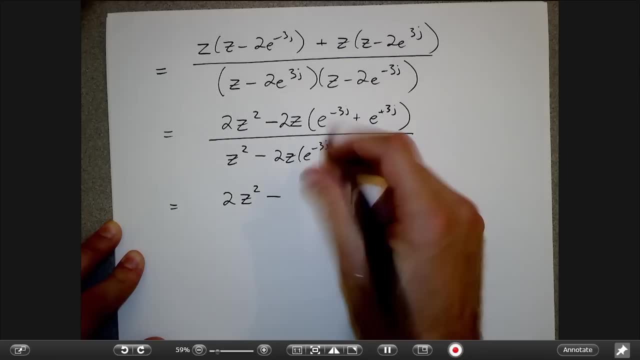 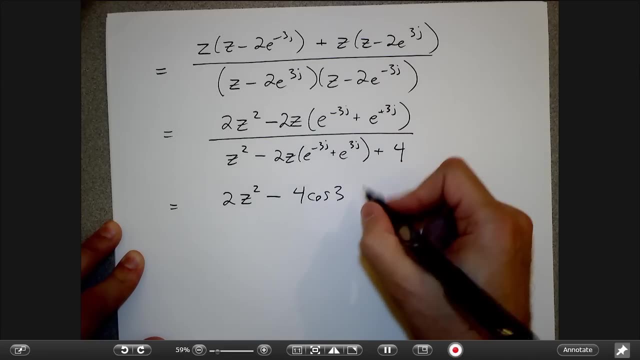 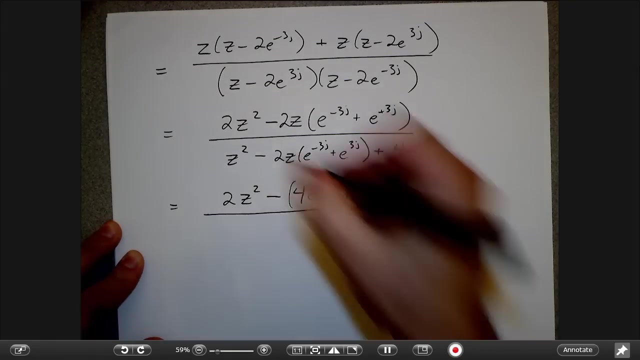 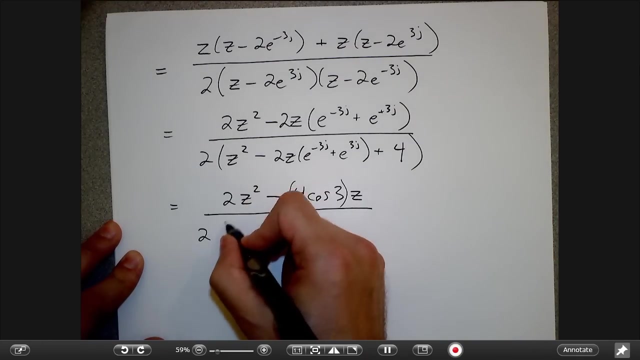 minus. this thing is like two cosine of 3j. so I'm going to get four cosine of 3z over. I think I lost a 2, there was a one half floating around there, so that's 2 times all of this stuff. So then I'm going to get a two times z squared minus 4 cosine. 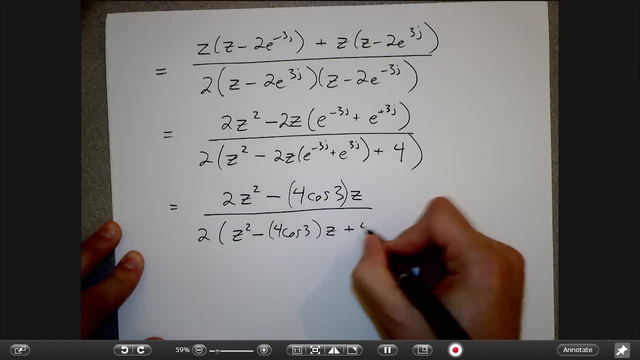 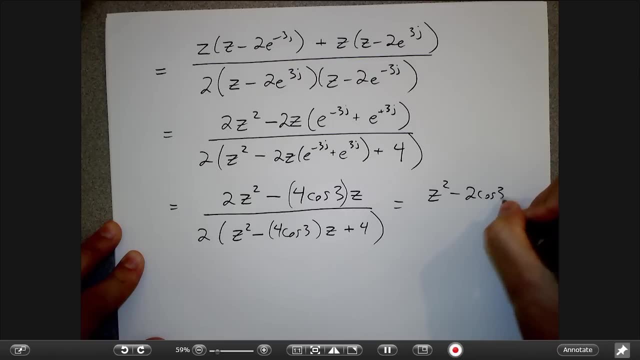 3z plus 4, and so then I'm going to be able to cancel this 2 out to get z squared minus 2, cosine of 3z over z squared minus 4, cosine of 3z plus 4.. Okay, so I kind of came up with the algebraic part of the Z-transform, and now let's think: 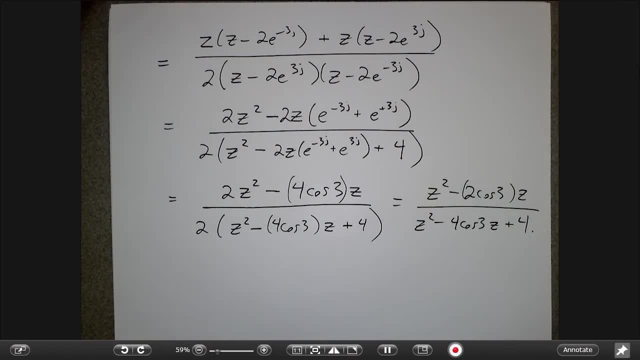 about? what does the ROC of this thing have to be okay? So actually, before I do that, let me just think about this, the poles and the zeros. So what do I have here? Well, I actually kind of can read off from the here before I multiply things out. 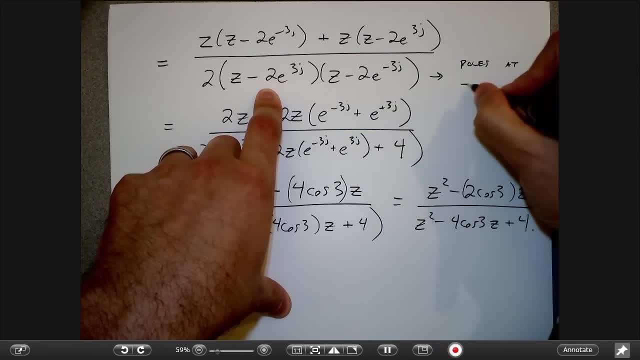 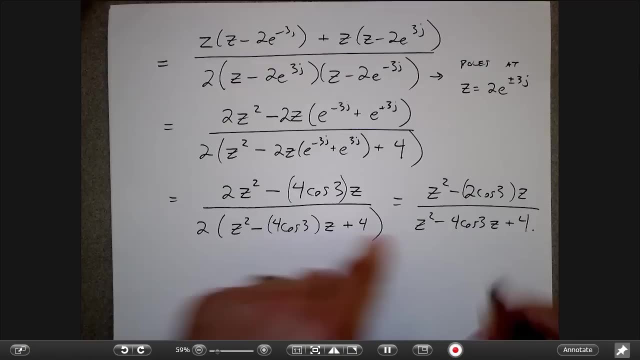 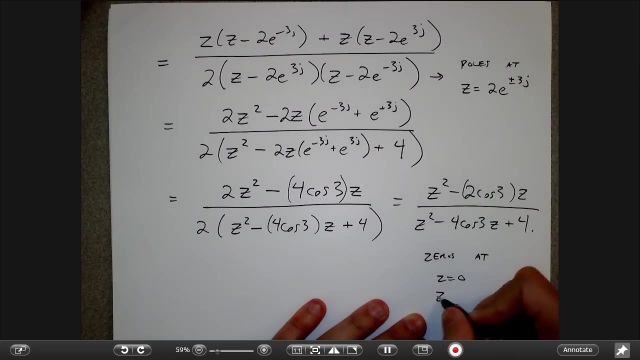 I get the poles at z equals 2e to the plus or minus 3j. and here I can see what the zeros are. I get zeros. Okay. I get the poles at z equals 0 and z equals 2 cosine of 3, okay. 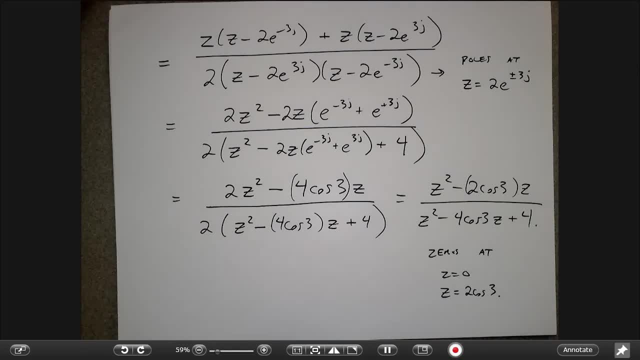 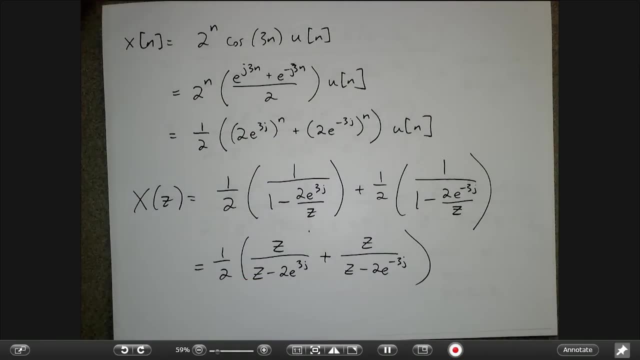 So let's think about what the ROC is for a second. So, again, let's go back to this formula here, right? The only time that I can do this is when the magnitude of each of these terms is less than 1, right? 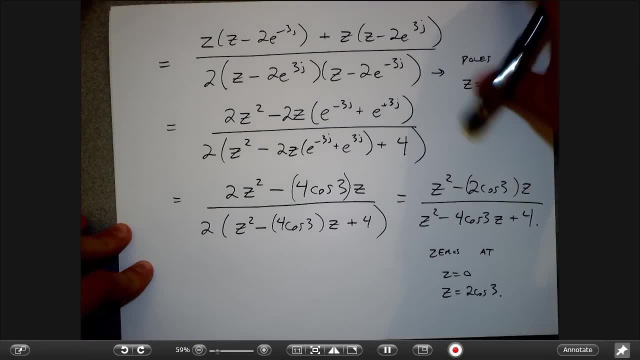 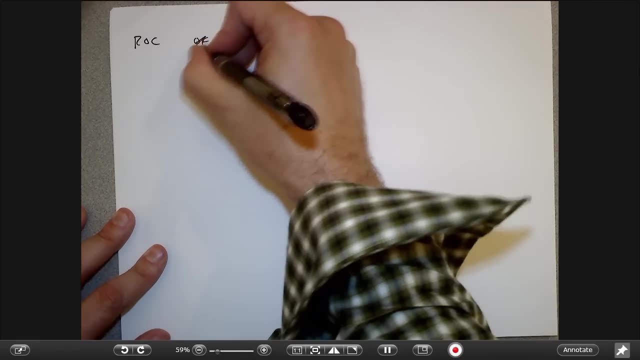 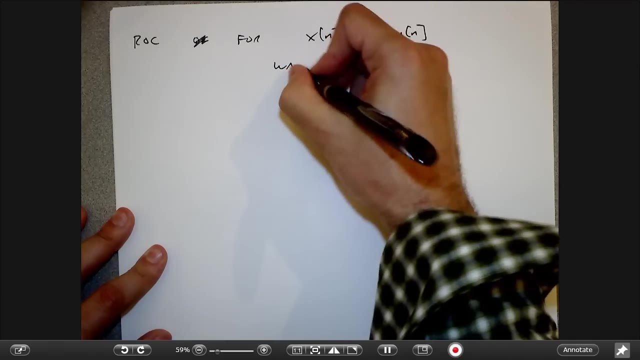 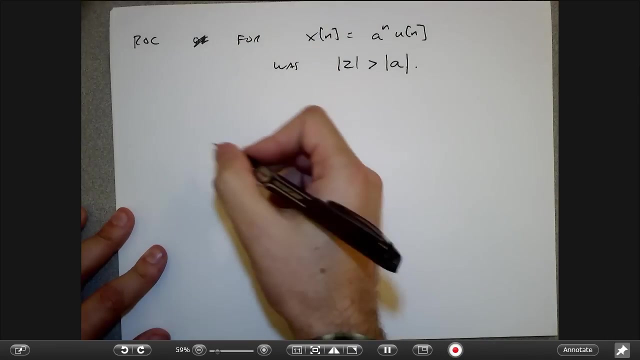 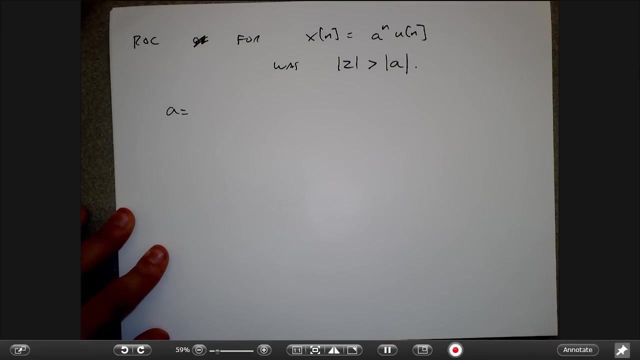 So the ROC Of you know, the ROC for this was magnitude of z, greater than a right. So in this case, a is going to be like what was it? it was like 2e to the plus or minus 3j. 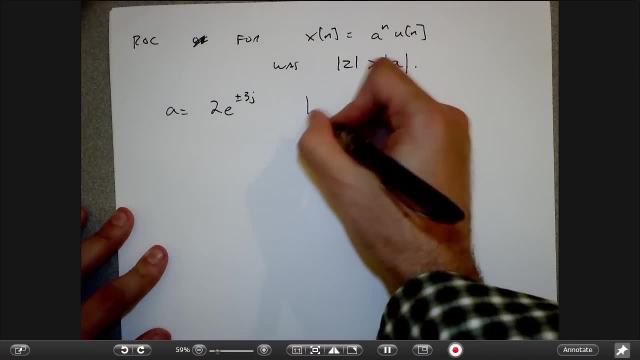 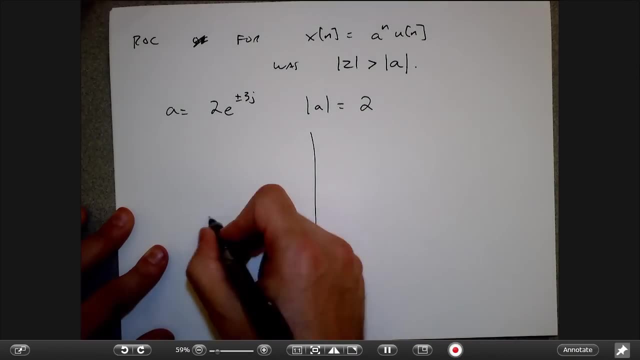 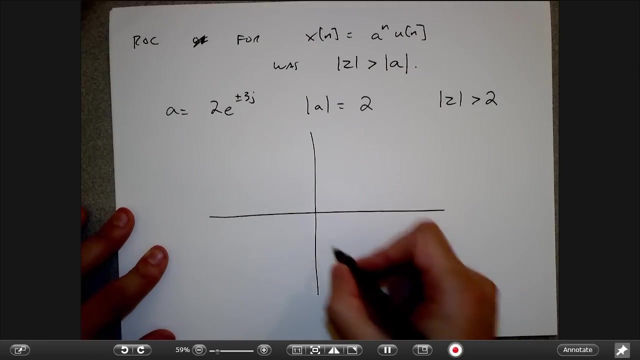 Okay, This is just some complex number that has magnitude 1, right? So the magnitude of this thing is just going to be 2.. And so if I were to draw the final thing, my ROC would be this: I can draw my poles and zeros where I'm going to get a pole. so here's a circle of radius. 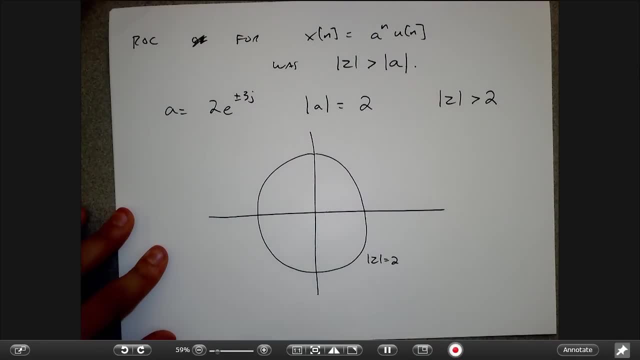 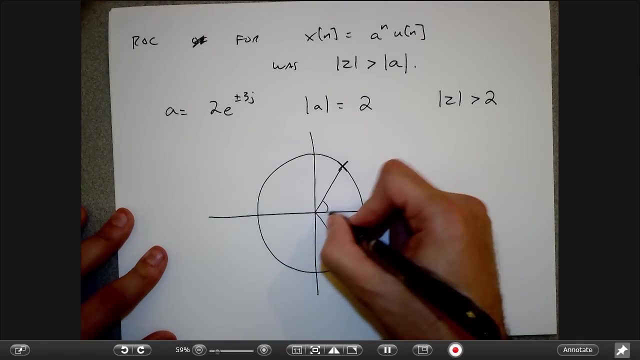 2, right, So this is like a circle of radius 2. I'm going to get poles at z, equals 2. These locations here where this angle is, basically you know, 3. So I get poles at 2e to the plus or minus 3j and I'm going to get zeros at, basically, 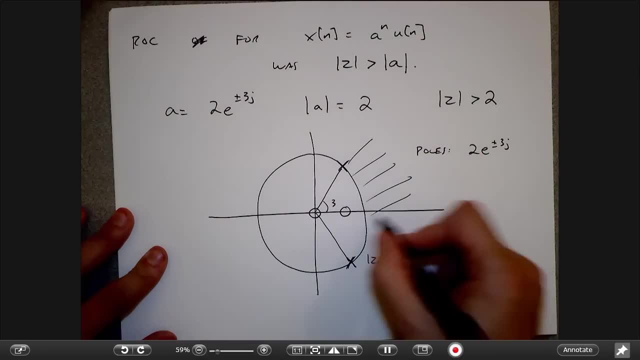 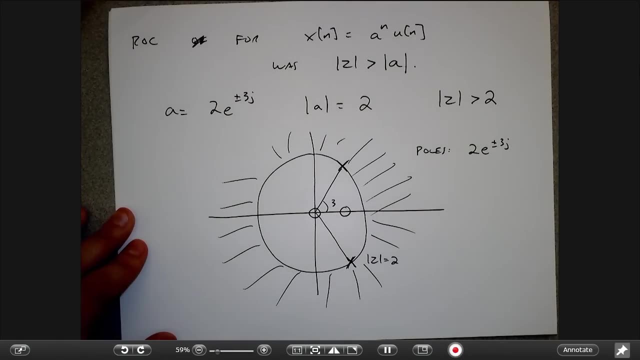 this location and this location and my ROC looks like this: Okay, Okay, Okay. So if I was being more careful, these poles are actually probably over here, because 3 is pretty close to pi, So forgive my poor diagram, But something like this right. 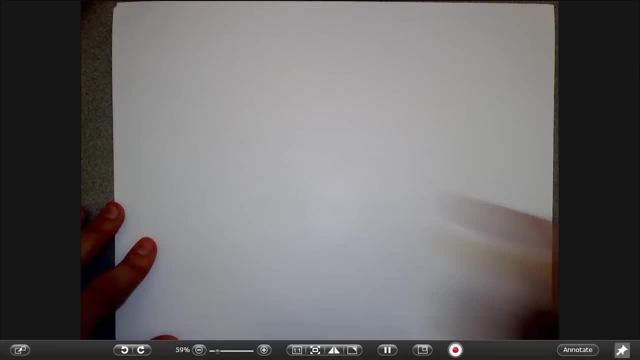 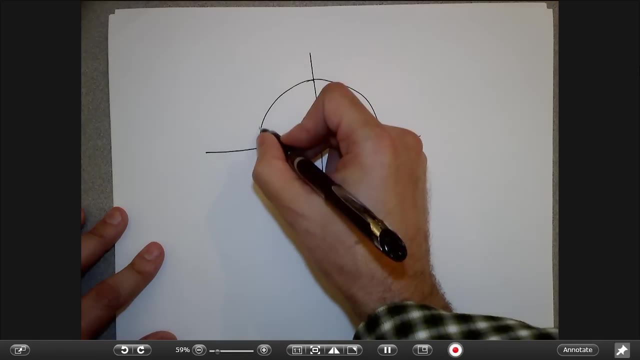 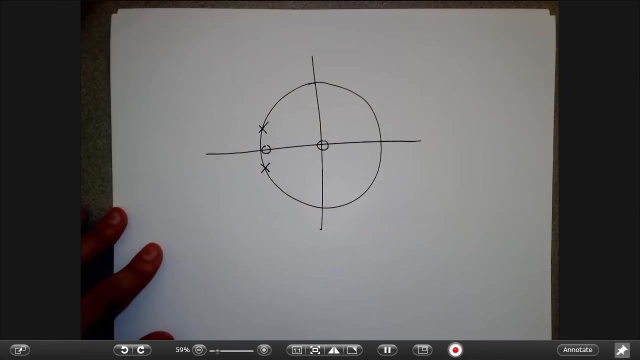 In fact, let me just draw that better. So probably the ROC is more like this. So this is pi right, So my poles are probably over here. right, I have a zero here and I have a zero here, But the ROC is still looking like this. 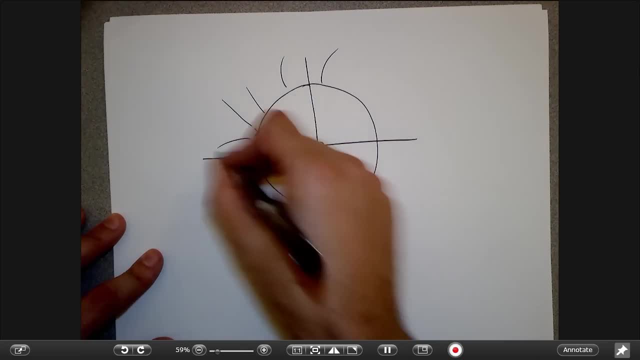 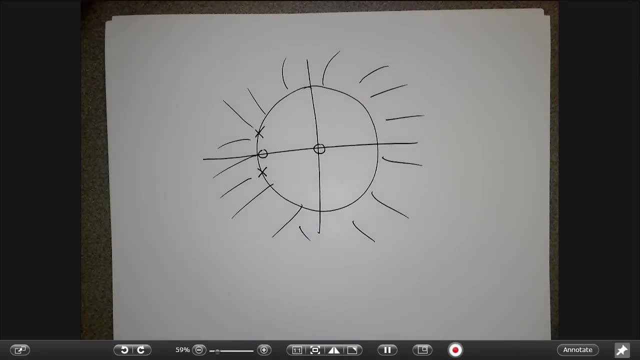 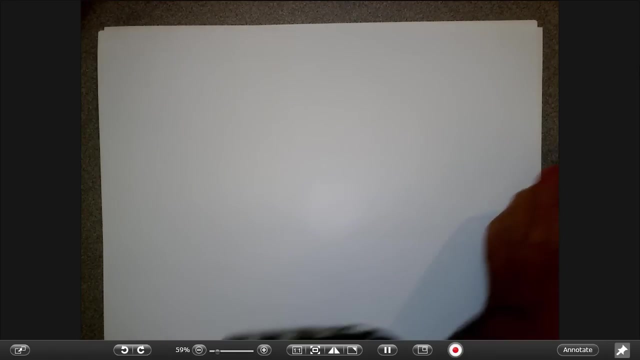 Okay. So at this point, what we should notice, right, is that the ROC always looks like it's somehow related to the poles, And so let me just make some statements about how the ROC and the poles are related. So kind of rules about the ROC. 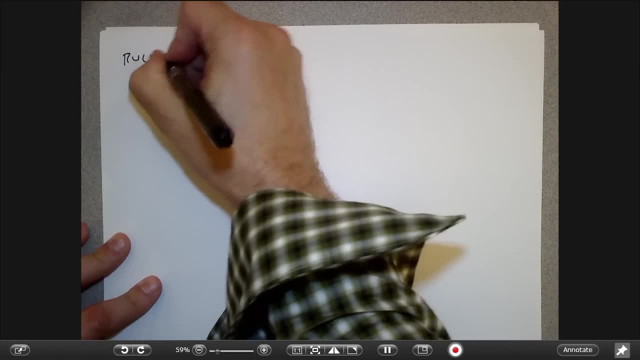 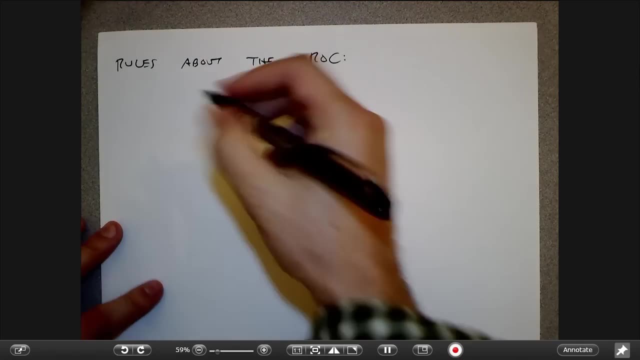 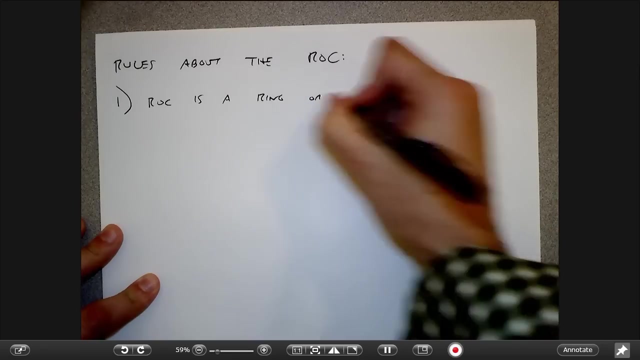 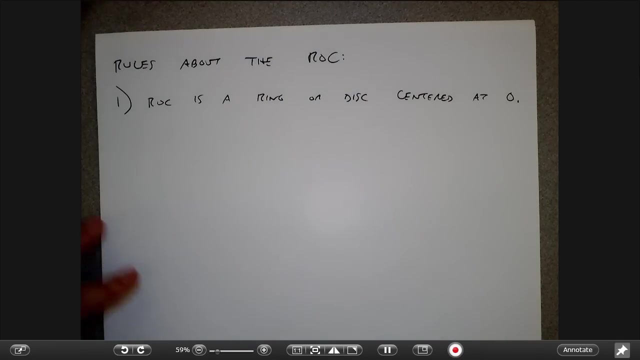 Okay, So the ROC is a ring or disk centered at the origin. We kind of already showed why that was true, because it depends only on the radius of the complex variable, and so that means that it's got to be something that only looks like a. 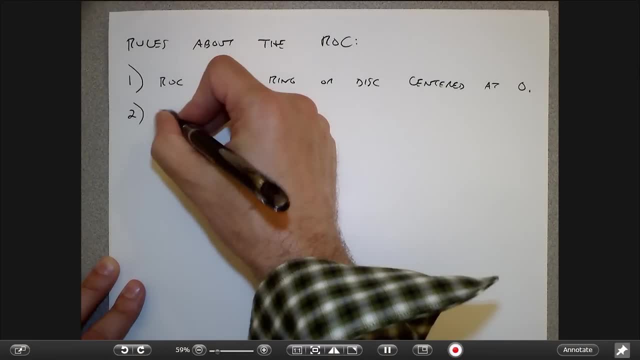 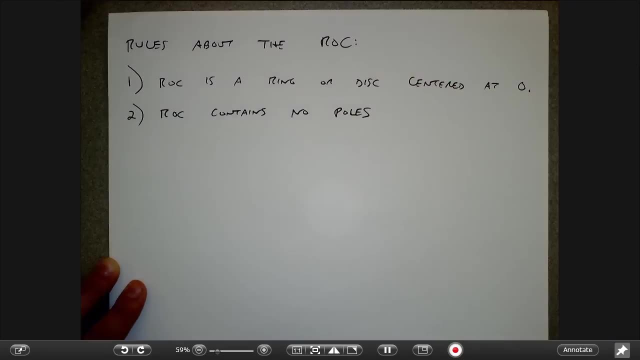 circle or something. Okay, So the ROC contains no poles, right? And that's kind of by definition right, Because if the Z-transform is infinity- right, that's what a pole means- then it certainly doesn't converge there, right? 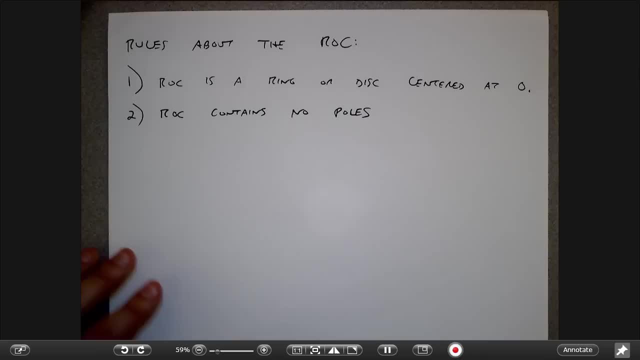 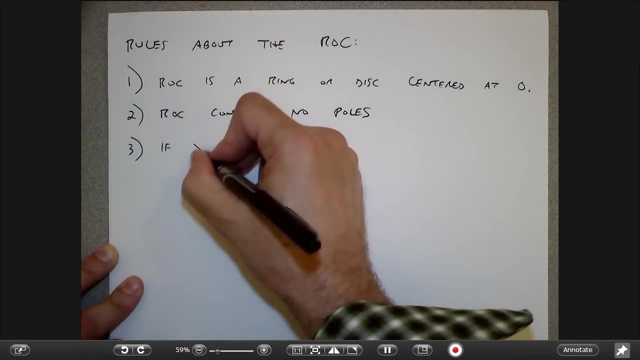 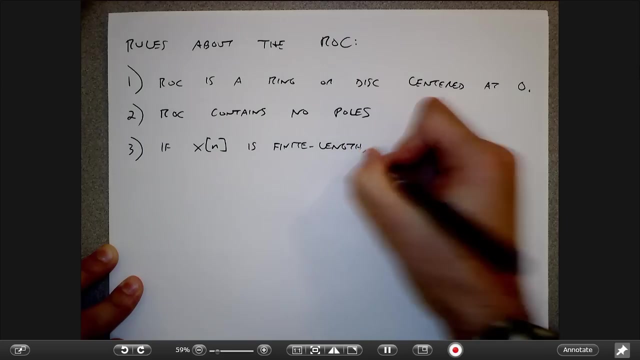 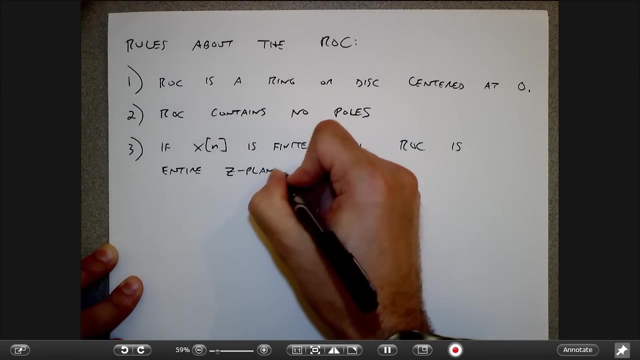 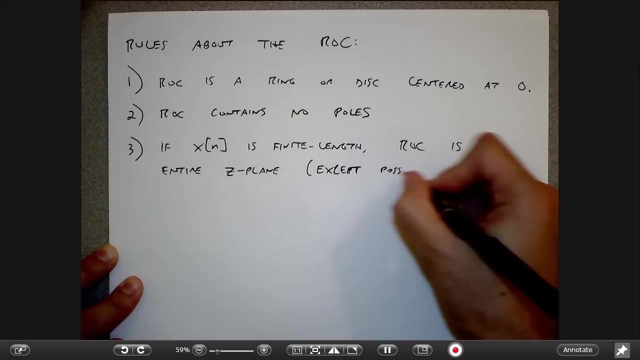 So the Z-transform never contains any poles by definition, Or, I'm sorry, the ROC never contains any poles by definition. Three: we kind of showed earlier is that if x of n is zero, right Okay. If x of n is finite length, the ROC is the entire Z-plane, except possibly you may run. 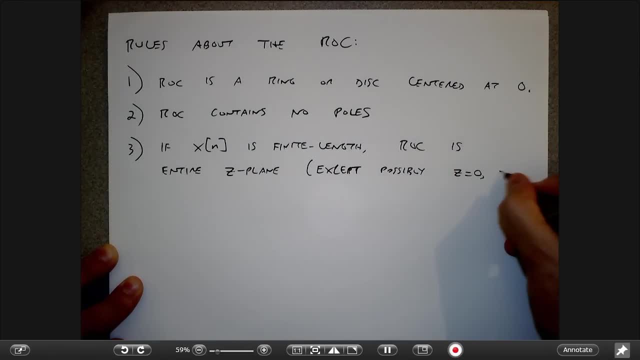 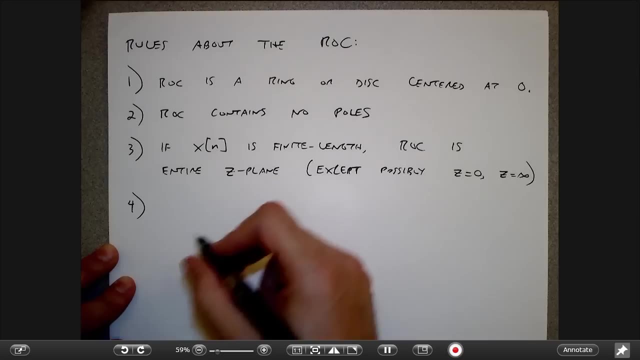 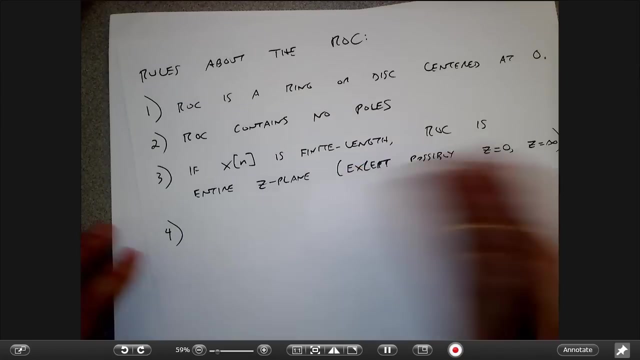 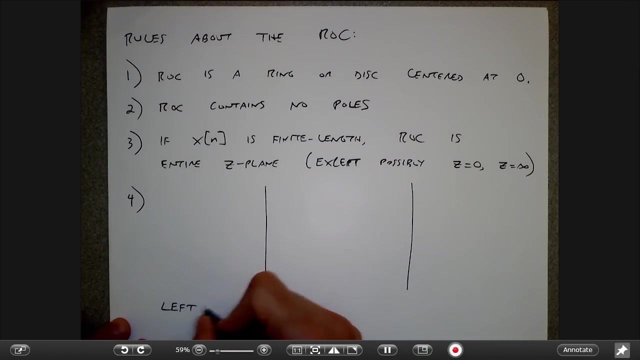 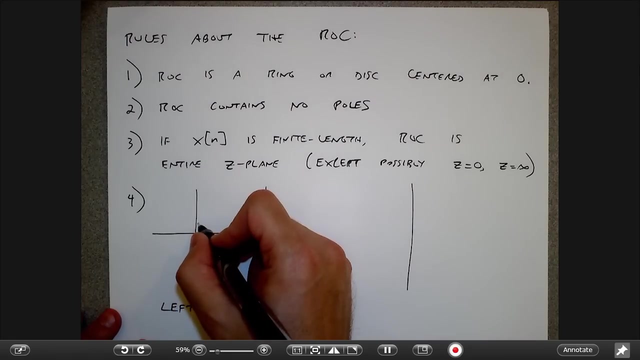 into problems at exactly zero or exactly infinity. Okay, Okay, Okay. So, basically, if kind of, I have a couple of caveats or a couple of cases, right? So if x of n is left-sided, my ROC is basically going to be the region inside the innermost. 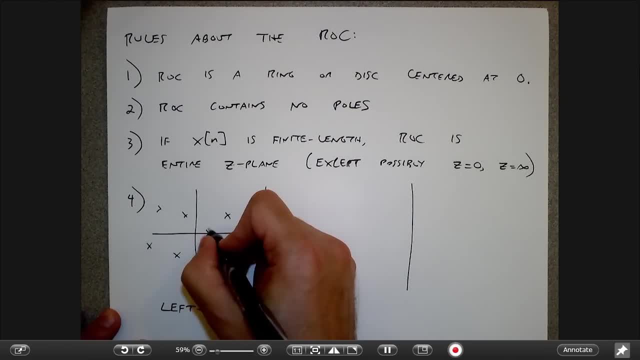 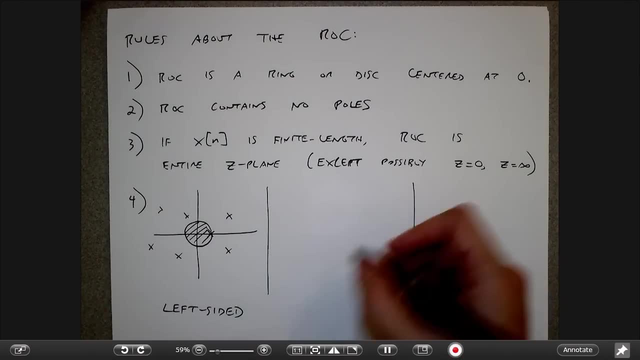 pole. So if I have a bunch of poles out here, the ROC is going to be the inner pole, Okay, Okay. So the ROC is going to be this region like this, The region inside all the poles. If I have a right-sided signal, the ROC is going to be kind of the reverse. 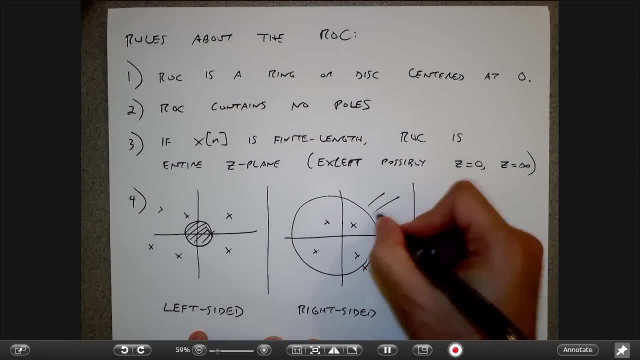 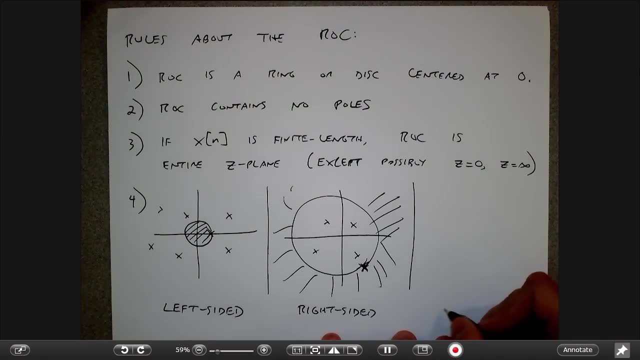 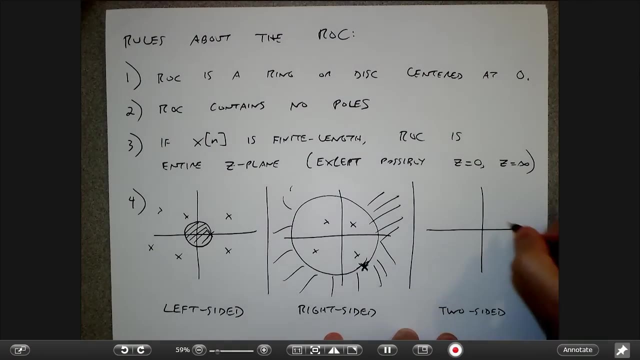 It's going to be the region that is outside the outermost pole And if I have a kind of a two-sided signal, Okay, Okay, then the ROC is generally going to look like some sort of a donut that is defined by the ring between two poles. 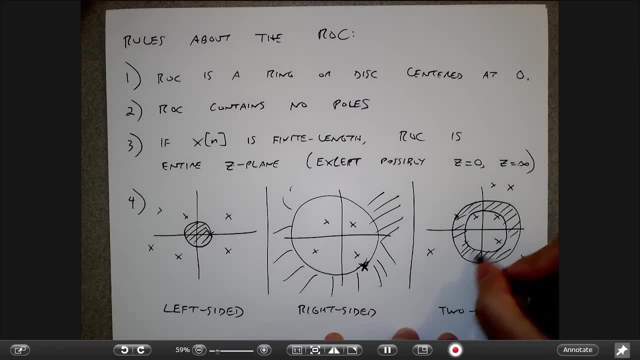 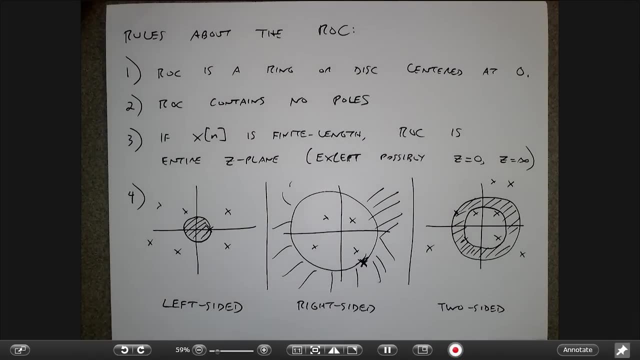 So I could have more poles up here, I could have more poles inside, but in general it's bounded by the poles. So this is kind of a way of saying the ROC is always bounded by the poles and that in special cases I kind of know that a left-sided signal looks like this: 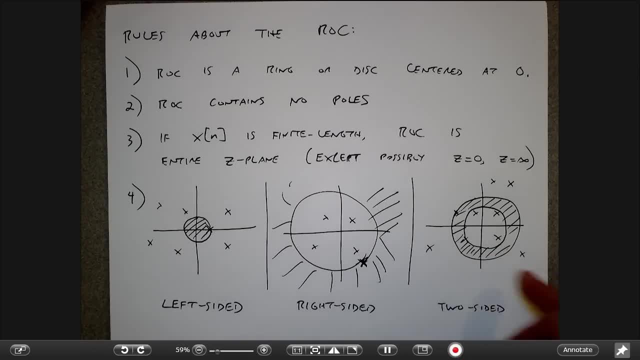 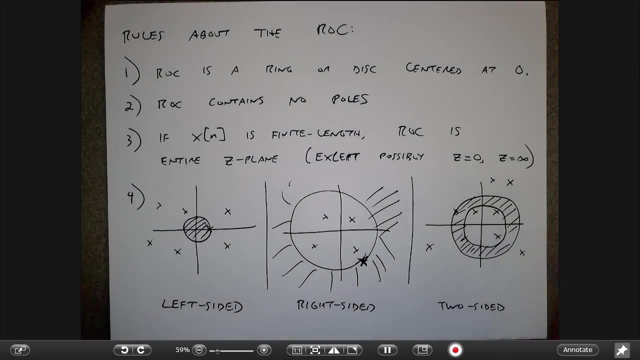 a right-sided signal looks like that In this case. there are many possible donut-shaped ROCs that correspond to different two-sided signals, and I'd have to kind of disambiguate within there which one I meant. Okay, So one thing that I can't have is I can't have a pole in the ROC. 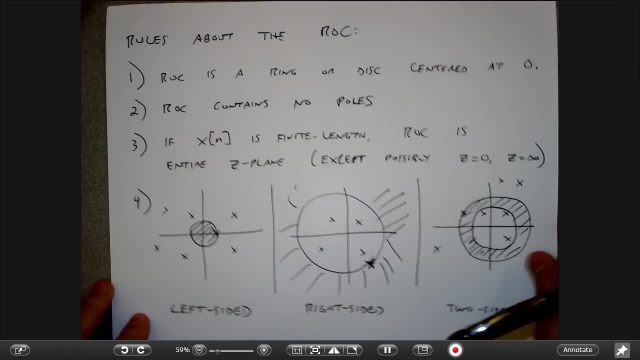 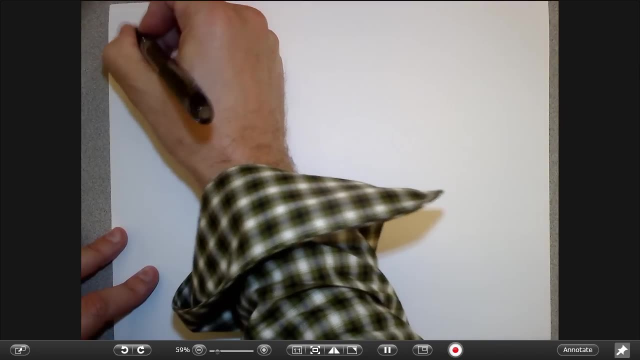 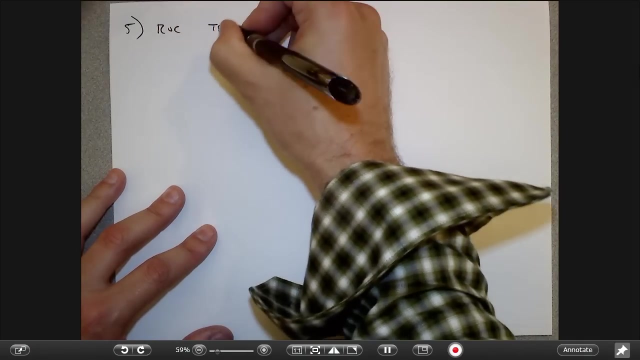 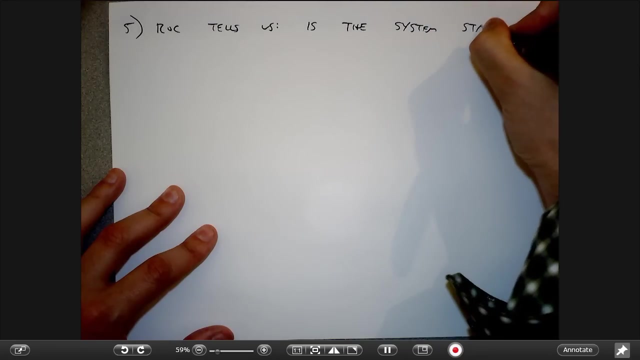 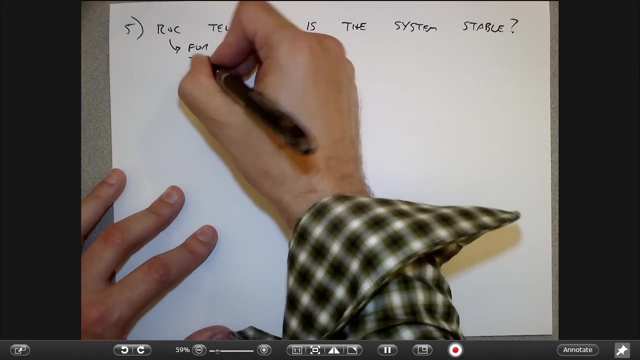 That's rule number two, And I guess the final thing I want to say is that. so the ROC kind of tells us: is the system stable? So ROC meaning for a, the transfer function H of Z. So when I apply this to a linear system, 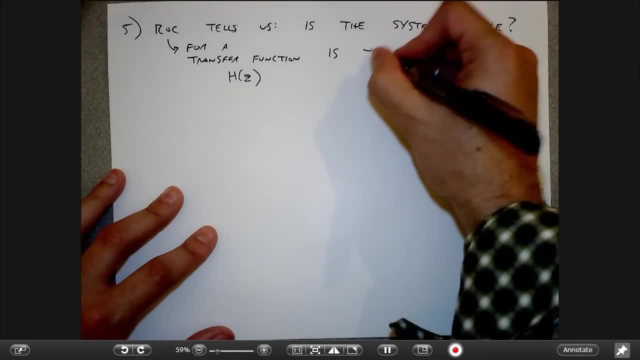 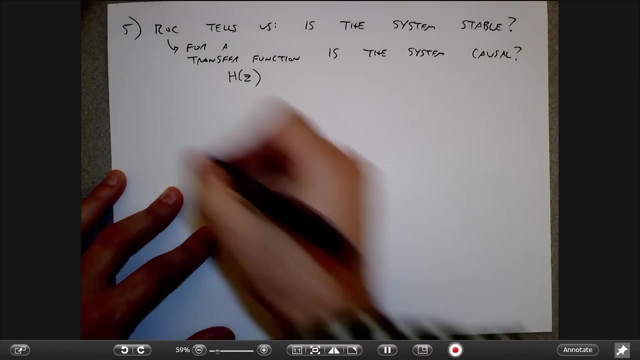 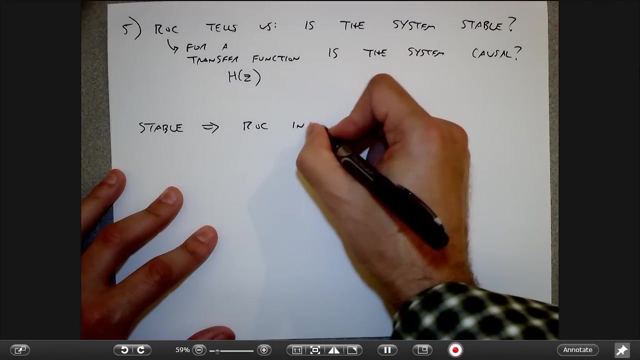 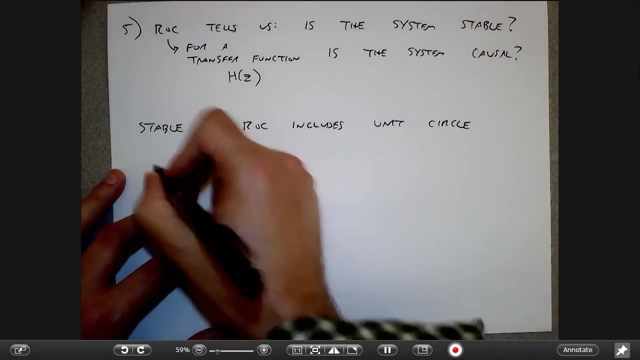 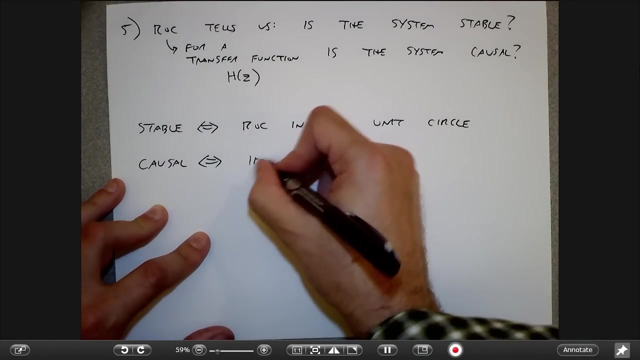 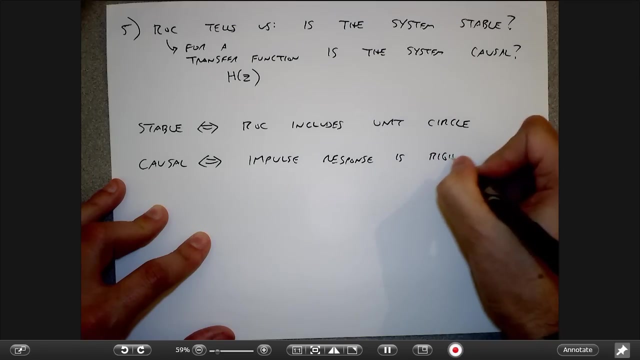 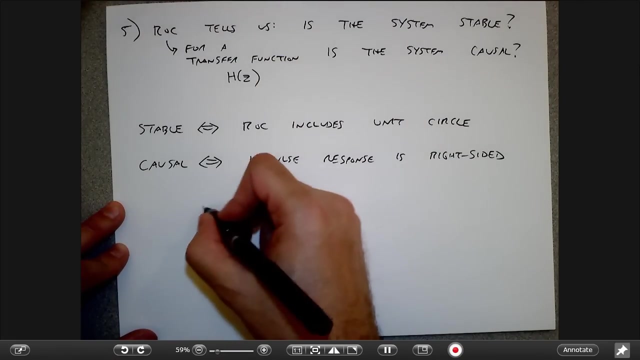 I can say: is the system stable And is the system causal? So, stable implies that the ROC includes the unit circle, And causal implies that you know, the impulse response is right-sided And so that means that I can have some cases where I can say: okay, you know. 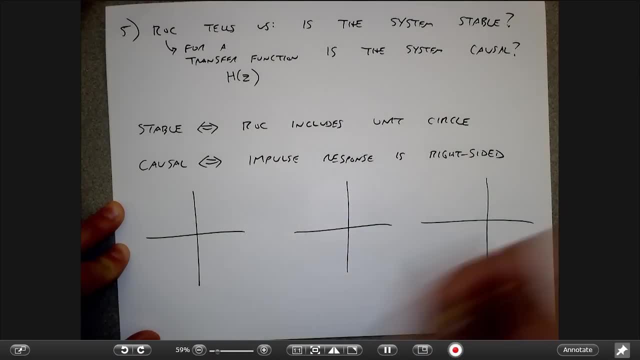 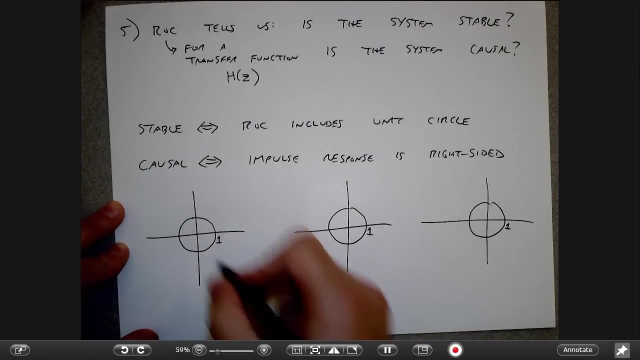 I can just kind of look at some possible ROCs and say here's the unit circle In each case. All right, so these guys are the unit circle, And let's suppose I have poles at, you know, one half and minus two. 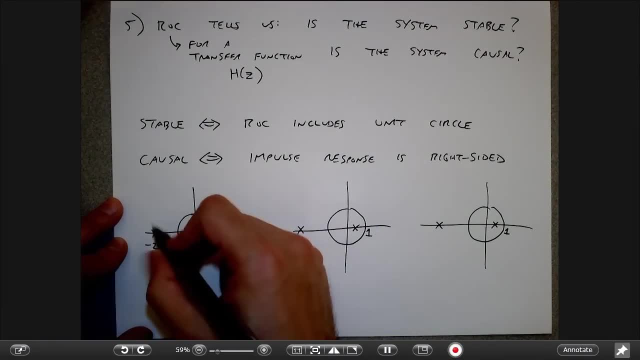 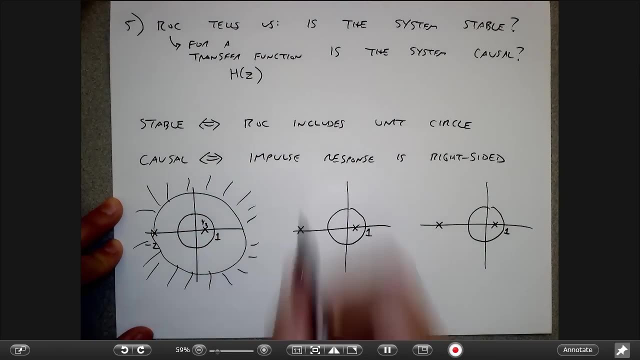 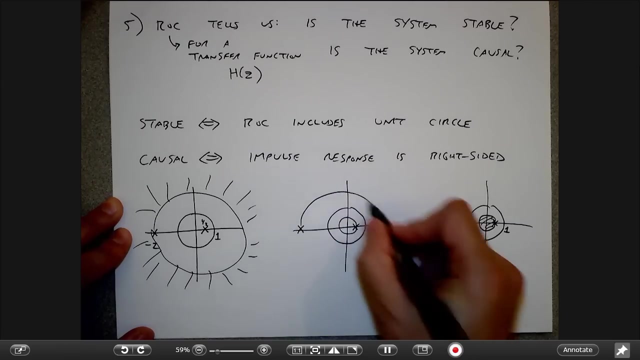 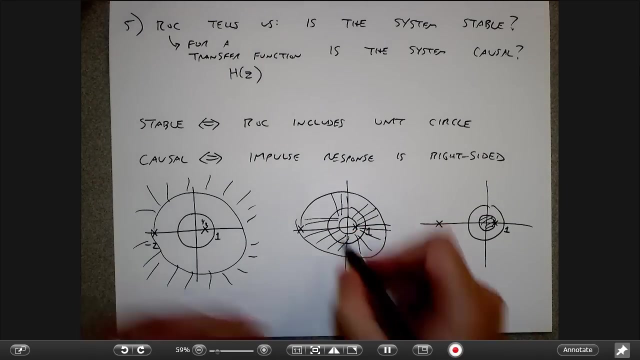 So there are three different kinds of ROCs I could have here, right. One is this guy, One is this guy And one is kind of this guy, right. So this one here. sorry for my crappy drawing. So this one here includes the unit circle. 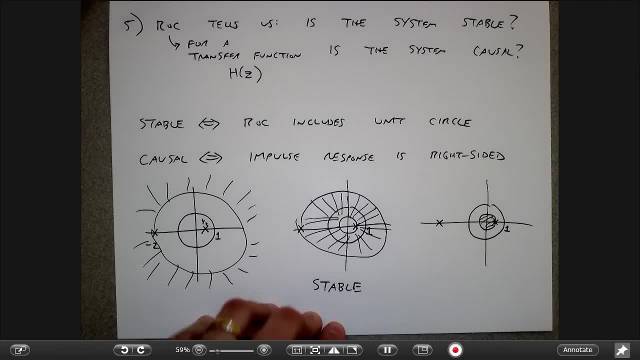 So this is a stable system. But because the ROC doesn't go out to infinity, this is not causal, Right? Okay, Okay, I get it. So this is not causal causal. Here this guy looks like a right-sided signal. so this is causal. but since it doesn't, 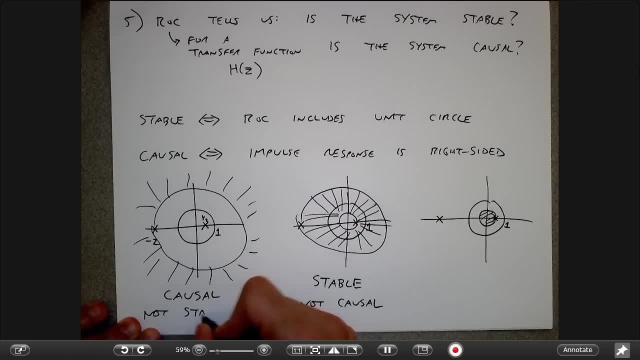 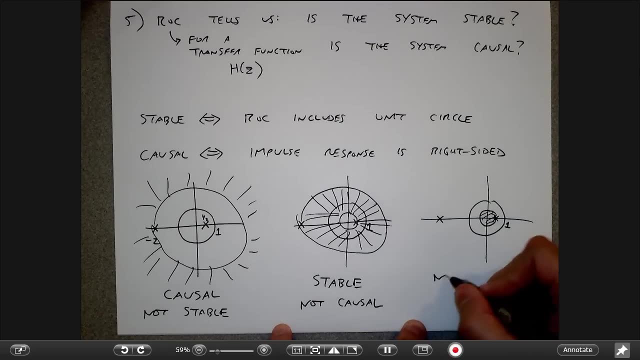 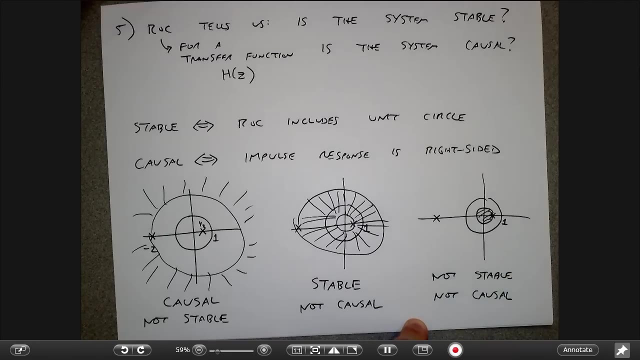 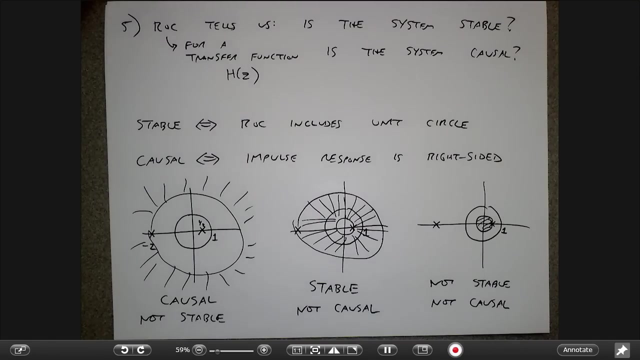 include the unit circle. it's not stable, And this guy neither includes the unit circle nor goes out to infinity, so this is not stable and it's also not causal, And so the thing that we desire the most is a system where all the poles are inside the 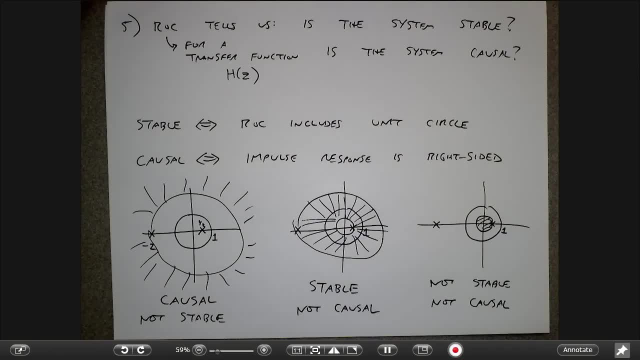 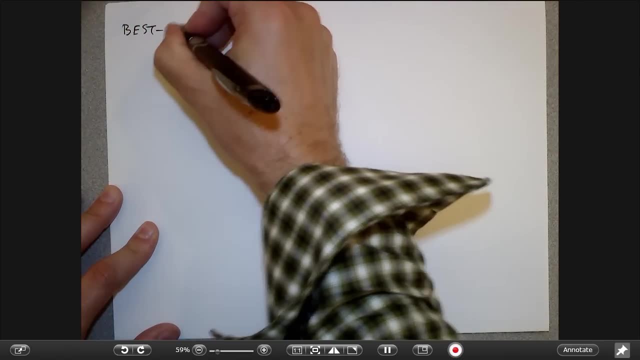 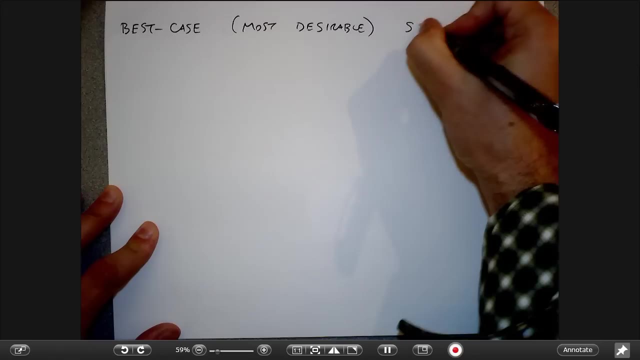 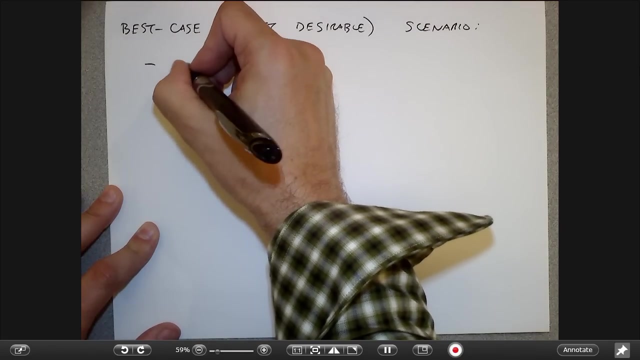 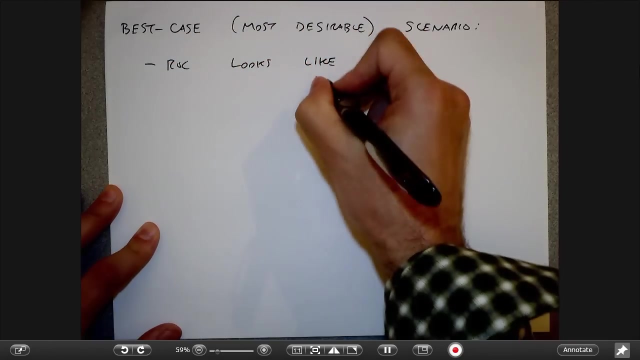 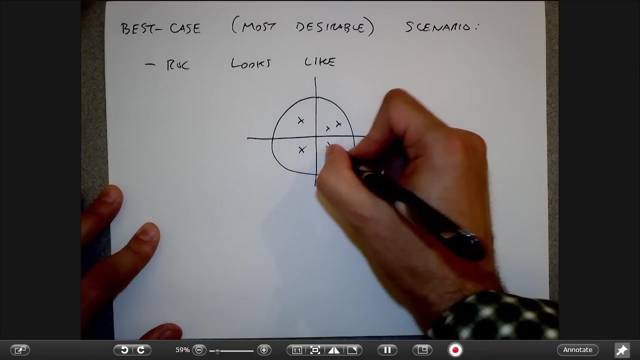 unit circle and the ROC looks like a starburst going outside that pole, the outermost pole. So the best-case scenario- maybe this is a little bit slangy- let's say most desirable scenario Number one is that ROC looks like: here's the unit circle, all the poles are inside the unit circle and 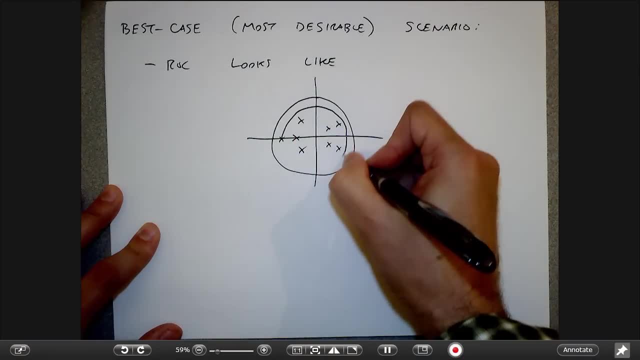 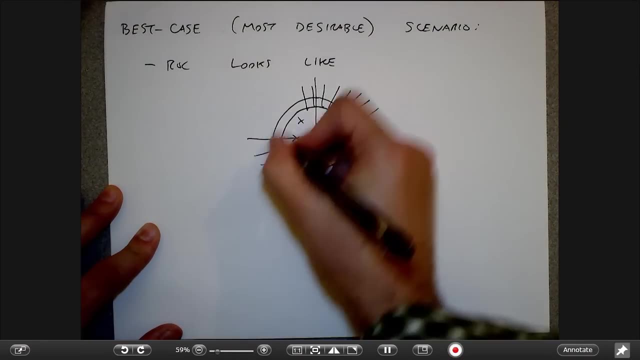 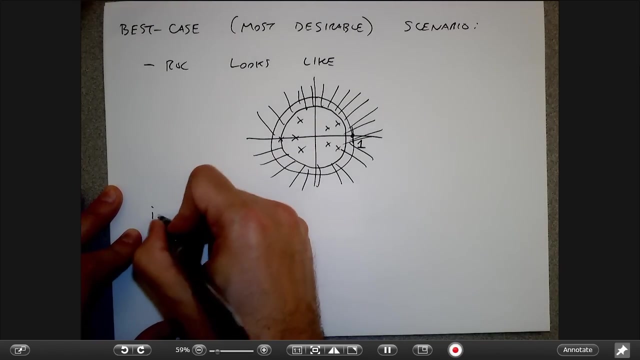 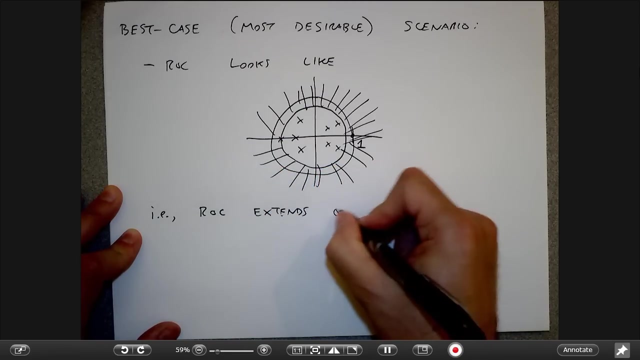 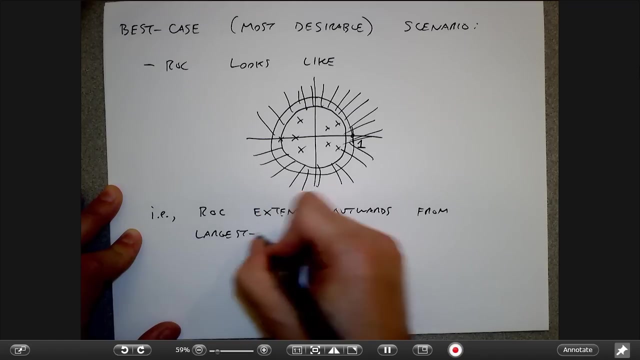 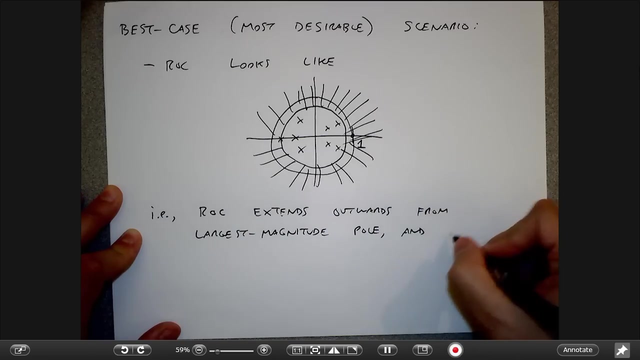 the ROC looks like a ring that is, or it looks like a sunburst that's extending outside the outermost pole, Right. so the idea is that this is the unit circle. So ie ROC extends outwards from the largest magnitude pole and all poles. 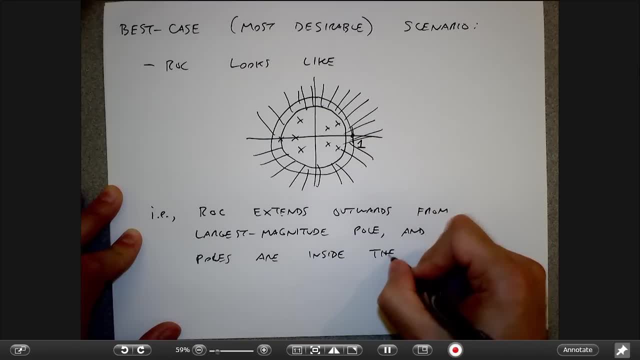 are inside the unit circle Right. so when we design systems, especially things like control systems- this is what we want- is we want to kind of make sure that all the poles are inside the unit circle and that the ROC extends beyond the outermost pole right. 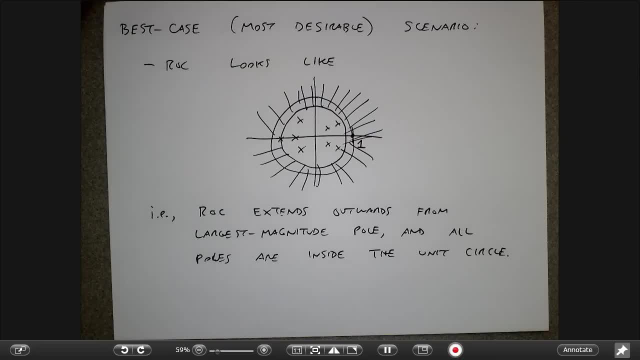 And this is exactly analogous to stuff that you must have done in signals, where we wanted, for example, to push all the poles into the left half-plane- right, That meant good things for continuous time systems, Right. And just in the same way that there were tests to show whether or not, for a given Laplace, 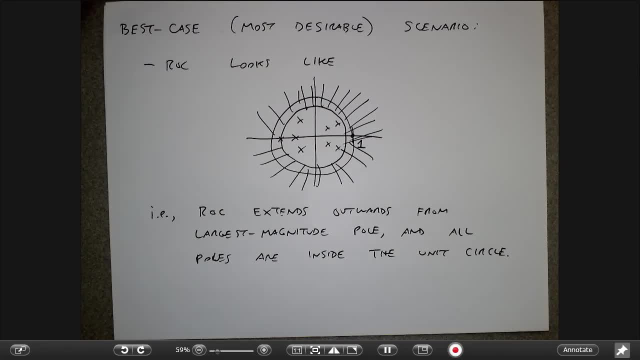 transform. version of the transfer function. the poles were in the right place. there are similar things for discrete time, right? So all those things like the Ruth Hurwitz test and root locus and stuff like that, you can do that for discrete time too. 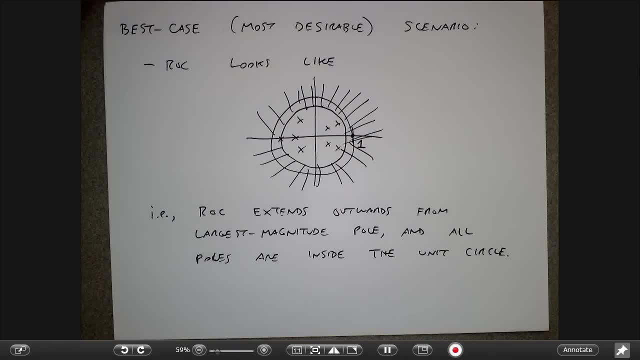 I don't think I'm going to get to things like root locus for this, but the same idea is applying, So and that stuff is actually kind of fun, like drawing the little diagrams for when things go past the unit circle- But I don't think we're going to do it in this class. 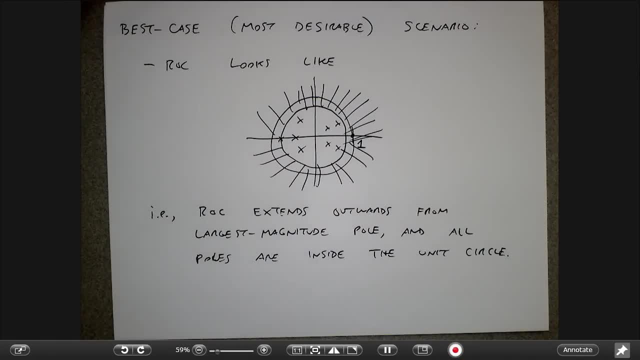 Okay, So all I talked about this time was basically the forward definition of the Z-transform. So what I'm going to talk about next time is kind of how do we deal with inverse Z-transforms and what are some Z-transform properties that make our life easier? 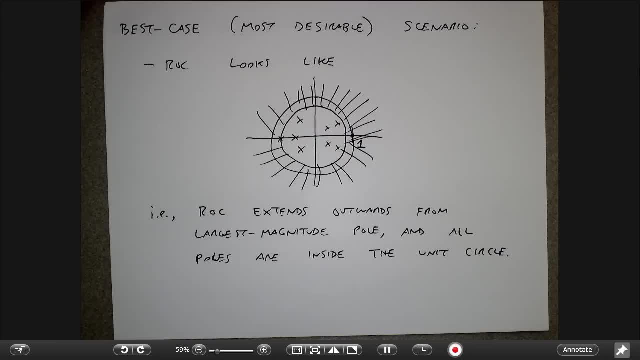 So any questions or comments? Okay, In that case, we are done for the day. 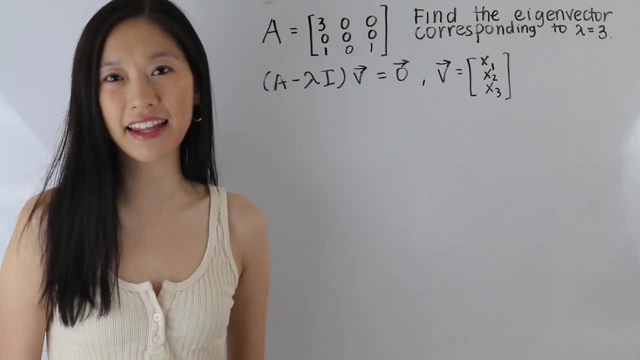 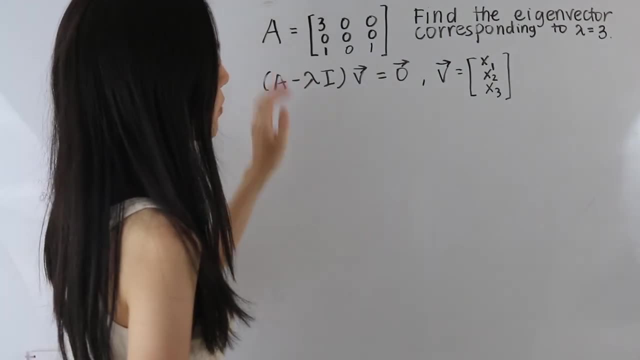 Hey guys, it's Janine here, and in today's video we are going to be learning how to find the eigenvector of an eigenvalue in a 3x3 matrix. So in this problem here, we're given this matrix A and we are asked to find the eigenvector corresponding to the eigenvalue. 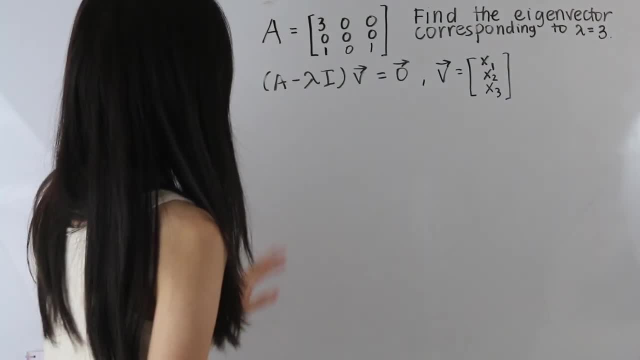 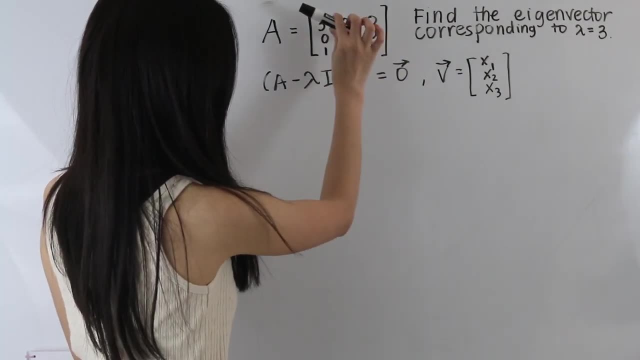 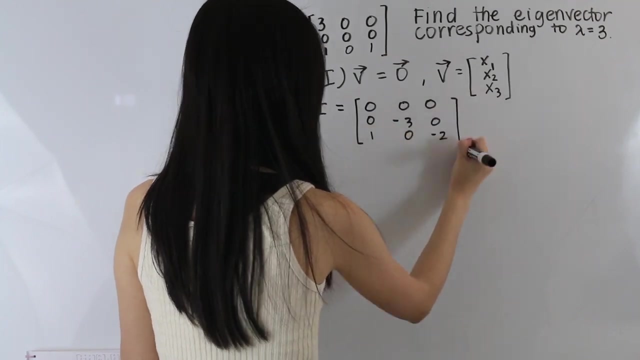 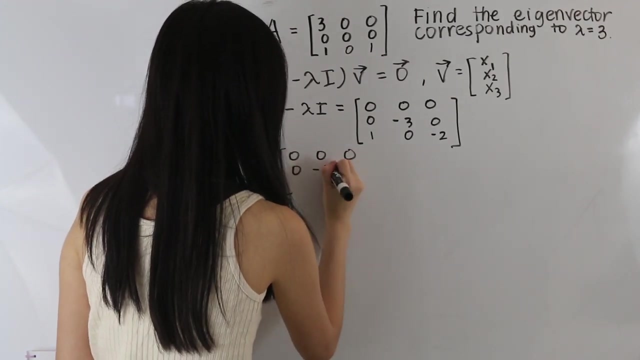 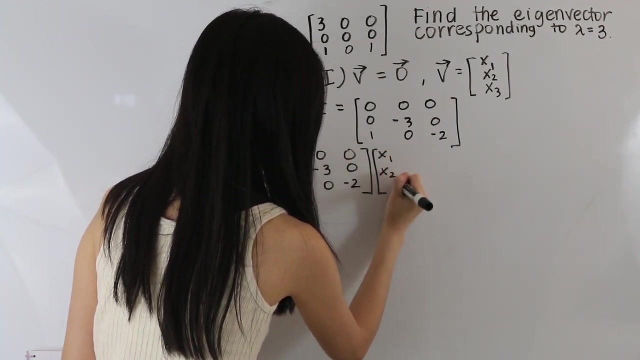 lambda is equal to 3.. So let's start off by determining what A minus lambda i is equal to. And remember all this means is that we're subtracting the diagonal elements of this matrix by lambda. So let's do that. So the next step is we're going to plug this in to here, And v is just the eigenvector. 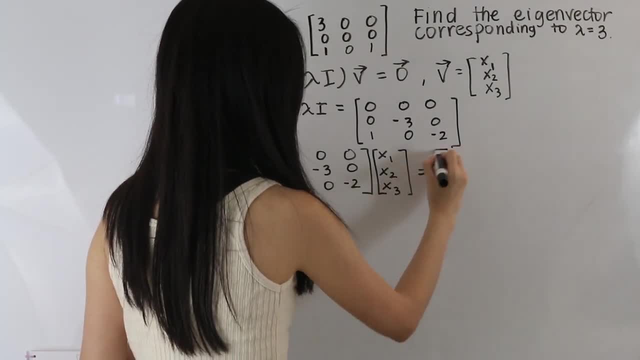